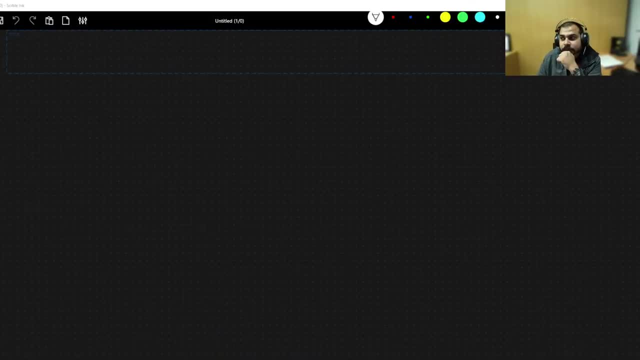 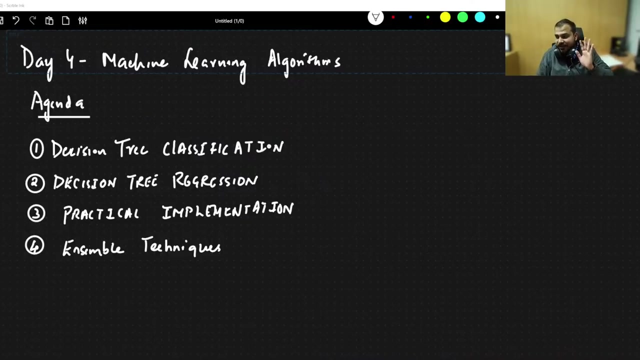 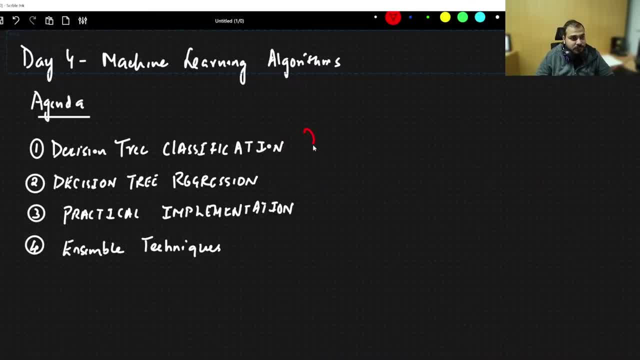 Okay, perfect. So this is the agenda of this session. We will try to complete this, all things Again. here we are going to understand the mathematical equations and all. Okay, Yeah, Okay, perfect, Okay. so my voice is basically very much clear. 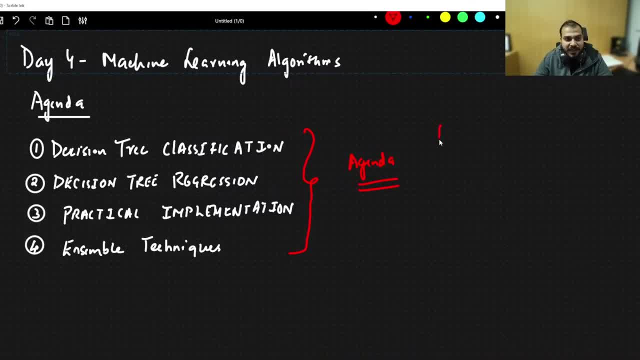 So how was the experience with respect to day 1,, day 2,, day 3? Day 3, all the sessions were good, Right? Okay, All the sessions. how was the experience Good enough, Right? So I hope it was amazing for you all. 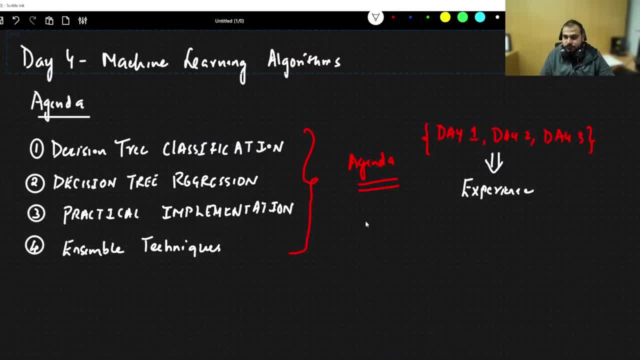 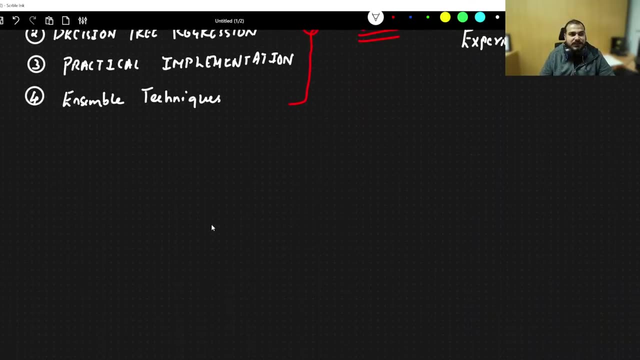 You may have probably learnt a lot. Yeah, Great, Perfect. So the next sessions that probably we will also again have 7 days live session, other 7 days live session. We will try to put EDA or some time. 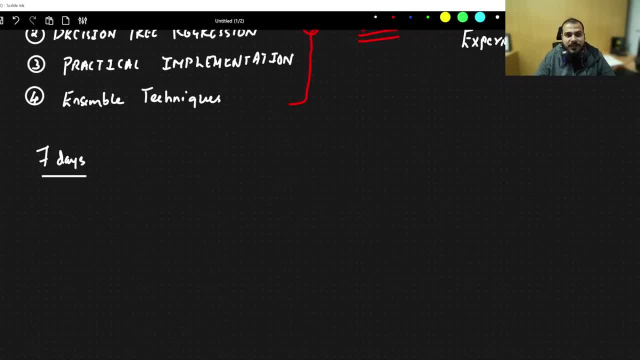 We will try to also cover up deep learning, But, again, based on time constraint, let's see how much we will be able to cover in 7 days. Okay, So in today's session, before we start, please hit like: 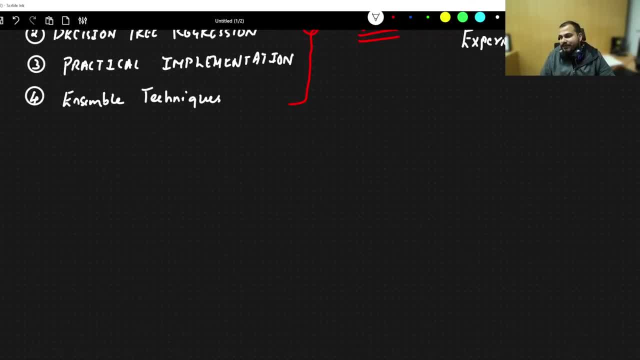 Okay, I see less number of people have joined today, but that's okay. Whoever are interested, they can definitely join. Okay, So here we are basically going to discuss about something called as decision tree, And this decision tree is amazing algorithm, okay. 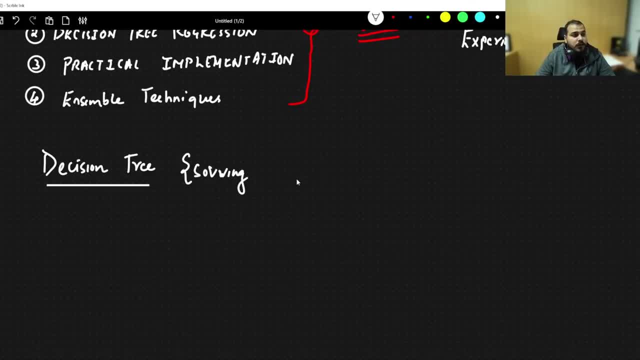 For solving many use cases. solving many use cases Why? I'll tell you: because in the later stages, when we'll be learning about, when we'll probably be learning about the ensemble techniques, it will definitely like you will be able to learn it a lot. 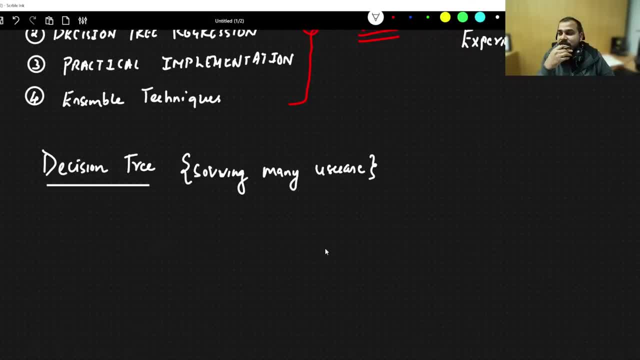 Okay, I mean the main accuracy. you know which is basically. you know which is basically there. Don't worry about the practical part, guys. right now for KNN NAVBIAS. I know Later on, when I get time, I will directly create those things and probably upload a. 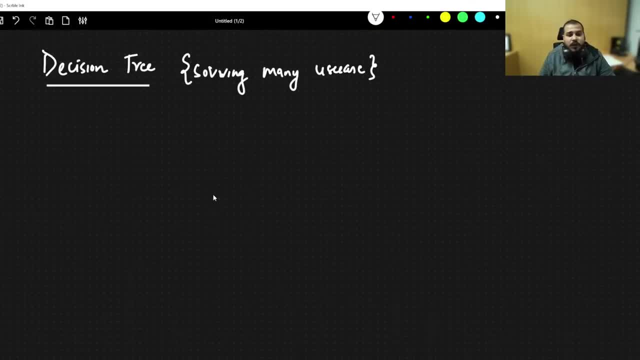 video or take a live session, Okay, So what? let's focus on the sessions now, Okay, Okay, So hit like and let's start Again, Again. some spammers. Spammers are everywhere. Everywhere, spammers are there. 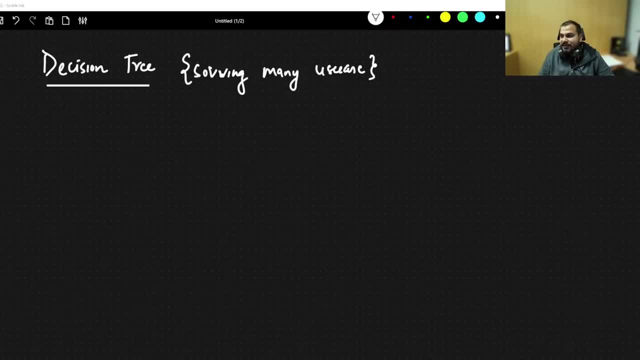 Can't help. Okay, fine, not a problem. Okay, So let's start. So today's session we are basically going to discuss about decision tree, Okay, And in this session we are going to basically understand what is the exact purpose of decision. 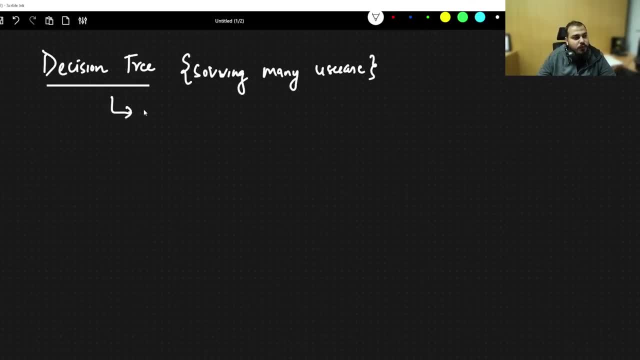 tree. With the help of decision tree, you are actually solving two different problems. One is regression And the other one is classification. So we'll try to understand both. this particular part, Okay, And we'll try to understand by taking a lot of examples where we will be solving a lot. 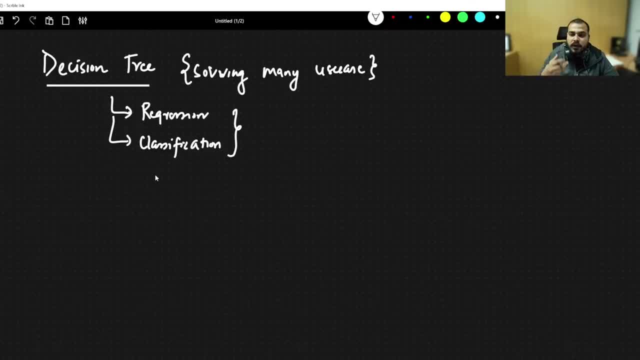 of. well, we will take a specific data set and try to solve those problems. Okay, Now coming to the decision tree, one thing you need to understand. Let's say that I'm writing a if else condition. I'll say that if. 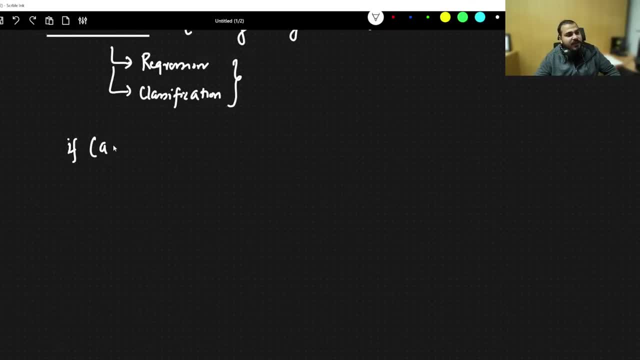 Age is less than 8.. Let's say I am writing this condition If age is less than or equal to 18, I am going to say: print go to college. Let's say that here I am printing, print college. And then I will write else if age is greater than 18. and or let me write it down like this: 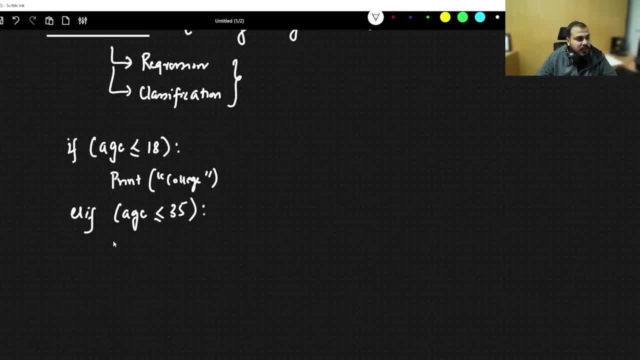 Page is less than or equal to 35 and say print work, Then again I will write else. if age is, let me put this condition little bit better So that you will be able to understand why I am specifically writing this: age conditions and all. 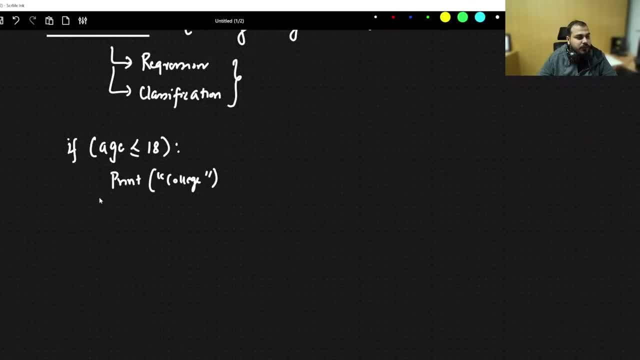 You will be able to understand just a second. Then I will write here: elif, age is greater than 18. And age is less than or equal to 35. I am going to say print work. Basically, people needs to work in this age. 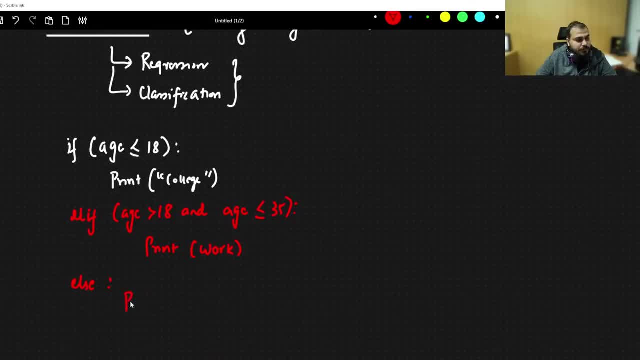 Else, I am just going to consider print retire. So here is my if else condition over here. Here is my if else condition. you can see over here: Now, whenever we have this kind of nested if else condition, What we can do is that. 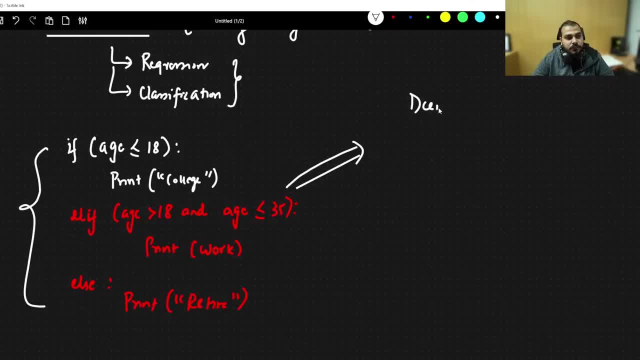 We can also represent this in the form of decision trees. We can actually form this in the form of decision tree And the decision tree here. first of all, we will have a specific root node. Let's say this is my root node. Now, in this root node, the first condition is less than or equal to 18.. 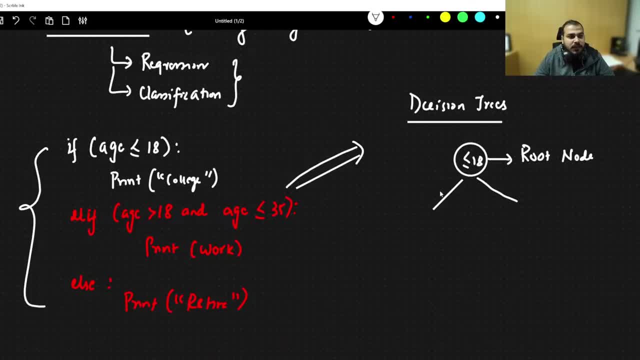 So here, obviously, I will be having two conditions, saying that if it is less than or equal to 18. And one condition will be yes And one condition will be no. So if this is yes and if this is no, If this condition is true, that basically means we will go in this side. 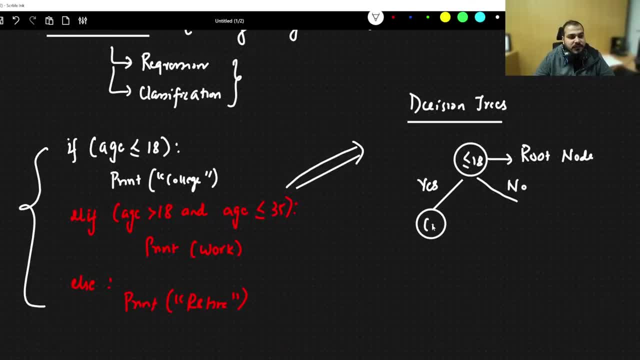 If it is true, then here we will basically have something like college. So this is your leaf node. Similarly, when I have no No in this particular case, we will go to the next condition. In this next condition, I will again create a node. 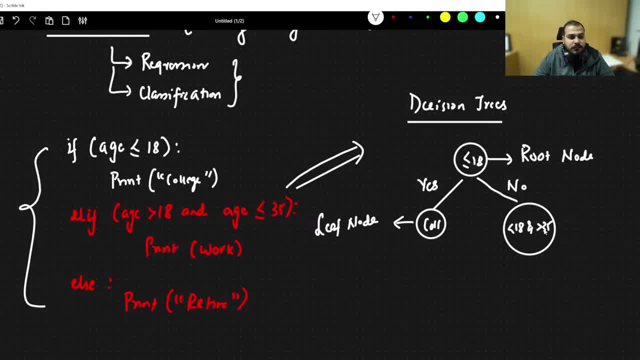 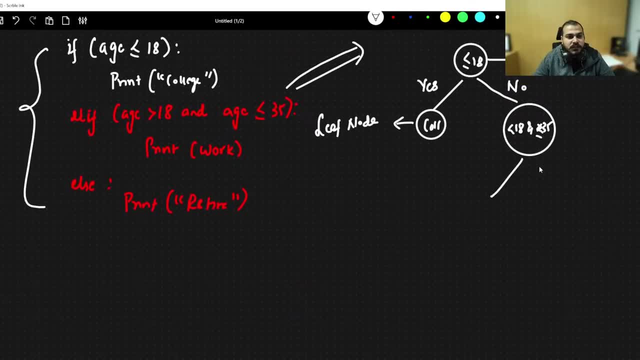 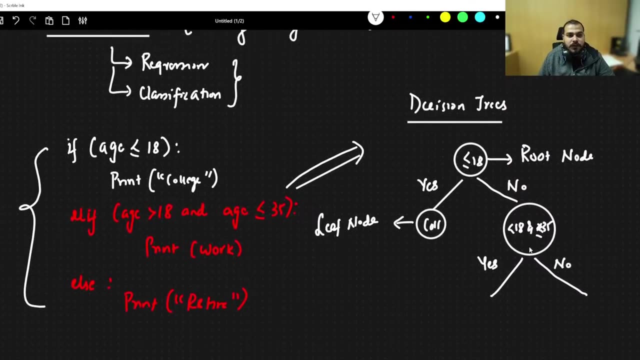 And I will say that, Okay, this is less than 18 and greater than- sorry, less than or equal to 35. So if this is also there, then again I will have two conditions, which is basically yes or no. Okay, Now, when I create this yes or no over here, you will be able to see. 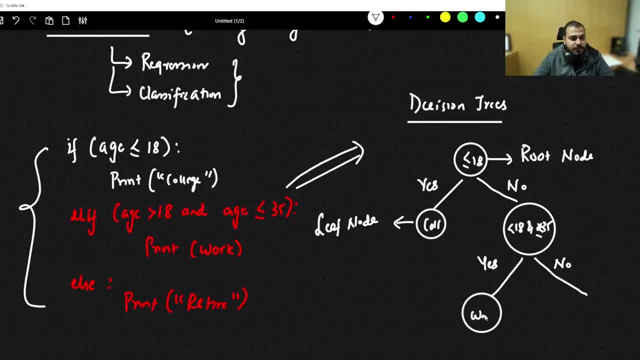 That basically means here again two condition will be there. If it is yes, I will say: print work, So this will again be my leaf node. And again for no, Again. Please note here: So yes, So here you can see that. 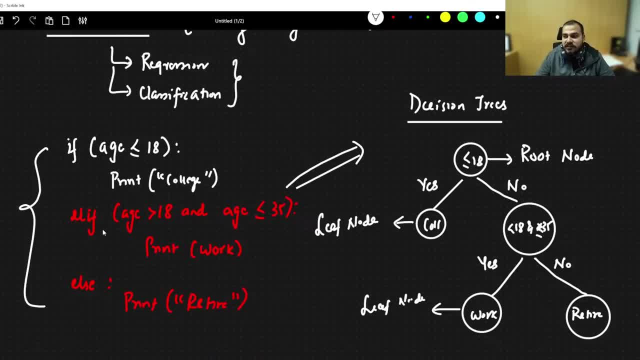 Once again I will complete my for another condition And once again I will say yes or no over here. Then once again, the result display will be green. Come over here again at mark 11.. In this form, two conditions are the one: improvement. Producer's fashion underscore. 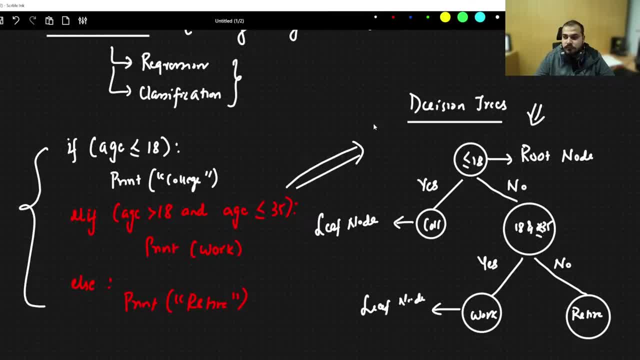 How about that? Oh Oh, So again, some try again can't help. ok again, if it is greater than 18,. ok, and less than 35,. so can we solve a regression and a classification problem? regression and classification problem. 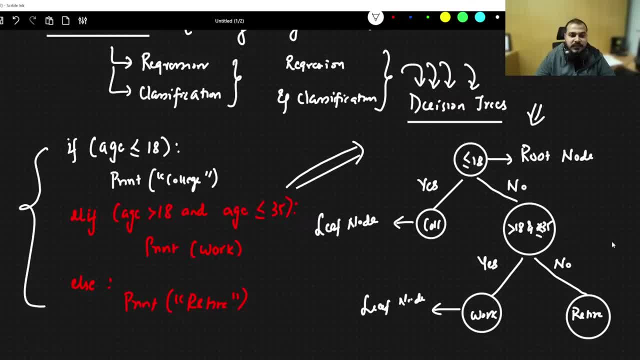 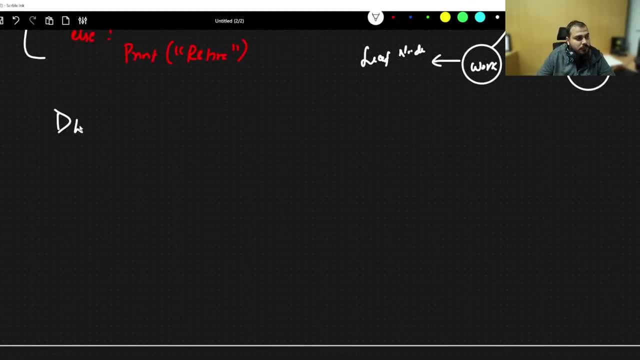 using this decision trees by creating this kind of nodes. so, in short, whenever we talk about decision trees, whenever we talk about decision trees, you will be seeing that decision trees are nothing but decision trees are nothing but by using this nested, if else, 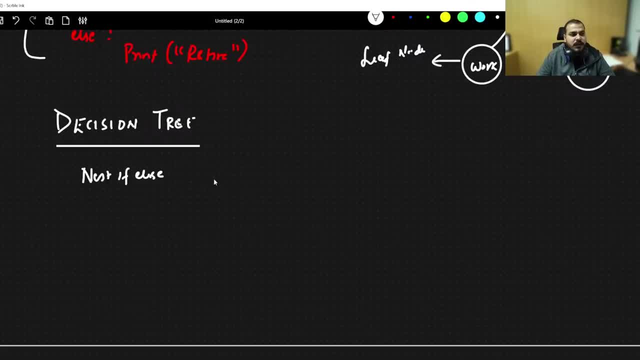 condition. we can definitely solve some specific problem statement, But here, in the visualized way, we will specifically create this decision tree in the form of nodes. Now you need to understand that what type of maths we will probably use. ok, so let's. 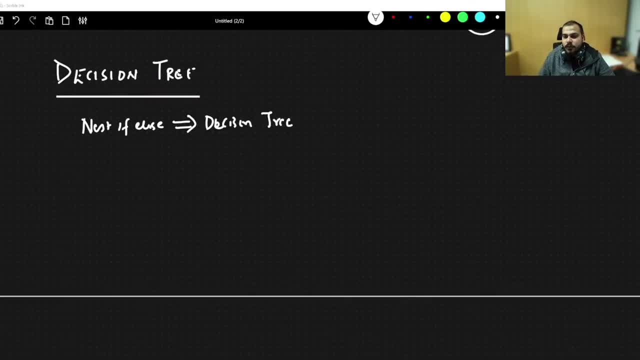 do one thing. let's take a specific data set, which I will definitely do it over here in front of you, ok, and we will try to solve this particular data set, and this will basically give you an idea like how we can probably solve this problem. ok, so let me just open. 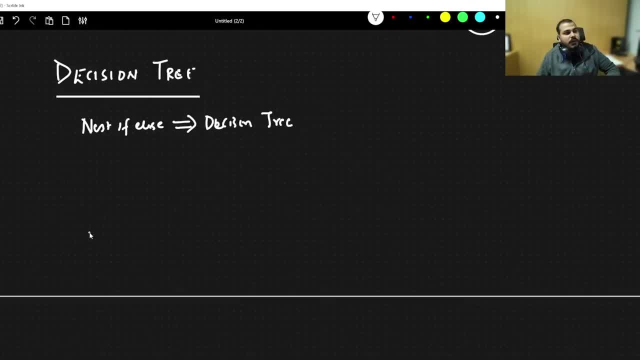 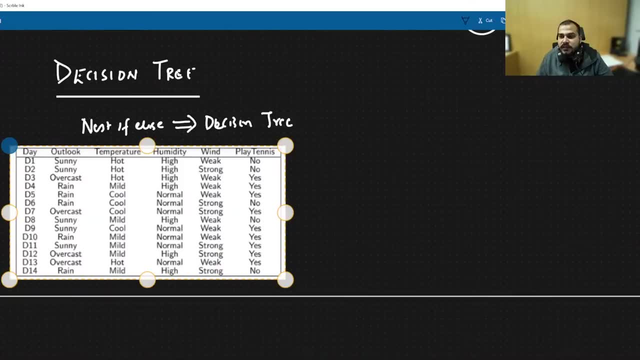 my snippet tool. So this is my data set that I have. ok, let's consider that I have this specific data set. I hope everybody is able to see this data set. ok, now this data set are pretty much important because this probably in research papers also, probably people who have come. 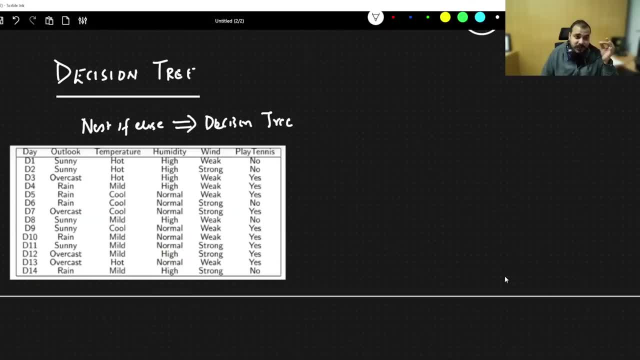 up with this algorithm. they usually take this, they take this thing, but right now, this particular problem statement, if I talk about this, is a classification problem statement. ok, So I will also help you to explain. I will also explain you about regression also how. 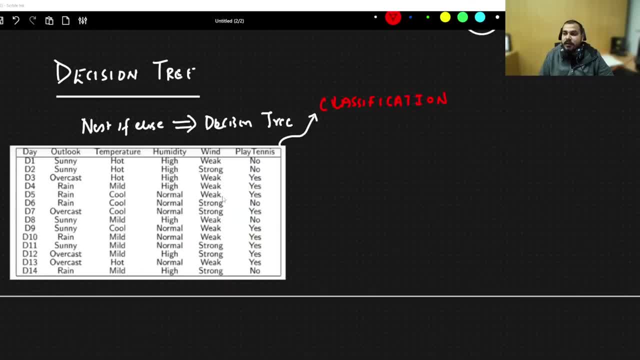 decision tree regression will definitely work, ok, So let's go ahead and let's try to understand. suppose, if I have this specific problem statement, how do we solve this? So this is my output feature: play tennis, yes or no? ok, whether the person is going. 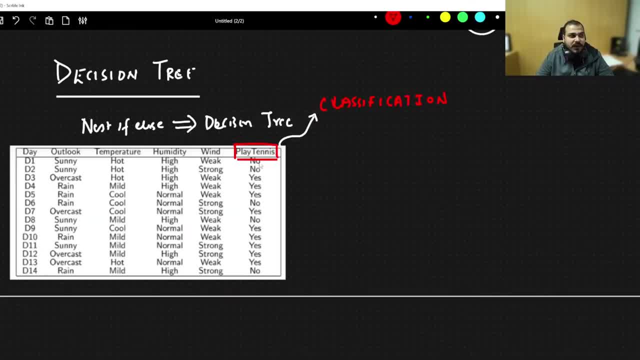 to play tennis or not, yesterday or day after yesterday or whenever you want? ok, so if I have this input feature, Like outlook, temperature, humidity and wind, is the person going to play tennis or not? this is what my model should predict with the help of decision tree. 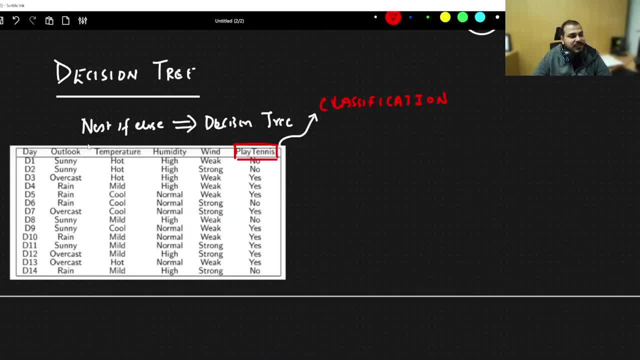 So how decision tree will work in this particular case. first of all, let's consider any, any, any specific feature. let's say that outlook is my feature, so this will be my first feature, which is specifically outlook. ok, now just tell me how many. how many are basically having? 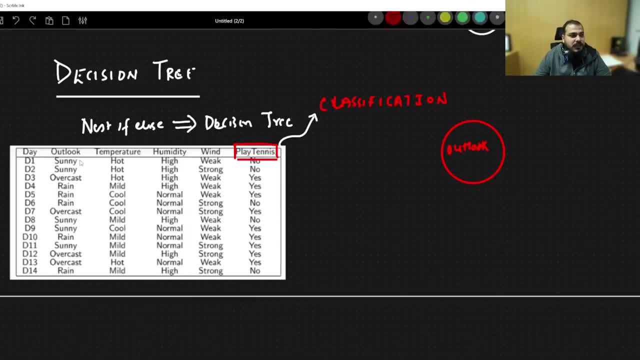 no's and how many are basically having yes in the case of outlook, how many total number of yes are there? how many total number of yes are there there? you will be able to find out. there are 9 yes, see 1,, 2,, 3,, 4,, 5,, 6,, 7,, 8,, 9. and how many no's are there? 1,, 2,. 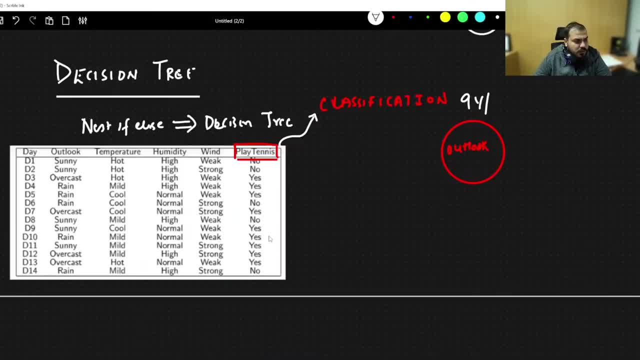 3,, 4, 5, I think 1,, 2, 3, 4, 5, so 9 yes and 5 no's are there, ok? So what we are going to do in this specific thing now we have 9 yes and 5 no's and the 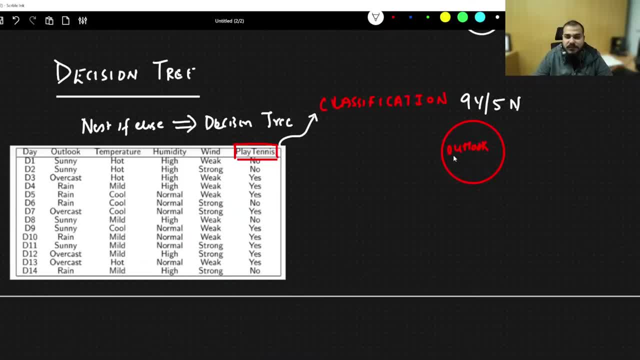 first node that I have actually taken is basically outlook. ok, so outlook feature. now just try to find out. we are focusing on this specific feature. I want to focus on this specific feature. ok now, in this feature, how many categories I have? I have one sunny category. 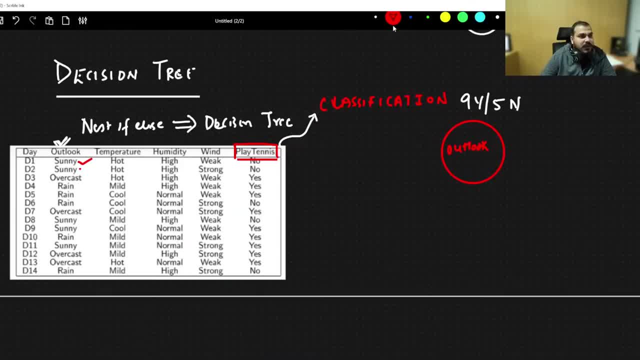 you can see over here I have sunny one category- Ok. Then I have another category called as overcast. then I have another category as rain- ok, so I have 3 unique categories. so based on these 3 categories, I will try to create 3. 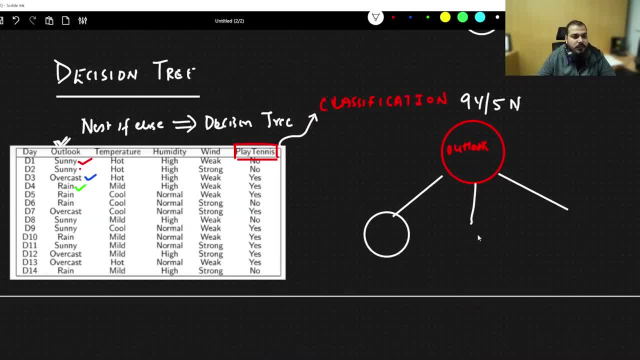 nodes. ok, so here is my 1 node, here is my 2nd node, here is my 3rd node. ok, so these are my 3 categories. so this category is basically called as sunny. this category is basically: 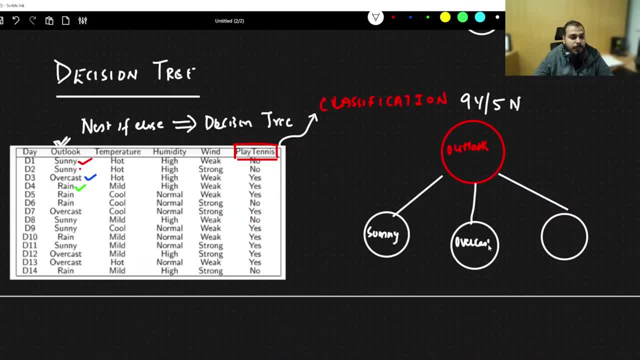 called as overcast and this category is basically called as rain. ok, so, based on these 3 categories, so I am splitting it now, just go ahead and see in sunny. how many yes and how many no are there? ok, how many yes with respect to sunny are there? see in. 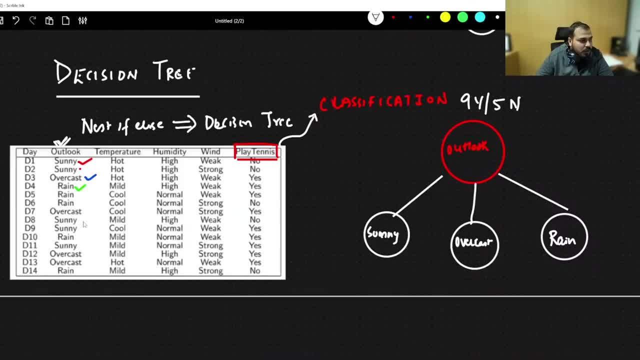 sunny, I have 2 no's, see 1 and 2 no, 1 more no, is there 3 no's? so here you can see: this is my 1.. Then this is my 2. no, this is my 3. no, right, and yes are 2,. so this 1 and this 1, so how? 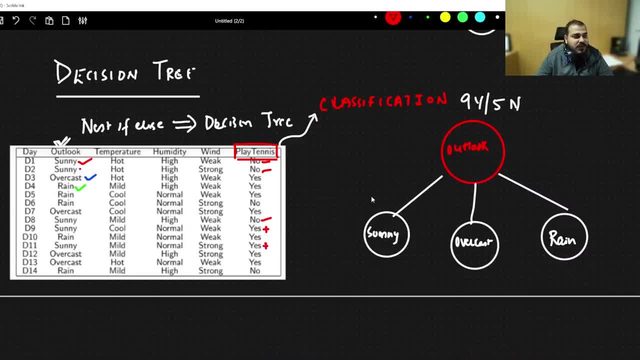 many total number of yes? how many total number of yes are here? ok, how many total number of yes are here? so here you can see that there are 1, 2, 2 yes and 3 no. ok, Rishi. 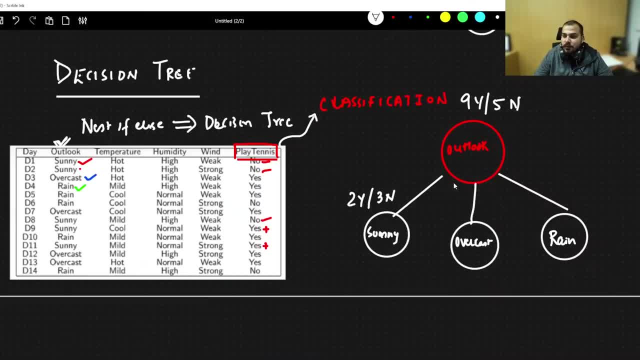 Chavan, don't spam. I will explain why it is taken as outlook, as a specifically I have just randomly selected right now. ok, I will talk about it. don't worry, let's say that I have randomly selected one feature, which is outlook. ok, I will talk about it why. 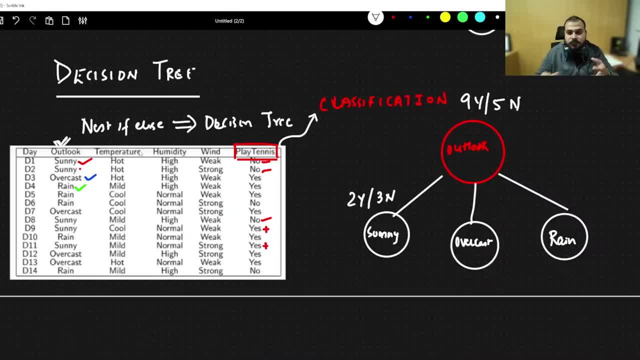 I have specifically. why can't I when, like, see it is up to it is up to the decision tree to select any of the feature? here I have specifically taken outlook. later on I will explain Why. Because it can basically select how it selects the feature. ok, I will talk about it, don't. 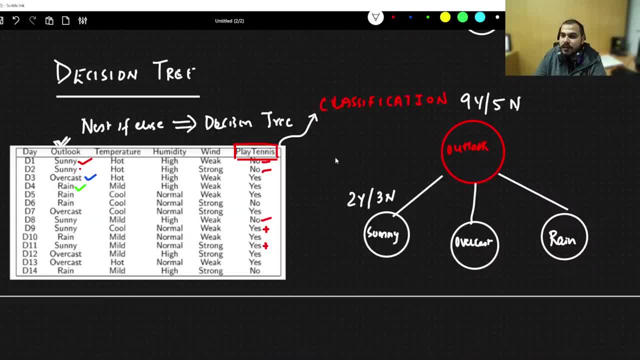 worry Guys, one request to you all: just trust me, ok, and focus on the session. I am telling you, in the world, no YouTuber has come and explained, live in front of you, any algorithms. ok, and so trust me, learn things and don't worry about anything. I will try to cover. 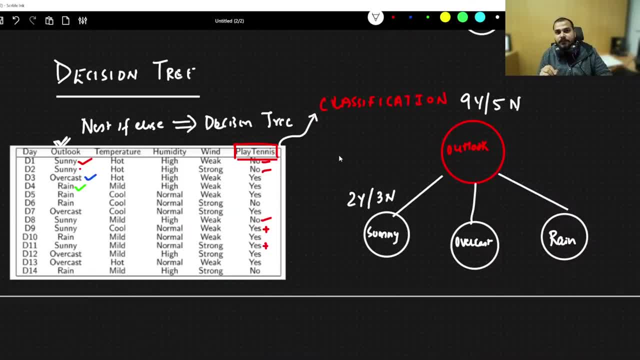 up anything that is available in this algorithm. Ok now some guys will ask about deep learning, some guys will ask about this, that that way, you will also not be able to learn, and my mind will also get disturbed if my mind gets. 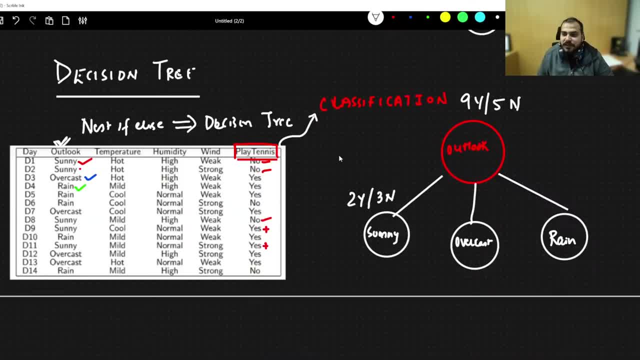 disturbed. many things get skipped, ok, so don't do it. focus on the lesson instead of focus on anything else. at last I will see your queries and then we will try to solve it. ok, So in the outlook we have two yes. sorry, in the case of Sunny, we have two yes and. 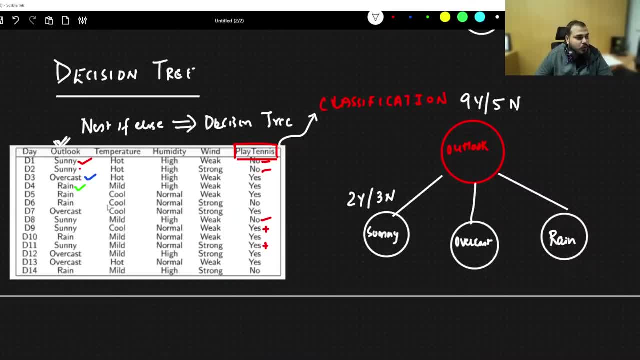 three no's- ok. now the next thing is that let's go and see for overcast. in overcast I have one yes. two yes, three yes and four yes. I don't have any no in overcast. so over here my thing will be that four yes and zero no's ok. four yes and zero no's. 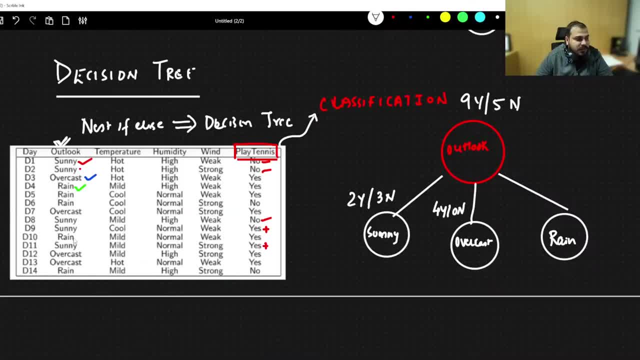 ok, So in the rain part, see in rain. how many features are there in rain? if you go and probably see it, how many number of yes and no's are there? go and see in one one yes, in rain two yes, then one no. then again you have one yes and one no, right? so here? 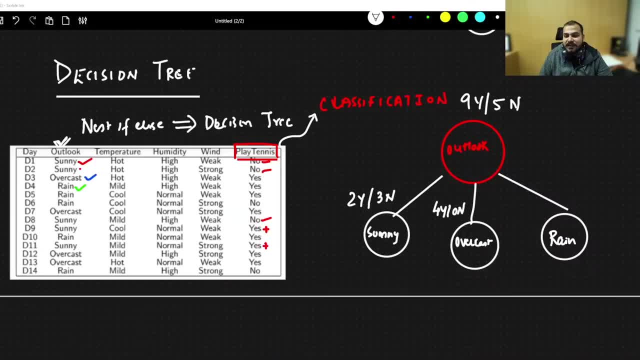 you can basically say that in rain, in the case of rain, if I take an example, how many number of yes and no's are there? you just tell me now It will be three yes and two no's. ok, understand, understanding algorithm. ek baar samajh loge. 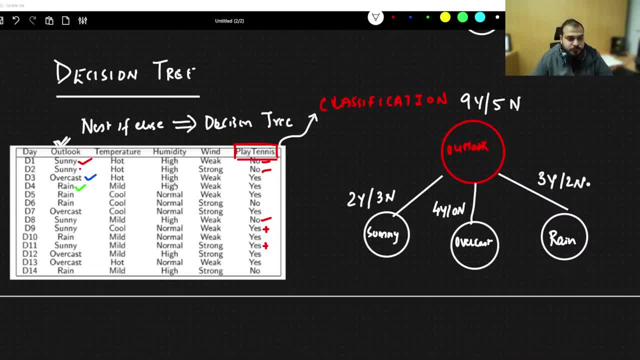 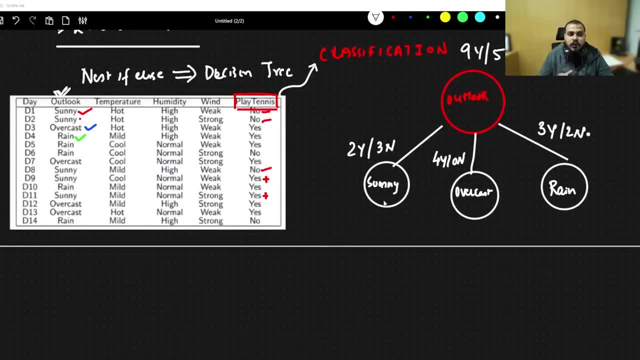 then everything will. you will be able to understand. ok, ok, perfect. Now these all are there. ok, now see this. now let's go ahead and try to see for Sunny. Sunny definitely has two yes and three no's. this has four yes and zero no's. here you 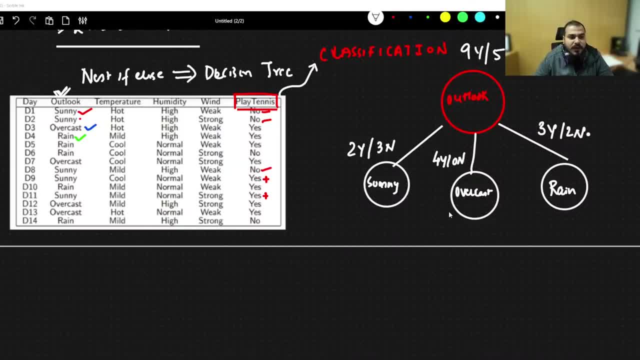 have three y's and three no's. Ok, Three y's and two no's, now if I probably take overcast. ok, over here. here you need to understand about two things: one is pure split and one is impure split. now what does? 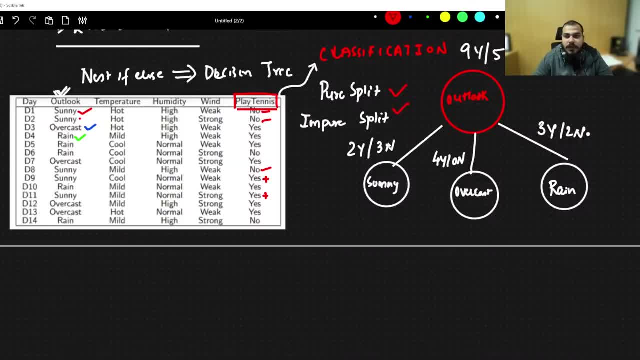 pure split basically mean. ok, what does pure split basically mean? pure split basically means that now see in this particular scenario, in overcast, in overcast I have either yes or no. So here you can see that I have four yes and zero no's. so that basically means this is: 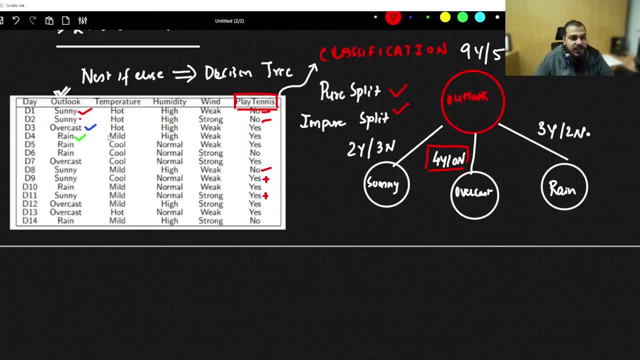 a pure split. anybody tomorrow in my data set, if I just take this outlook feature, suppose in one day, in day 15, the outlook is outlook is basically overcast, then I know directly it is the person is going to play right. so this part is already created. 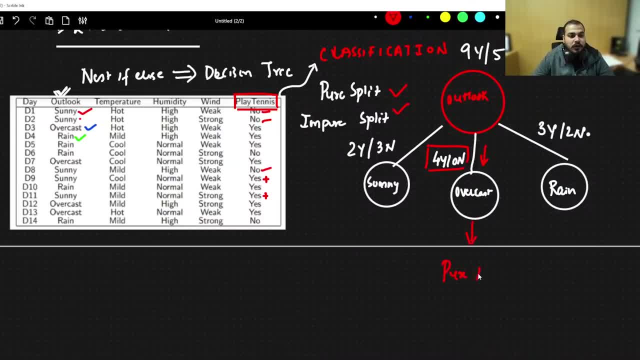 and this node is called as pure node. understand this. why it is called as pure node? Because either you have all yes or zero no's, or zero yes or all no's, like that. in this particular case, I have all yes. ok, so if I take this specific path, I know that with 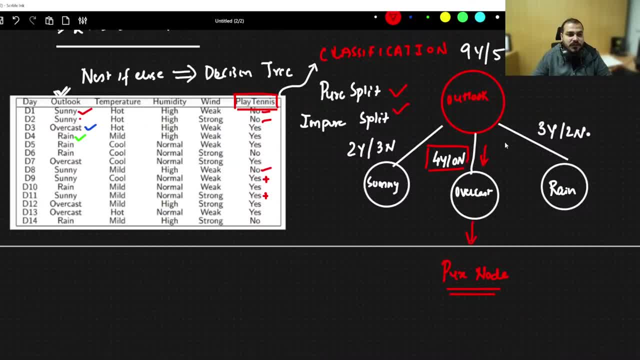 respect to overcast my final decision, which is yes, it is always going to become yes. ok, so this is what it basically says, so I don't have to split further. so, from here, I will probably not split, not split, I will definitely not split, I will definitely not. 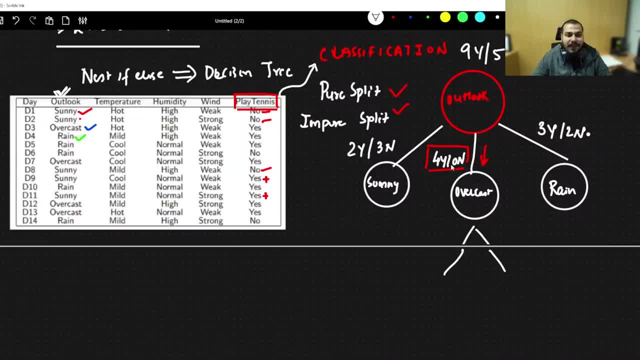 split more because I don't require it, because I have. it is a pure leaf node. ok, you can also say that this is a pure leaf node, so I am just going to mention it again. so this is a pure leaf node, this one I am specifically talking about. now let's talk about sunny. 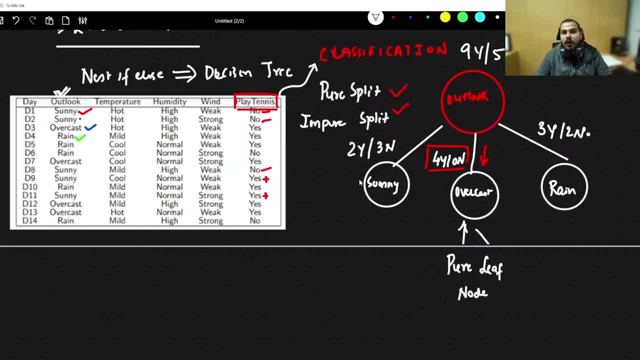 in the case of sunny, you have two yes and three no's, so this is obviously impure. so what we do? We take next feature. and again, how do we calculate that? which feature we should take next? I will discuss about it. let's say that after this, I take up temperature, I take 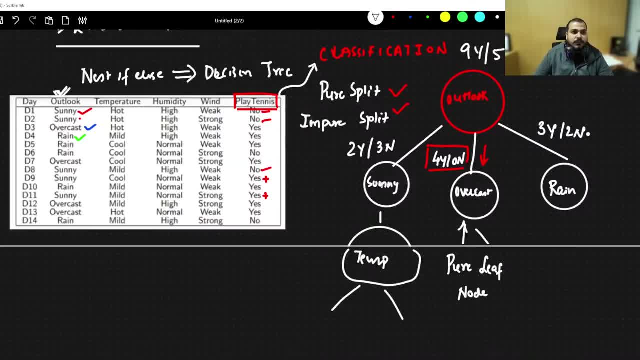 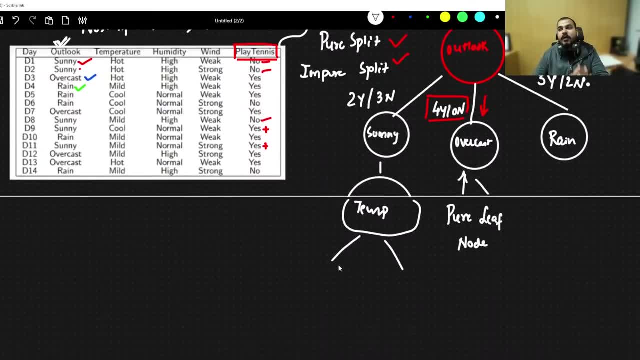 up temperature and I start splitting again. ok, since this is impure. ok, and this split will happen until we get finally a pure split. ok, similarly, with respect to rain, we will go ahead and take another feature and we will keep on splitting. 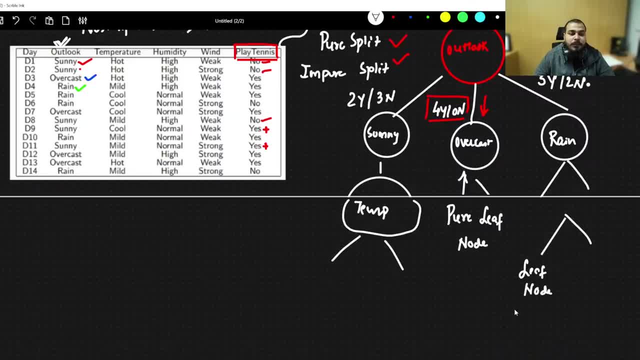 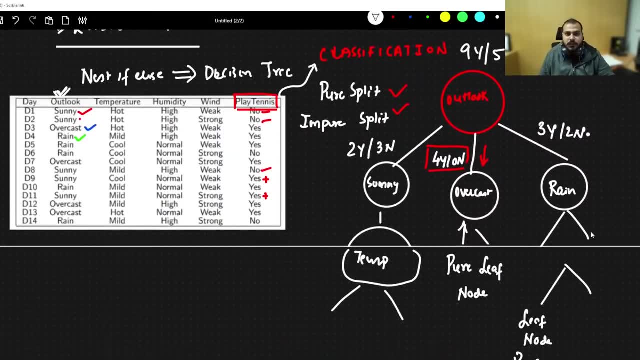 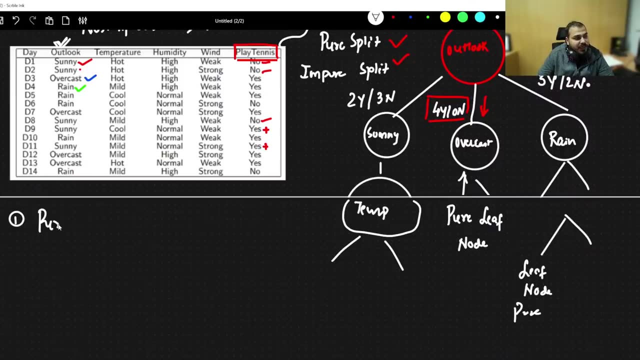 We will keep on splitting unless and until we get a leaf node which is completely pure. ok, so I hope you understood how this exactly works. ok, now two questions. two questions, is that, Krish? the first thing is that: how do we calculate this purity and how do we? 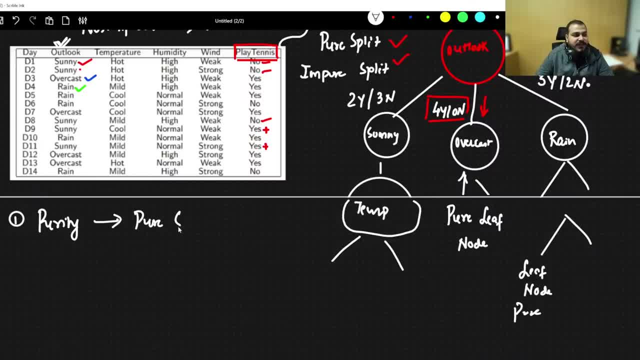 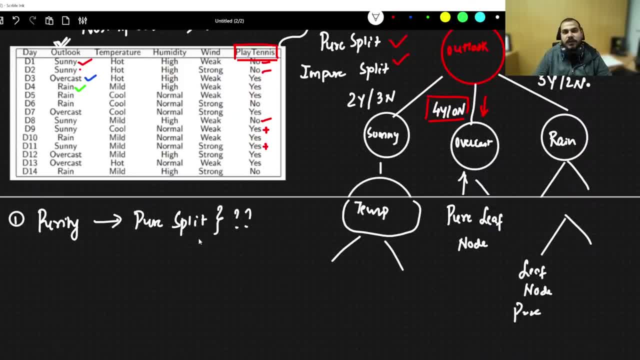 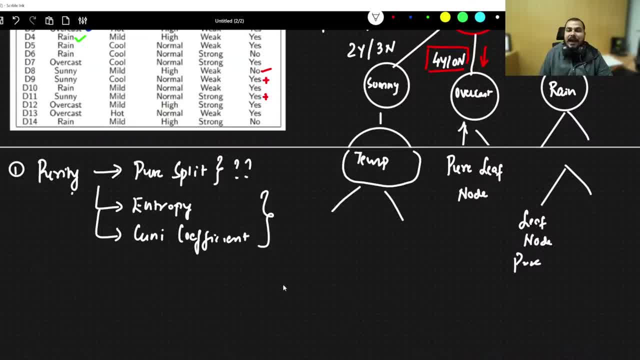 so we will try to understand how does entropy work and how does Gini coefficient work in decision tree, which will help us to determine whether the split is pure split or not, or whether this node is leaf node or not. if node or not, okay then, coming to the second thing. okay, coming to the second thing. one is: 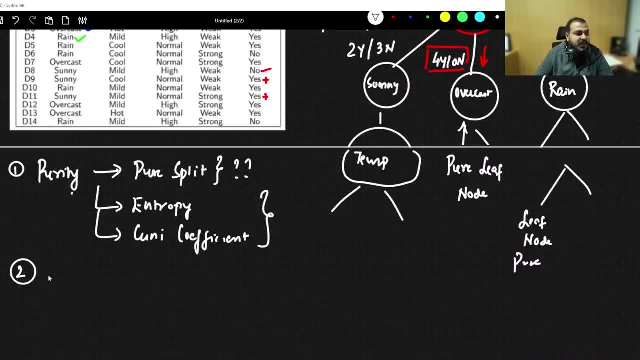 with respect to purity. second thing, your first, most important question which you had asked: why did i probably select outlook? how the features are selected, how the features are selected. this is the next question that i need to answer, and here you have a topic which is called as information gain, and if you know this, both, your problem is solved okay. 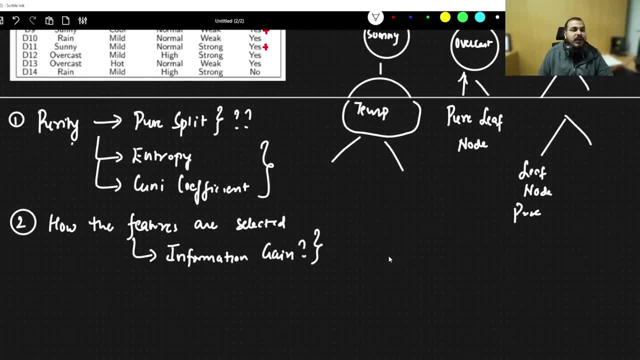 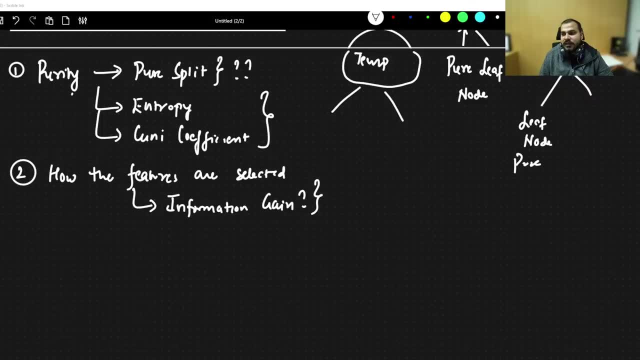 so now let's go ahead and let's understand about entropy or guinea coefficient or information gain, okay, so i hope can i get a confirmation. you have understood till here. yes, i hope everybody is understood till here. entropy or guinea coefficient or sorry, guinea coefficient, i'm saying guinea impurity also you 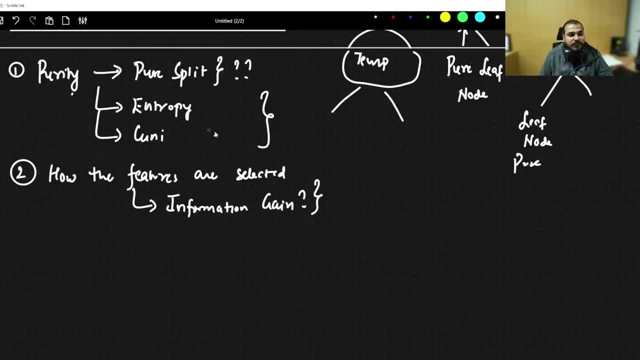 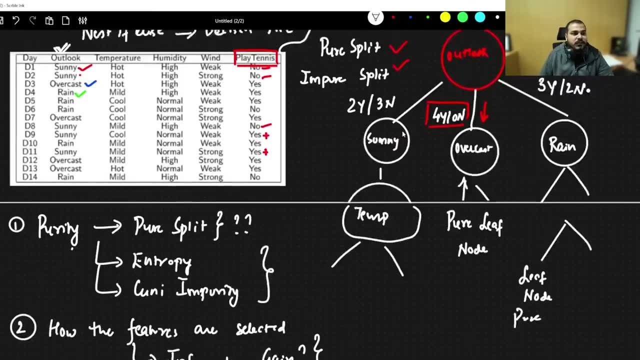 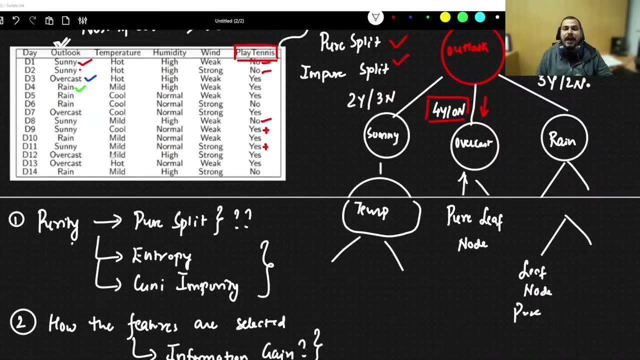 can say over here. i'll write it as guinea impurity, not coefficient. also, i'll just say it as guinea impurity. but i hope everybody is understood till here, right, everybody understood about the splitting mechanism, what funda we are going to use. okay, right now let's go ahead and 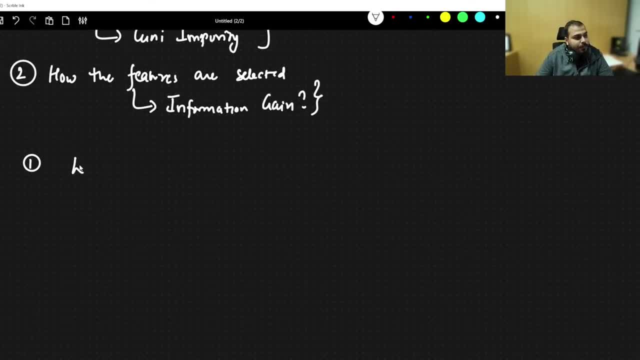 let's discuss about the first thing, that is, entropy. how does entropy work and how we are going to use the formula? so entropy- here i will just write guinea, guinea, impurity. so we are going to discuss about this, both the things, okay, okay, so we are just going to discuss about this. please make sure that you hit the like button. 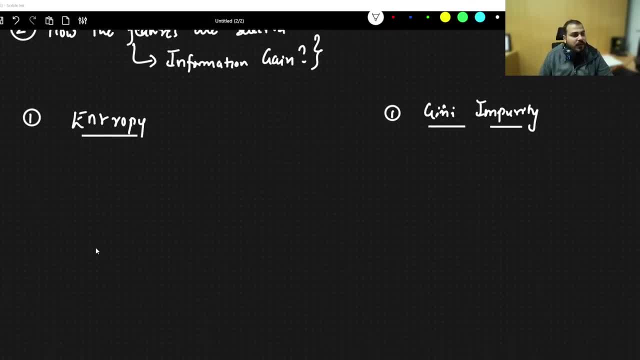 okay, and let's go ahead. okay, let's say that the entropy formula which is given by- i will write h of s is equal to. again, guys, i'm not going to derive this formula because you need to understand how the decision tree is actually working. i will discuss about each and every. 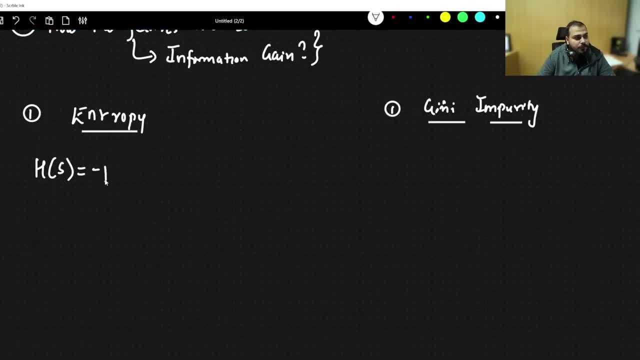 component of the entropy formula which is given by. i will write: h of s is equal to the components that is present in the formula. so h of s is equal to minus p plus. i'll talk about what is minus. what is p plus: log base to p plus, minus p minus, log base to p minus. so this is the. 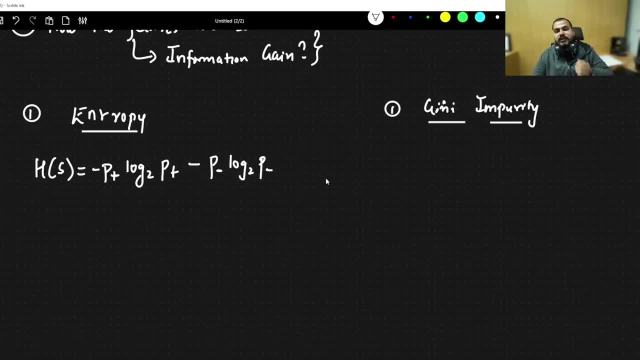 formula for entropy. everybody write it down. i will discuss about each and every component, don't worry. okay. and in guinea, impurity, the formula is one minus p plus log base to p minus. so this is the formula for entropy. everybody write it down. i will discuss about each and every component, don't worry. 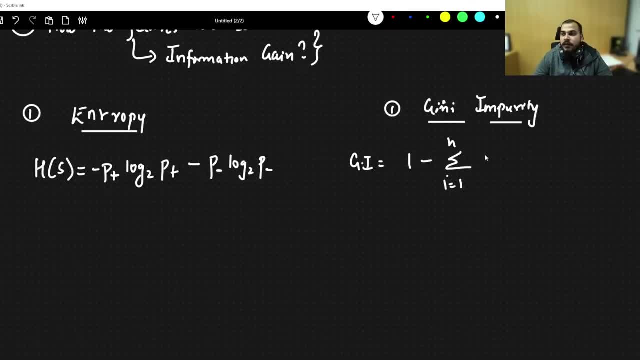 okay, and in guinea impurity the formula is one minus p plus log base to p plus log base to p minus summation of i is equal to one to n p square. i'll even talk about when you should use guinea impurity, when you should not use guinea impurity, when you should use entropy, you know by default. 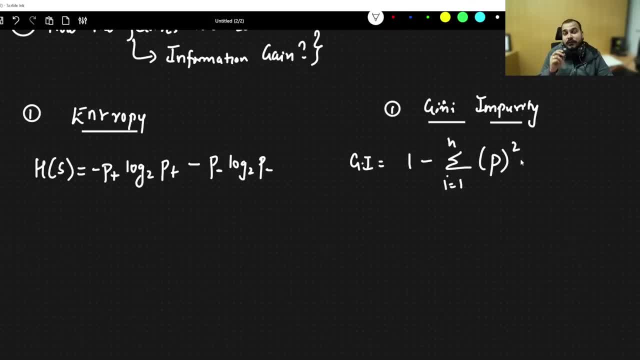 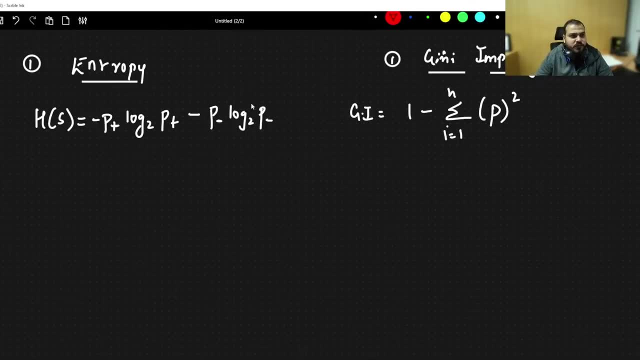 the decision: tree regressor or classification. sorry decision: tree classification uses guinea impurity. okay, now let's take one specific example. so my example is that i have a feature one, my root node. i have a feature one, my root node. i have a feature one, my root node. 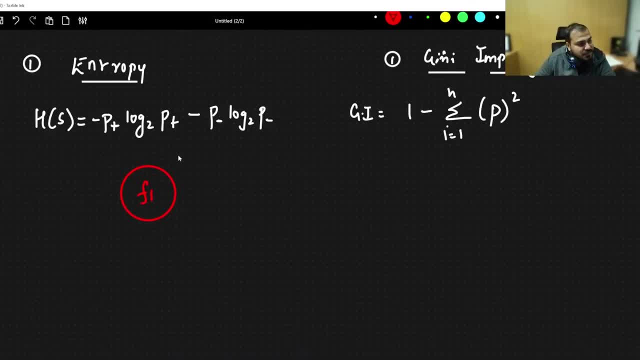 and let's say that in this root node i have six yes and three no's. okay, very simple. let's say that this has two categories and based on these two categories of split has happened. that is c1. let's say, in this i have three yes, three no's, and here i have three yes, zero no's. okay, and this is my. 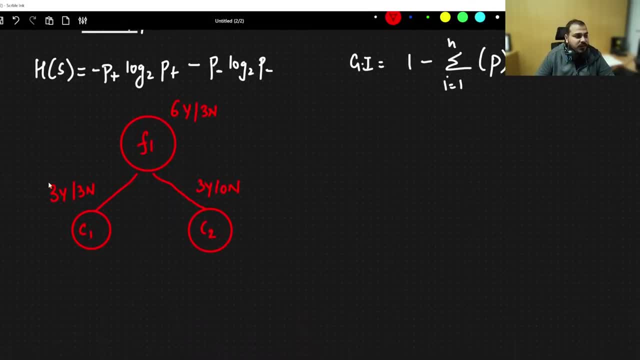 second category always understand: if i do the summation, three yes and three yes is six yes, see this, this submission. if i do three plus three is obviously six. three plus zero is obviously three. okay, so this you need to understand. based on the number of root nodes, only almost it will be same. 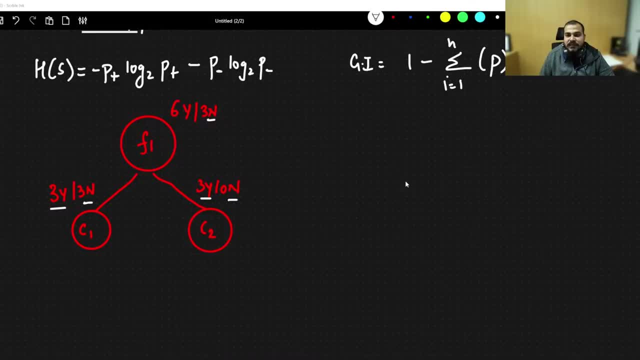 okay, now let's go ahead and let's understand how do we calculate. let's take this example: how do we calculate the entropy of this? so i have already shown you the entropy formula over here. now let's understand the component. okay, i will write: h of s is equal to minus sign. is there what is p plus? p plus basically means that 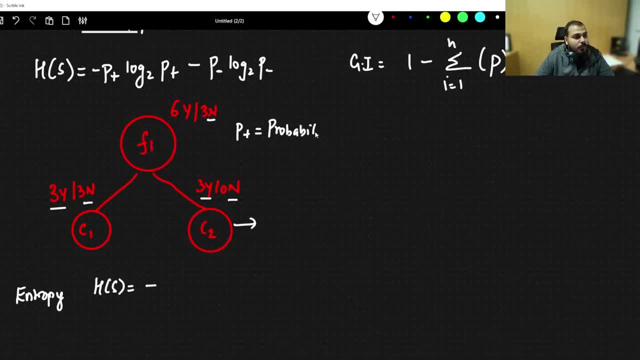 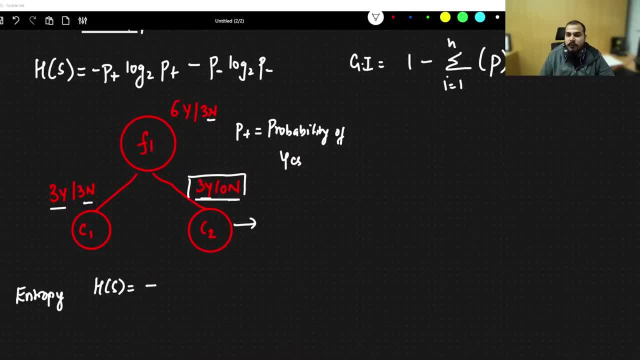 probability of yes out of this. so obviously how you'll write if you want to find out the probability of yes out of this. so obviously how you'll write if you want to find out the probability of yes out of this. see, when i say plus, that basically means yes, okay. when i say: 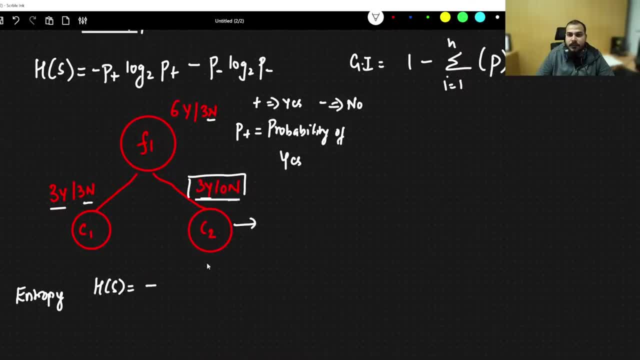 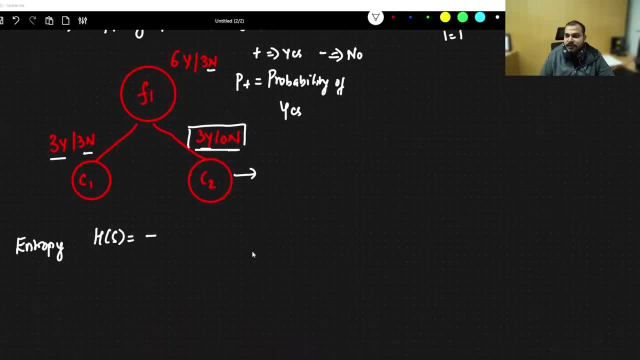 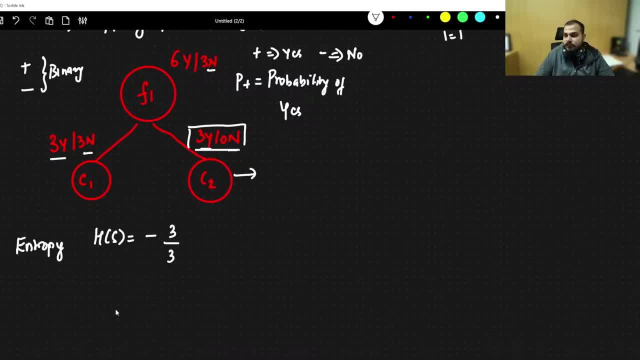 probability with respect to yes, can i write three by three? can i write three by three everyone? can i write three by only for this? only for this? what is the probability out of this total number of this? is there three by three right? similarly, if i go and see the next term log to the base two p plus. so again, if i go ahead and 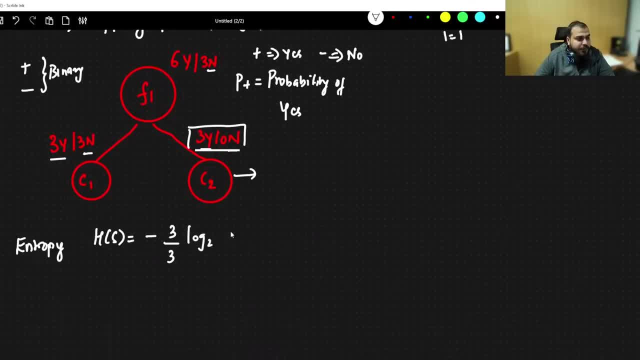 write over here: log to the base two: p plus p plus is again three by three. okay, so then again we have minus and this is now p minus. what is p minus? what is p minus? zero by three. log base two, zero by three. this obviously will become zero. this will obviously become zero because zero divided by anything is zero. 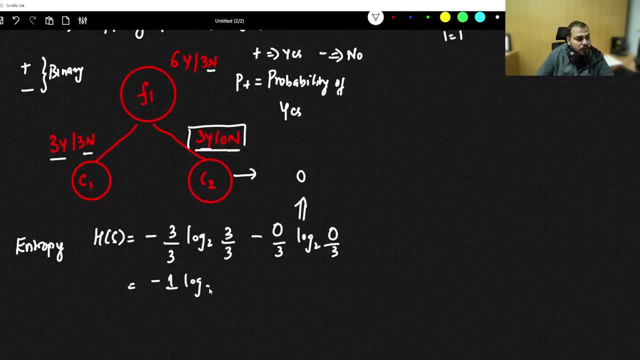 what will this be? one log to the base one. what is this? this is nothing but zero. log to the base one is nothing but zero. now see over here. tell me whether this is a pure split or impure split. tell me whether this is a pure split or impure split. 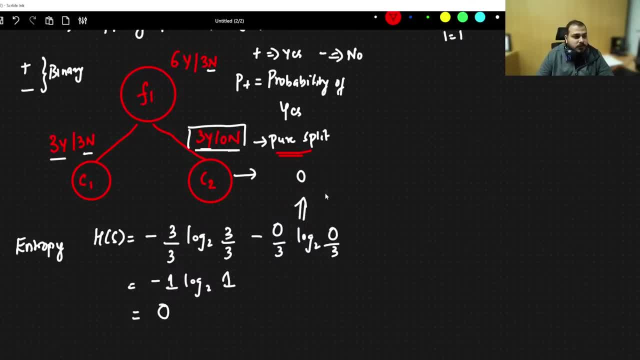 so this is a pure split. whenever we have a pure split, the answer of the entropy is going to come to zero. so here i'm going to define one graph. okay, here i'm going to define my graph. this is h of s. okay, and let's say: this is p plus or p minus, okay. 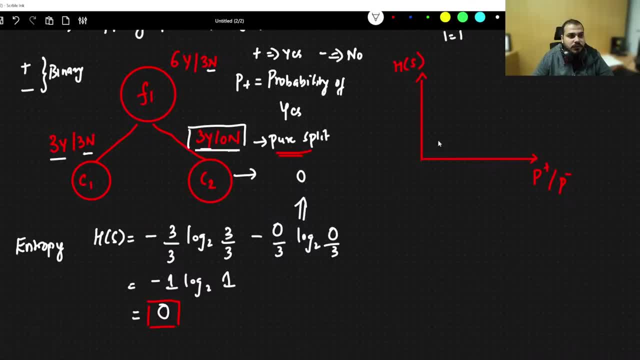 this is p plus and p minus. so if my probability of plus, see, when i say probability of plus is 0.5, what will be probability of minus? it will also be 0.5, right, because it's just like p is equal to 1 minus q, right? if p is 0.5, then q will be 1 minus p. same thing, right. so when it is 0.5. 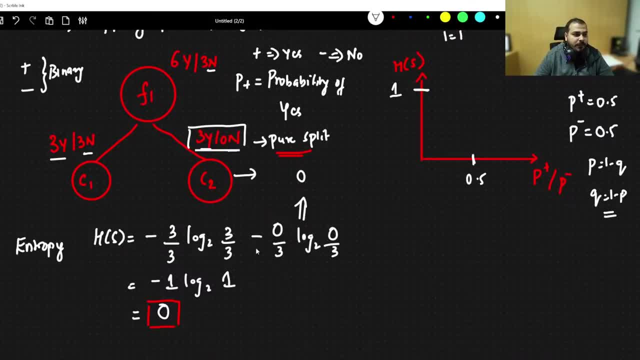 obviously, my h of s will be 1. okay, let's say so. this is the graph that will basically get formed, but don't worry, i will again explain you, since i did not come to the next part. let's go ahead and try to calculate the entropy of this. 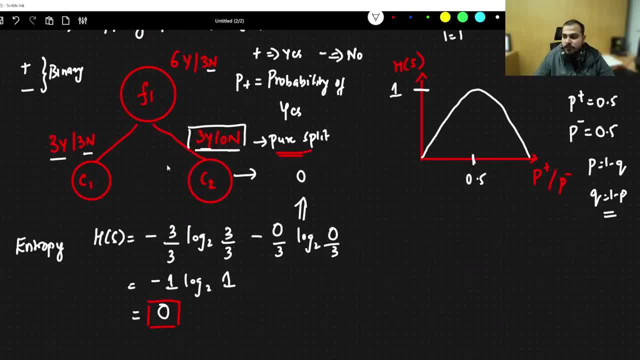 guys, what will be the entropy of this node? what will be the entropy of this node? okay, what is the entropy of this node, let's calculate. so here i'm going to write, so here i'm going to just make a graph h of s minus. what is p plus? p plus is nothing but three by six. 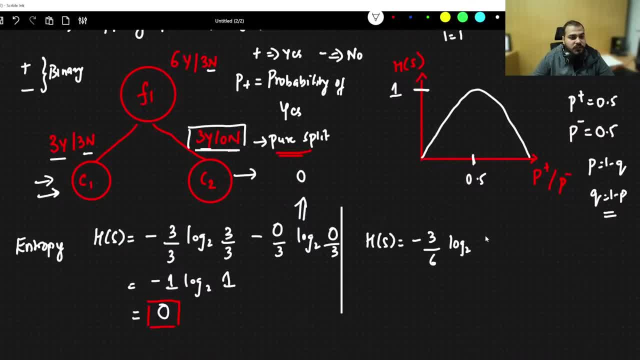 log base two, three by six. minus three nodes, are there three by six log base two, three by six. so if you compute this log base two to the power of one, if you do the calculation here i am actually going to get one. okay, here i am going to get one. you can basically go and check it out. 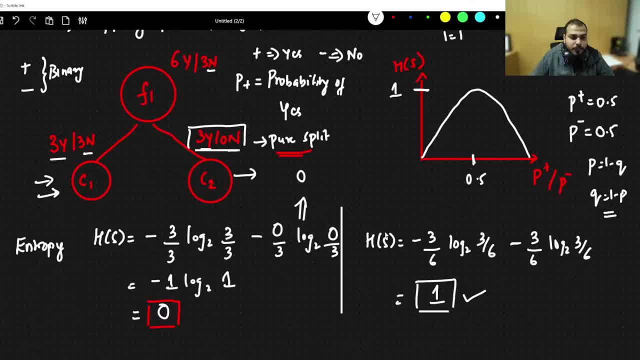 okay. so when i'm getting one, when i'm actually getting one, when you have three yes and three no's, what is the probability? it is 50, 50 percent, right? so when your p plus is 0.5, that basically means your h of s is coming as one. so from this graph you can see that i'm getting one. 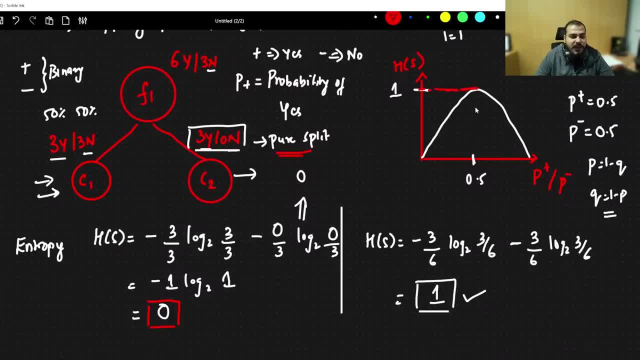 right, i'm actually getting one. if this is zero, this is one. right, this is zero and this is one. i hope everybody is able to understand this, so let's go ahead and do the calculation here, guys: zero and one right. if your p plus is zero or if your p plus is one, that basically means it. 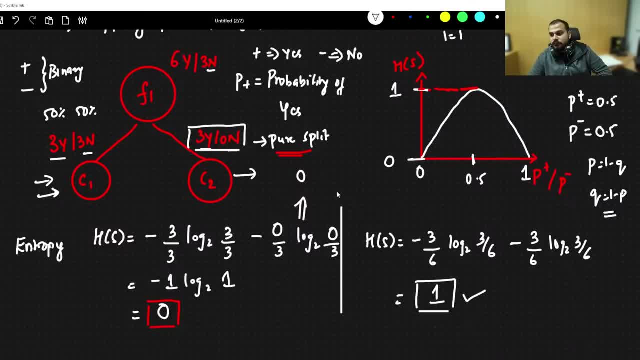 becomes a pure split. so in h of s you are going to get zero. so always understand: your entropy will be between zero to one. if i have an impure, this is a completely impure split because here you have 50 probability of getting yes, 50 probability of getting no. right, i hope everybody is able to understand yes or no. 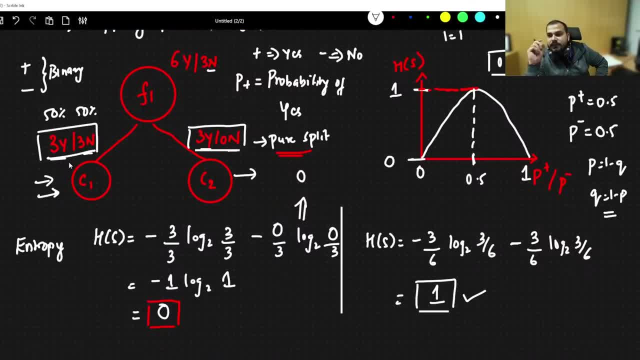 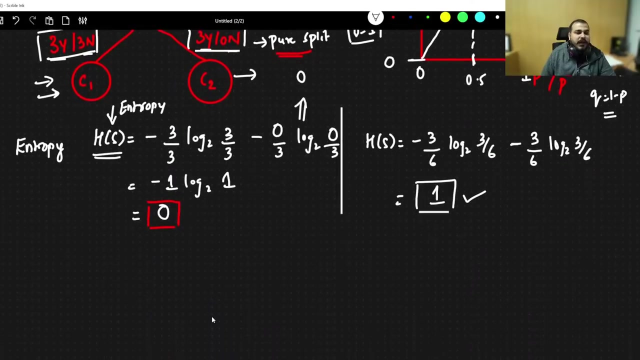 guys till here you are loving the session. your always entropy is going to between zero to one. clear, perfect wait for genie impurity. i will discuss about it. you want to go mars? then go mars. okay, h of s is entropy. this is entropy for the sample h of s notation that i'm using. is h of s right? so if, whenever the split is happening, the first 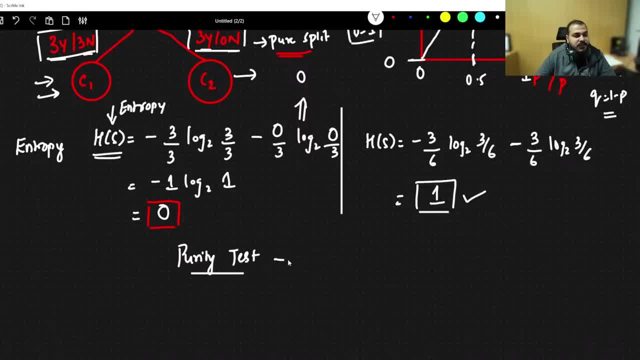 thing is done: the purity test. the purity test is done. the purity test is done. the purity test is done with the help of entropy. right now i'll also show guinea guinea impurity, don't worry. so with the entropy you will be able to find if i am getting one. that basically means it is a impure split. 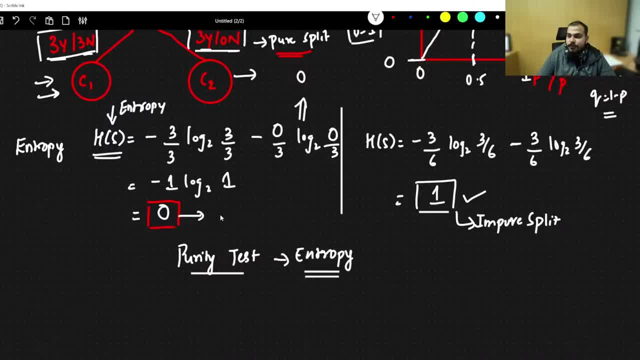 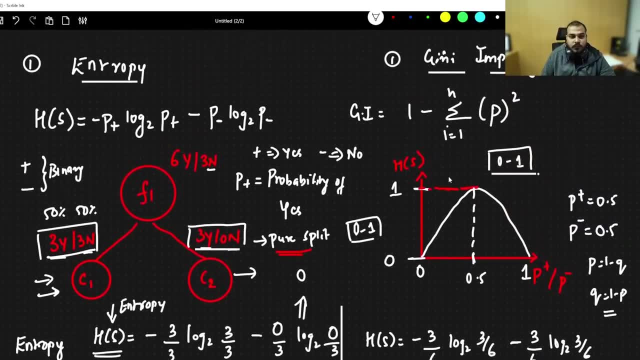 okay, and if i am getting zero, it is pure split. so this is the graph. okay, this is the graph, and this graph is basically the entropy graph, okay, okay, again understand: if your probability of getting yes or no is 0.5, that basically means 50- 50 is there three yes and three no's, then your entropy is going to be one h of s, okay. 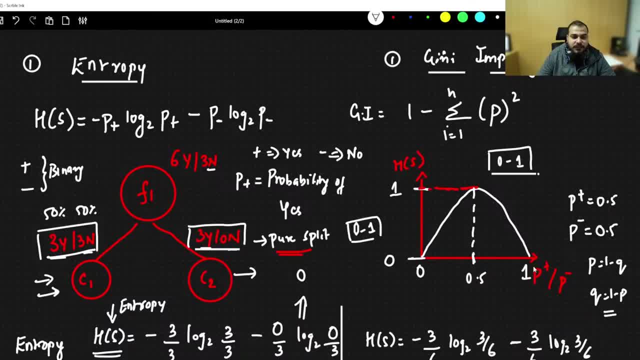 if your probability is completely one, that basically means either you are getting completely yes or completely no, so your your entropy will be zero. that basically means it is pure split. so in the case of probability 0.5, you are getting plus one. then it will keep on reducing. 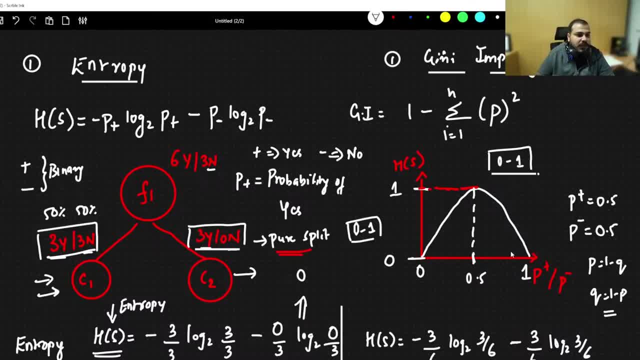 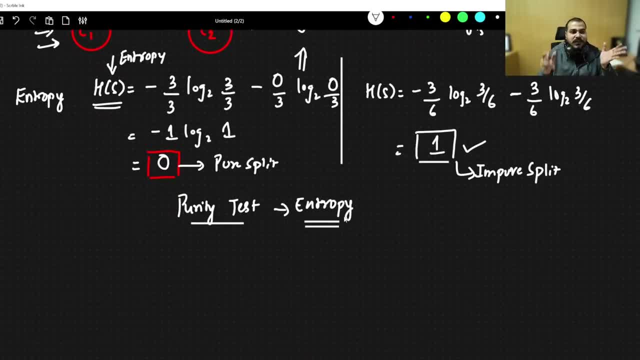 okay, now let's go ahead and let's try to understand. so here you have understood about purity test with definitely you'll use entropy, try to find out whether it is pure or impure. if it is impure, you go ahead with the further shift, further division of the categories. again you take another. 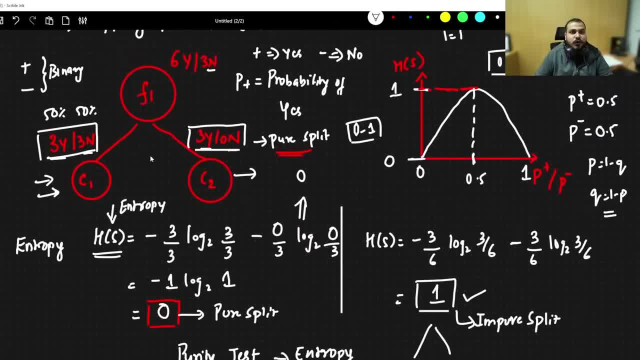 divide it, because here, from this two which split, you will do further, you will do this split as further. okay, if you are getting 0.6- 0.6 is this specific value- then you probably go and draw over here. this is your entropy. if your probability is here, which is 0.3, then you will go over here. 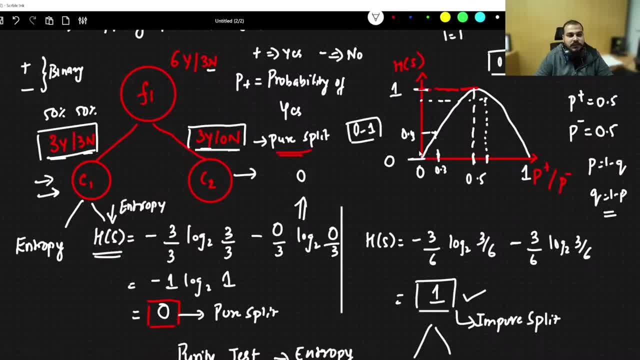 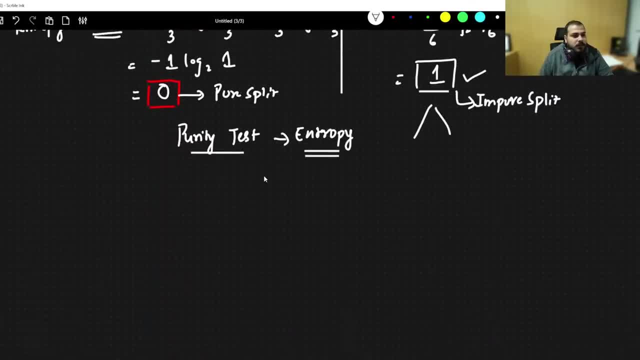 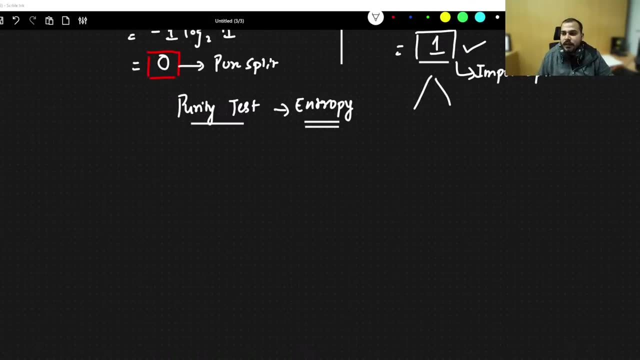 and create this. this may be 0.4 or 0.3, something like this. after this, it is getting vanished forever. okay, it will be between 0 to 1. it will be between 0 to 1. okay, let's go ahead and discuss about the. 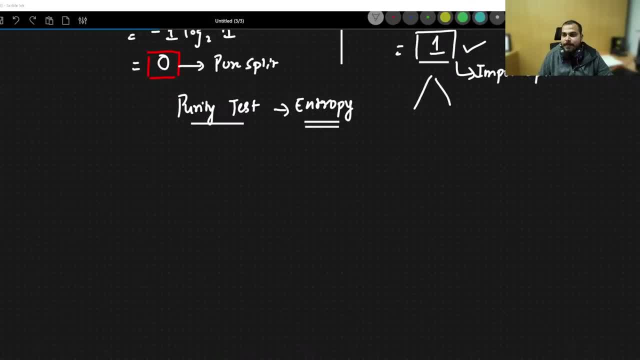 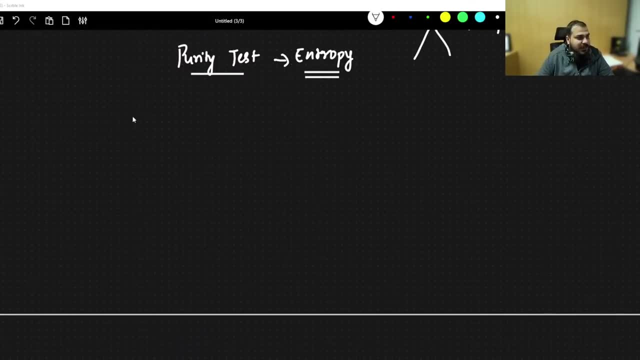 second issue i hope everybody is discussed about. we have discussed about checking the pure split or not, and we have understood this much right. but the next thing is that, okay, fine, krish, this is very good. you have explained well that I have some features. okay, now coming to the second problem: how do we consider which node to 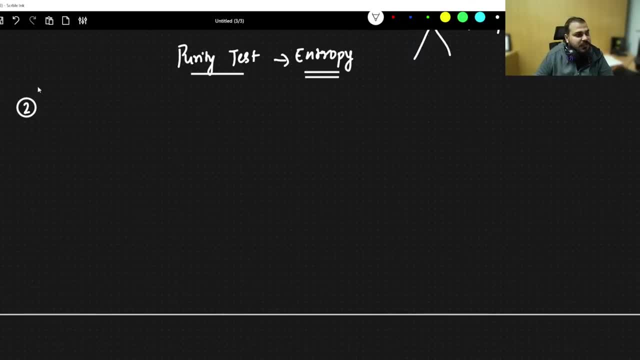 cap. which which feature to take and split, because here I may have one, one split. so again, let's see that. what is the second problem? which feature to take to split, to split right, this is the second problem that we are trying to solve. let's say that I have one feature, one over here, and I have 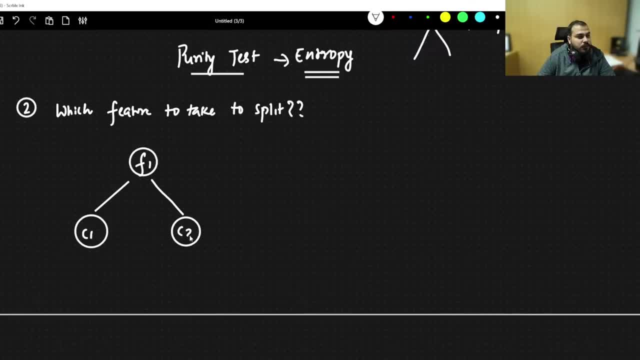 two categories. let's say this is their c1 and c2. okay, here let's say that I have 9 yes, 5 nose, and then I have 6 yes, 2 nose. here I have basically 3 yes and 3 nose. let's say: 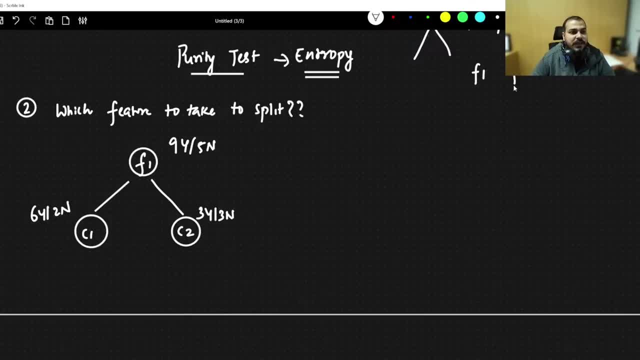 okay, and in my data set I have features like f1, f2, f3. okay, now let's say that another split. I can actually start with feature 2 also, and in feature 2 I may have probably three categories like c1 and c2, c1, c2, c3. so with respect to the root node and all the other features, because after this also, 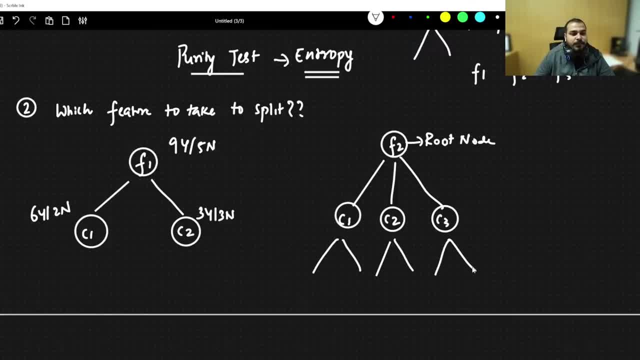 i may have to split right. i may have to take another feature and keep on splitting right based on the pure or impure split. how do i decide should i take f1 first or f2 first, or f3 first or any other feature first? how should i decide that? which feature should i take? and probably do the 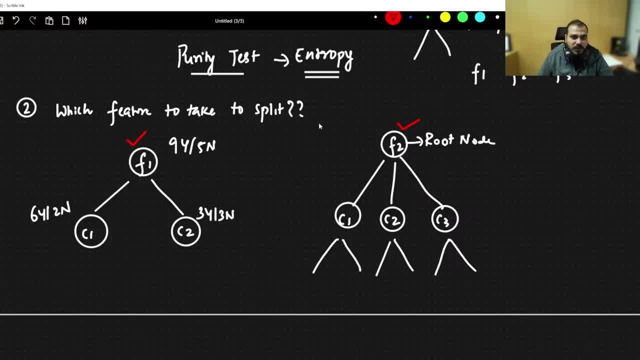 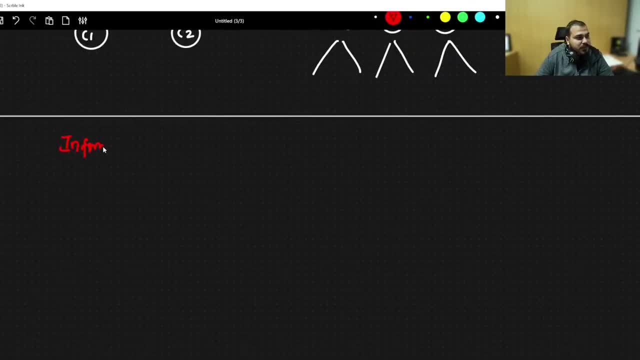 split. that is the major question. so for this we specifically use something called as information gain. so here i'm just going to say, here we basically use information gain. now, what is this information gain? i'll talk about it, okay, don't worry. so, information gain, first of all, i will 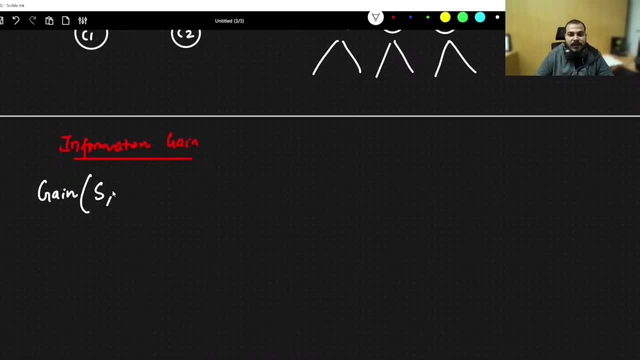 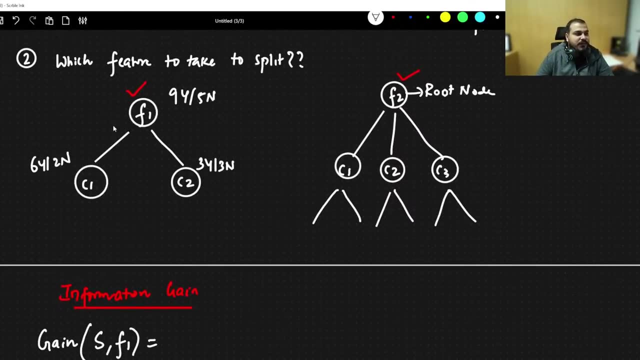 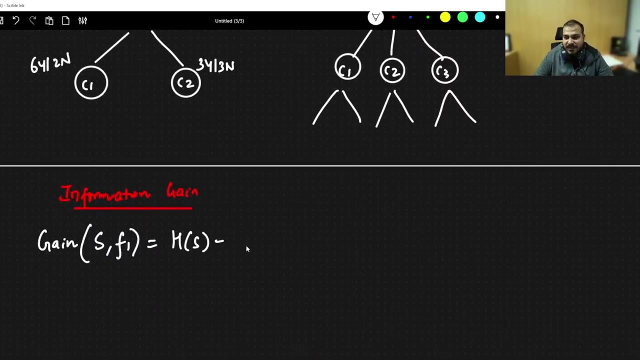 write the formula. we basically write gain with sample, first with feature one, i will compute. so first with feature one i will compute. suppose this is my first split of my data and probably i'm computing over here. this can be written as h of s. i'll discuss about each and every parameter. don't worry, summation of v belong. 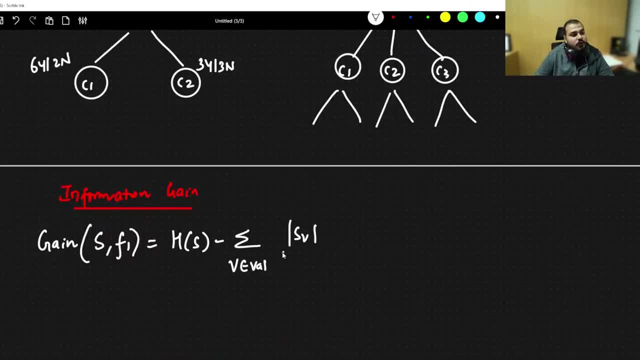 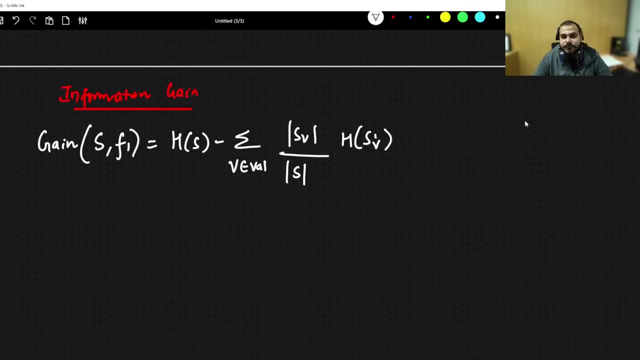 to values s of v. don't worry, guys, if you have not understood the formula, i will explain it. then the sample size h of sv. okay, now this is my thing. okay, i'll discuss about each and every parameter. okay, let's say that i'm taking this feature one split. i have. you have already seen what is feature one, so this is: 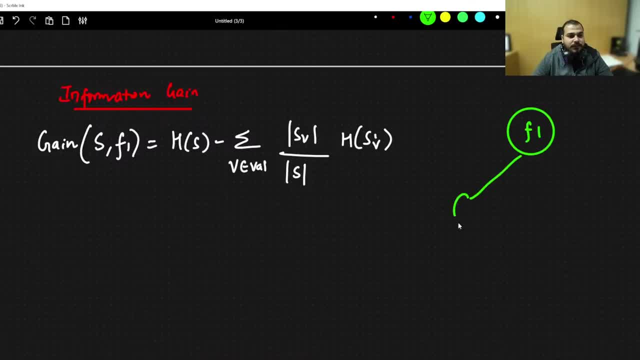 my feature one. okay, i have two categories: c1, c2. okay, this has nine yes, five no's, this has six yes and two no's, and this has three yes and three no's. okay, now i will try to calculate the information gain of this specific split. okay. 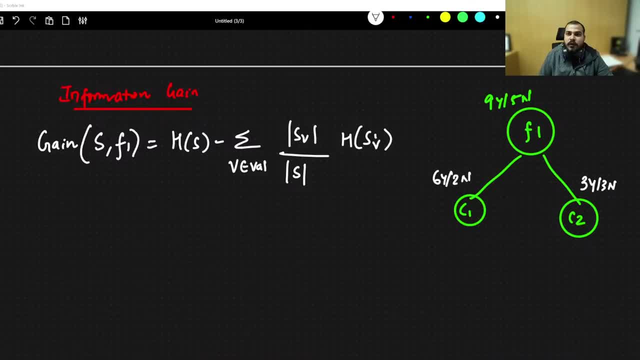 now i will go ahead and probably take this up now. see over here. we'll try to understand what is this. now. if i want to compute the gain of s of f1 first is first. first thing that i need to find out is h of s. now this h of s is specifically of the root node. so i need to first of all calculate what is. 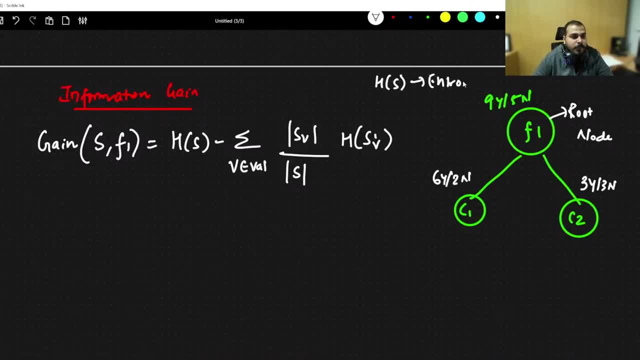 h of s. h of s is nothing but entropy, entropy of the root node. okay, So if I want to compute the entropy of the root node, tell me how should I compute. h of s is equal to minus p plus log base, 2 p plus calculate guys along with me- minus p. 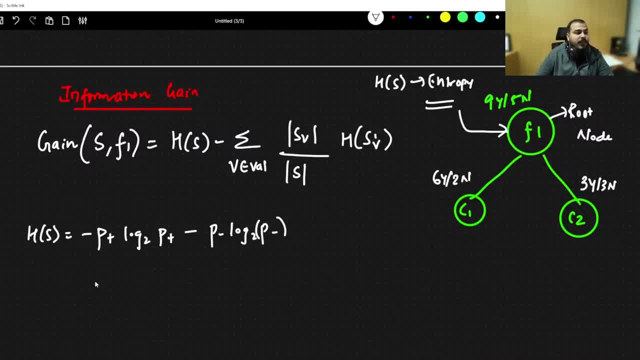 minus log base 2: p minus. So I hope everybody knows this. So here I am going to compute by what is probability of plus over here in this specific root node. It is nothing but 9 by 14.. Then I have log base 2, again 9 by 14.. 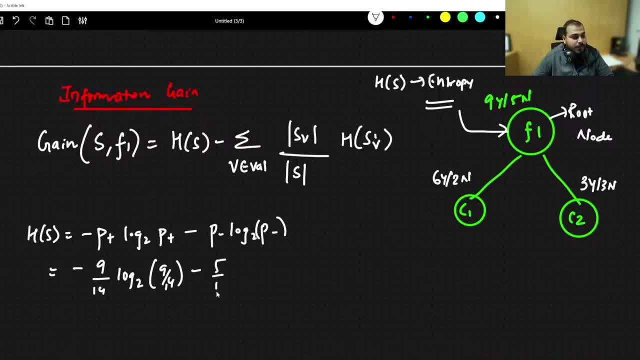 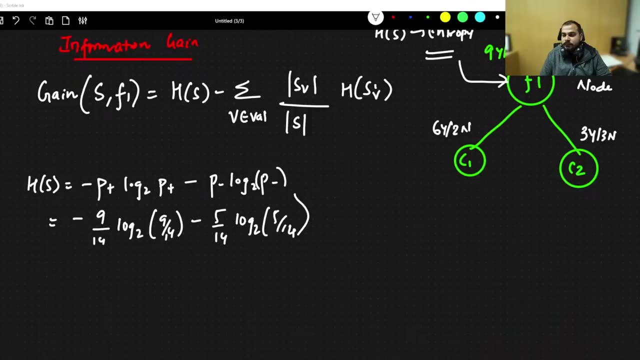 Then I have p minus. what is p minus? 5 by 14, log base 2, 5 by 14,, 5 by 14, right, I can definitely get this much. I hope everybody is understanding till here. Himanshu Shekhar, your entropy will always be between 0 to 1.. 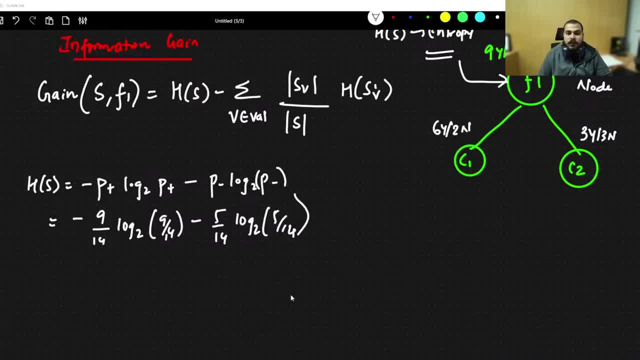 Okay, So here it is. You can see this. Now do the calculation. whatever calculation you are getting, Just let me know quickly. So this calculation, I will probably get it as 0.94. okay, approximately equal to 0.94.. Just check it whether you are getting this or not. 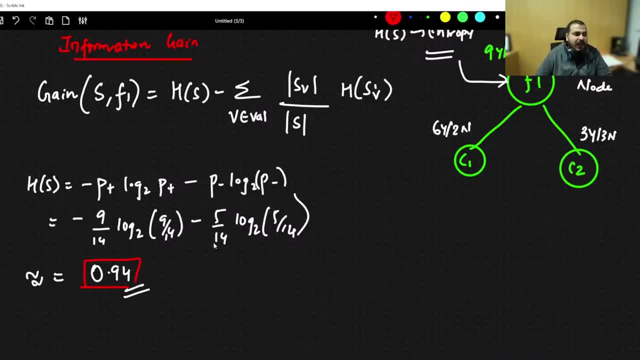 Again, you can use calculator if you want. Okay Now, Okay, So I am going to conclude about this. This is specifically for the root node. Now let's see the next thing, the next important thing, which is this part: What is S of V and what is S and what is H of S? V? 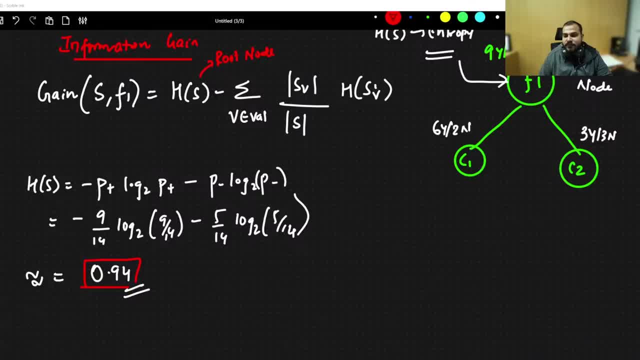 It is very, very simple, Okay, Very, very simple. I will discuss about it. Okay, now, very important. just have a look. okay, everybody see this graph. okay, see this graph. I will talk about H of SV first of all. I will talk about H of SV. okay, this. 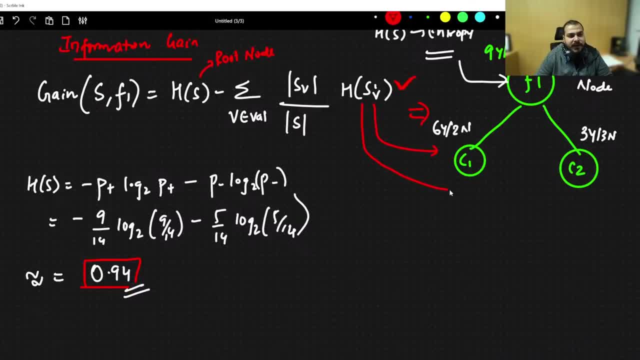 one. this is the entropy of category 1 you need to find and entropy of category 2 you need to find. so go ahead and find quickly. so if I write H of SV of category 1, so what is category 1 for this, I will write SC1,. let's say I am going to write like this: 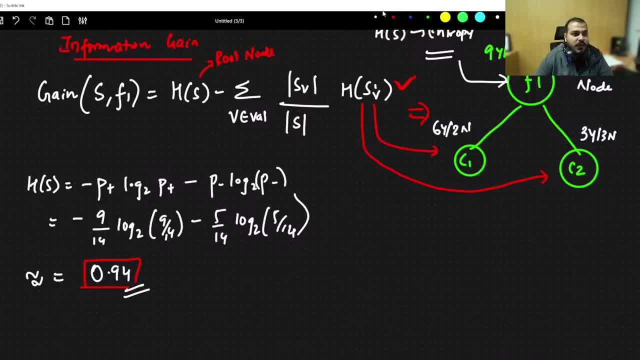 quickly calculate the H of SV of this. and this, okay, separately. you need to calculate so H of SV of C1, okay, so here again you will write: tell me minus 6 by 8, log base 2, 6 by 8. 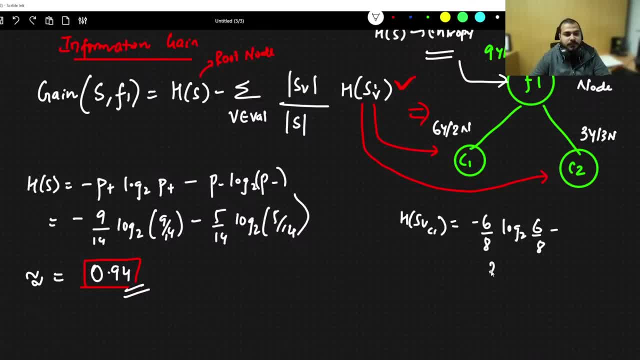 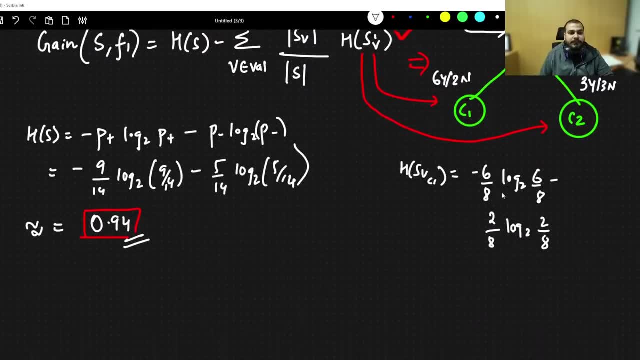 minus 2 by 8, log base 2, 2 by 8, I hope everybody knows this how we got it okay, so please write it down. I will try to write it down again for you so that your simplification. 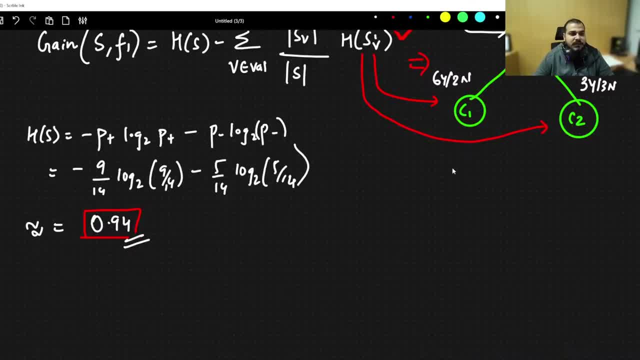 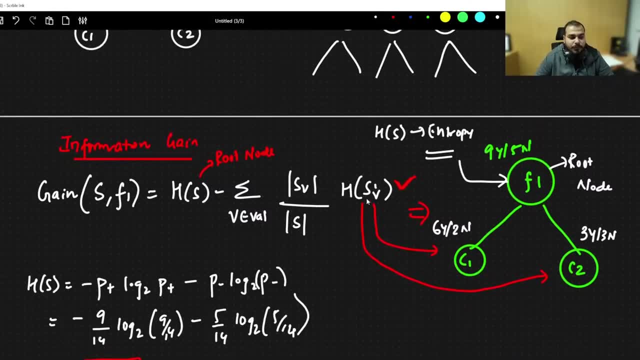 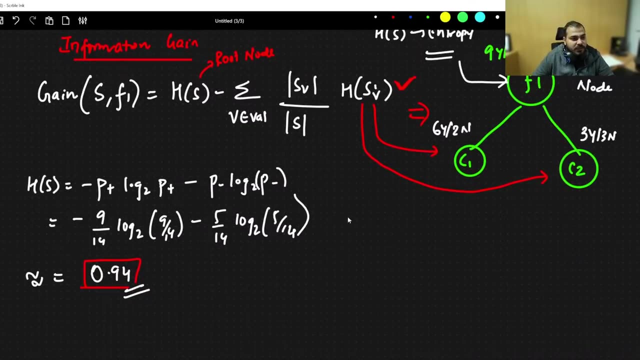 and again people will say: no, I did not understand. okay, so let's see this. okay, so H of SV basically means I am going to compute the entropy of this category And this category. okay, so for that I will basically write H of H of C1, so here I will. 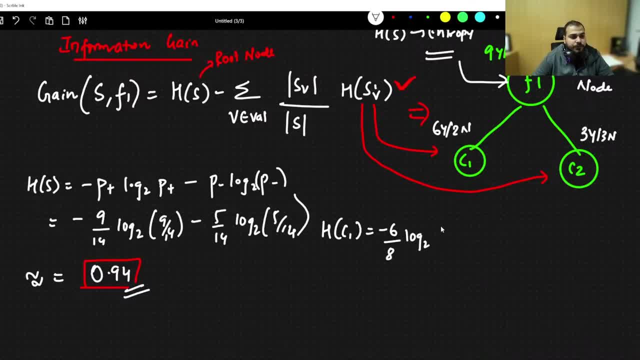 write: minus 6 by 8, log base 2, 6 by 8, minus 2 by 8 log base 2, 2 by 8, so if I get it, I am actually going to get 0.81, H of C1, okay, and similarly, if I calculate: 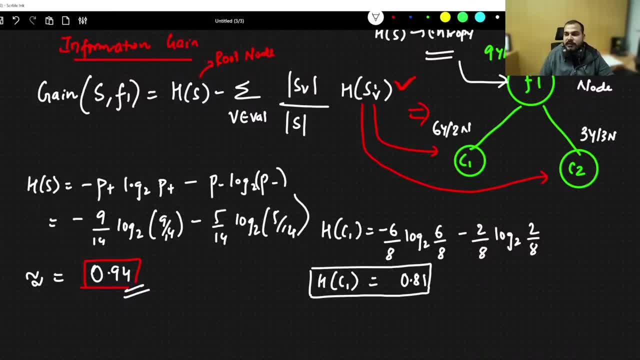 H of C2, quickly calculate how much you are going to get guys H of C2, how much you will get. see there are 3 yes and 3 no's. come on 6 by 8,, 6 by 8, with respect to this. 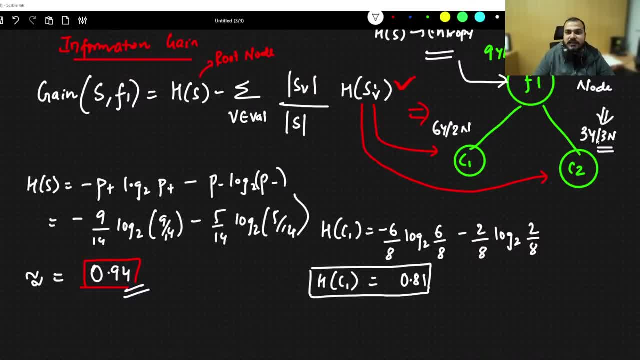 we need to find out how much we will get. come on, think over this common sense. common sense, come on, guys. what is the end result? Entropy for this H of C2, 1,. amazing, I like it okay. 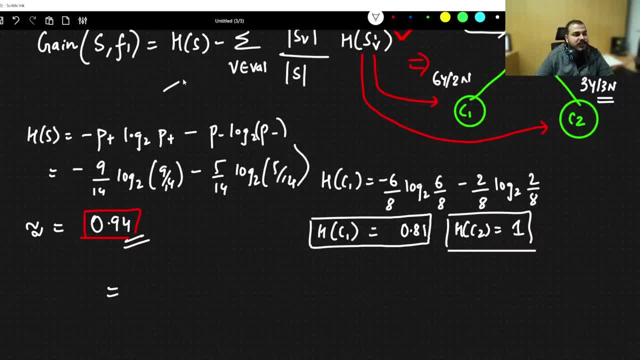 So now we have all these values, we will start equating them to this equation. okay, So here we have finally gain of S F1, okay, So let's say that here I am going to basically add 0.94 minus: see minus summation of okay. 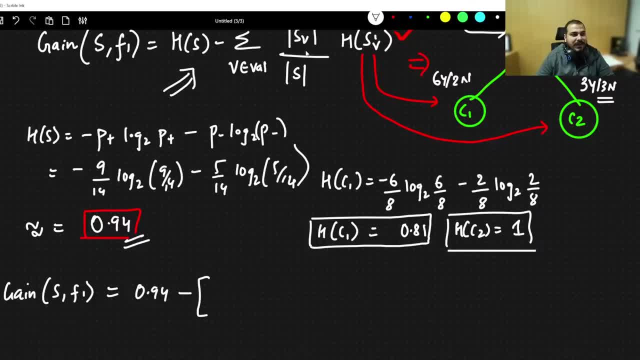 summation of what is S of V. understand. S of V basically means that how many samples I have over here, Let's say for category 1, how many samples I have for category 1 over here. simple, if you really want to just calculate, it is nothing but 8, and total number of sample is how much. 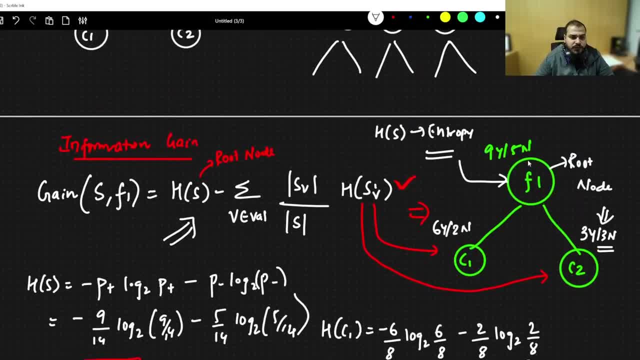 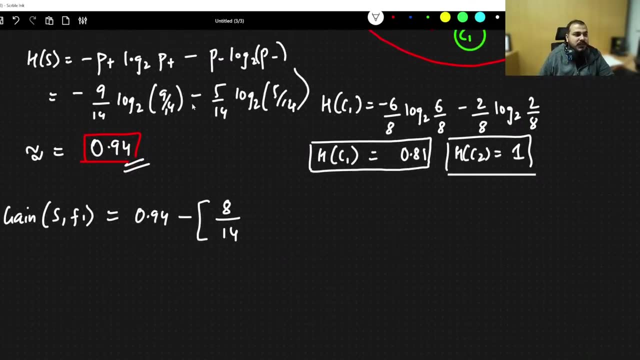 if I go and see over here, there are 9 yes, 5 no's okay, 9 yes and 5 no's. that basically means 14 total sample. Here you have 8 sample, okay. so this will become 8 by 14, then you multiply by what. 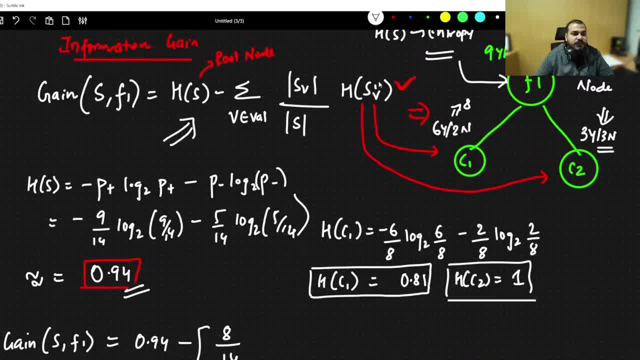 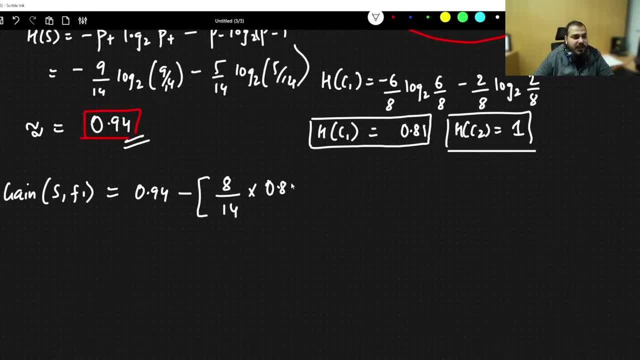 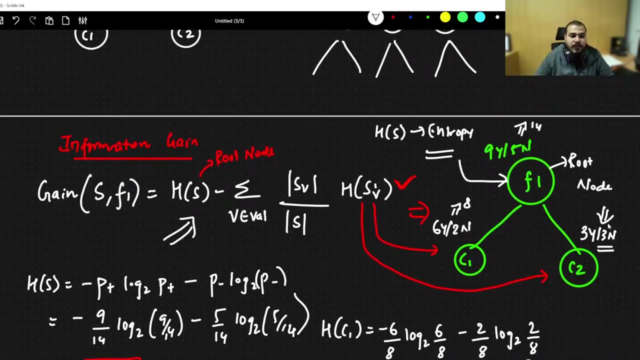 see from this equation: you multiply by H of S V, so H of S V is nothing but the entropy of category 1, so entropy of category 1 is nothing but 0.81 plus. then you go again back to the graph and try to see that for C2, how much, how many total number of samples are. 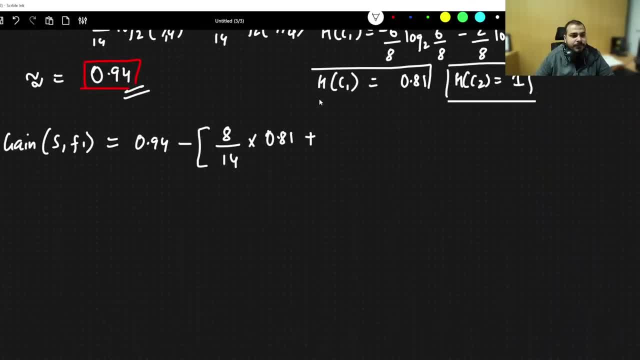 there 3 plus 3, 6.. 6 by 14, it will become multiplied by 1, right, so this is your entire thing. okay, this is your entire thing. Now, from this, do the calculation, try to find out what is the output. so here after: 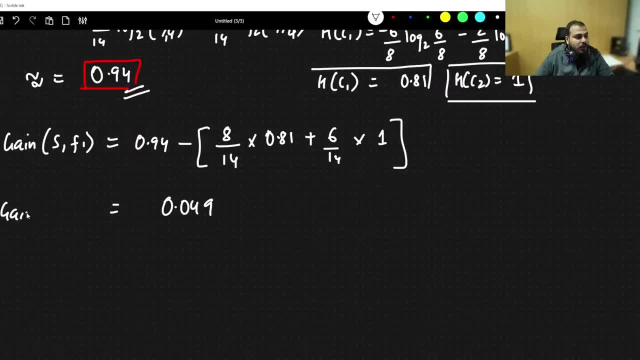 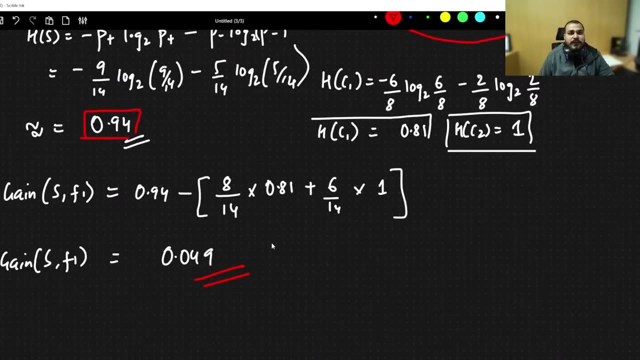 all the calculation, you are going to get 0.041.. So this is my gain with S F1,. okay, so here I have got this value. amazing, this is amazing. now, I did this with feature 1, only. what about feature 2,? let's say that this was my split. 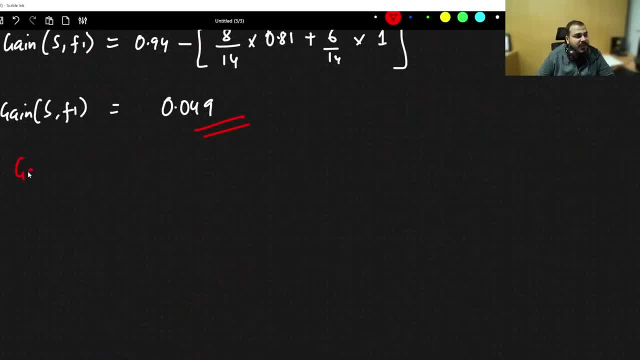 for feature 2 and suppose I get the gain for S feature 2 as 0.00051,. if I get this now, tell me In using which feature should I start splitting first? using which feature should I start splitting first? splitting first whether it should be F1 or whether it should be F2. 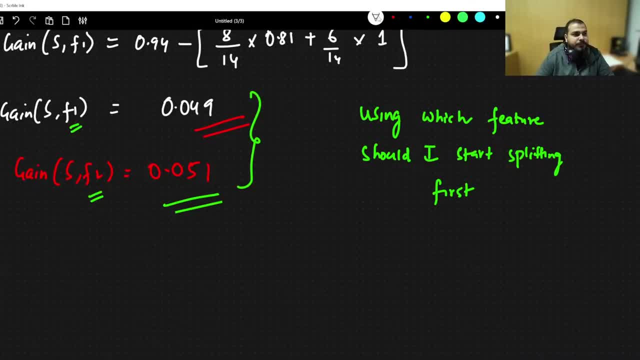 based on this value. you know that over here the gain, the information gain, of S F2 is greater than F1.. Gain of S F1,. so your answer is very much simple. we will definitely use feature 2 to. 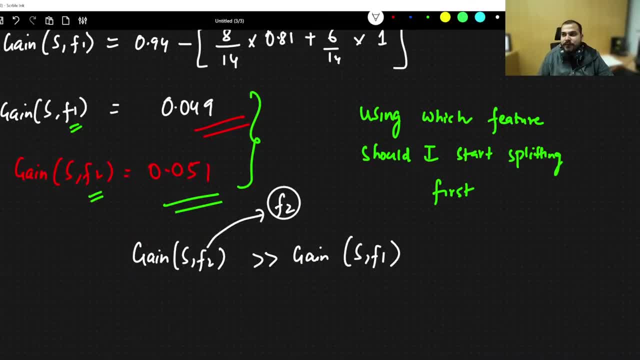 start the split. I hope everybody is clear from this. yeah, hit, like. I hope you are having fun, I hope you are having fun guys. so like it, make it 500 at least quickly. then only I will enjoy, I will get red bull. 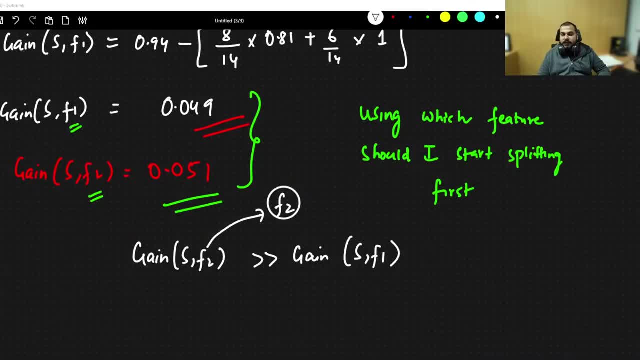 Right. So Understand one thing over here. okay. so the thing over here you are trying to understand: that if I really want to select which feature to select to start my splitting, then I have to basically calculate the information gain and go throughout the all the paths and whichever. 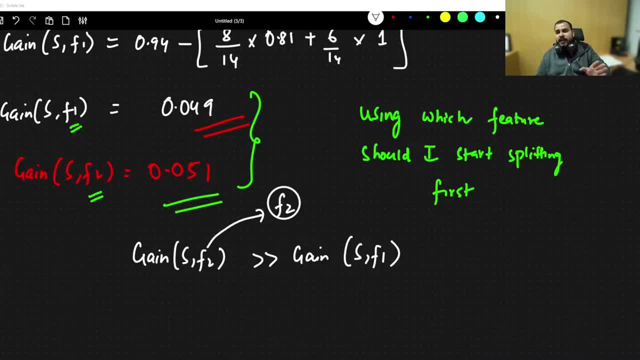 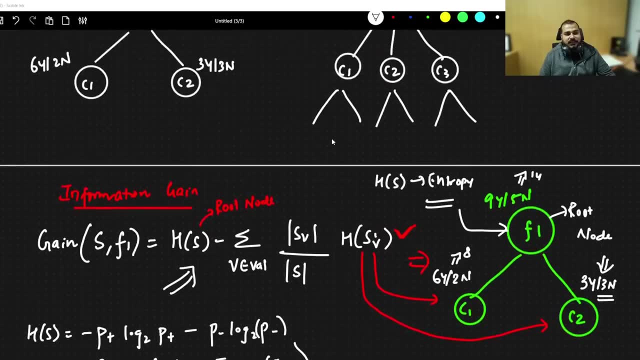 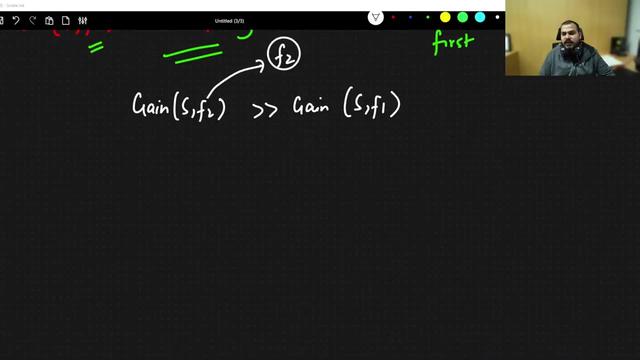 path has the highest information gain, then we will select that specifically. okay, very good. Now the question rises, Krish. obviously this is good, but you had written about Gini impurity. what is the purpose of that? please explain us and why Gini impurity is basically. 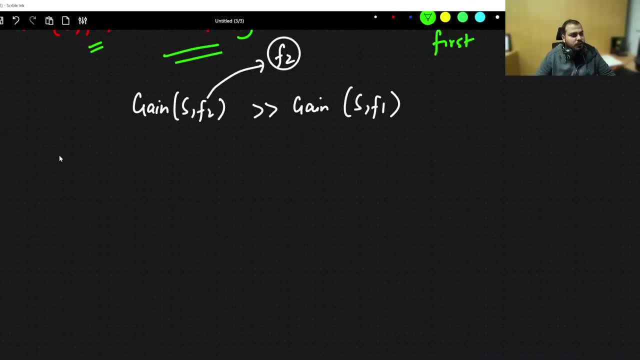 used. So let me go ahead with Gini impurity, the next topic. I told about that, sorry, Gini impurity. I told that, yes, you can obviously use, you can obviously use entropy, but why Gini impurity? 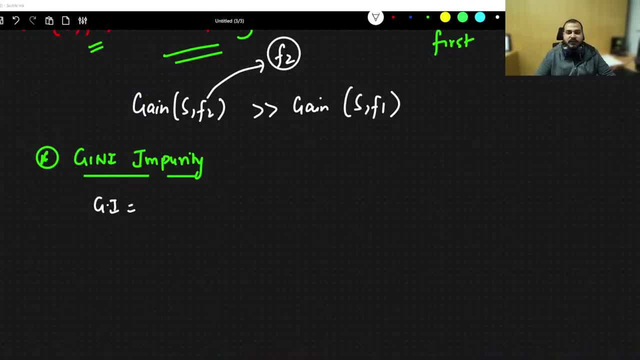 So Gini impurity formula, Which I have specifically written as one minus summation of I, is equal to 1 to n P squared. Now, what is this P squared? What is this P squared? Okay, So this P squared. you really need to understand. 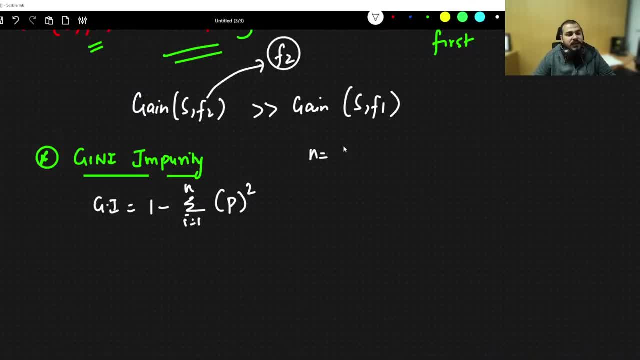 Okay, Suppose let's say that in my n n is the number of outputs right now how many outputs I have. I have two outputs, yes or no? Okay, So I will expand this one minus. since this is summation, I is equal to 1 minus summation. 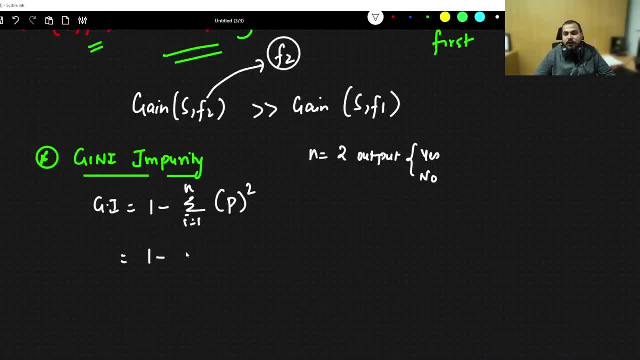 1 minus summation of i is equal to 2.. Okay, to 1 to n. I am basically going to basically say that: ok, fine, I will write probability of plus whole square plus probability of minus whole square. so this is the formula for guinea. 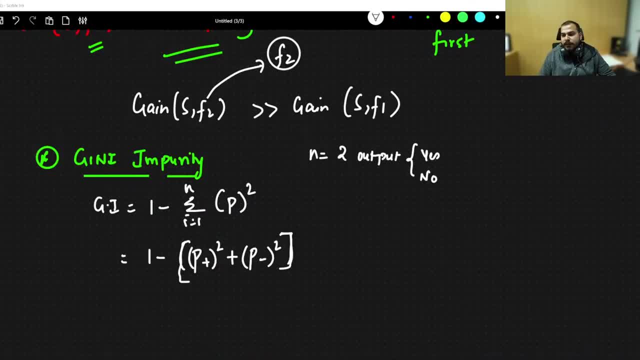 impurity. ok, now you may be thinking: ok, fine, the calculation will be obviously very much equal. easy, right, suppose, if I have a node, sorry, if I have a node which has two yes, two no's. now, in this particular case, how do I calculate my this probability? ok, if I have 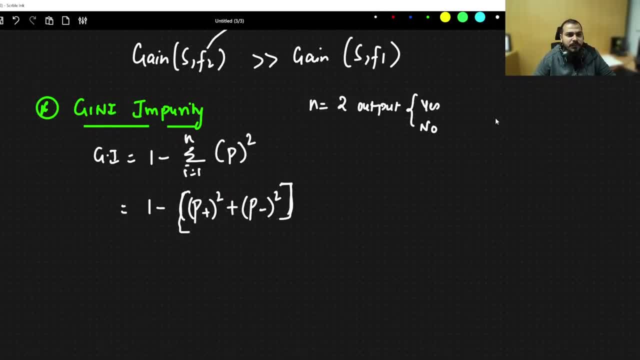 two yes or two no's, suppose let's say that I have a node over here which is my split. ok, and this is having two yes and two no's. so how do I calculate? I will write one minus what is probability of square one by two. square, sorry, not one by two. 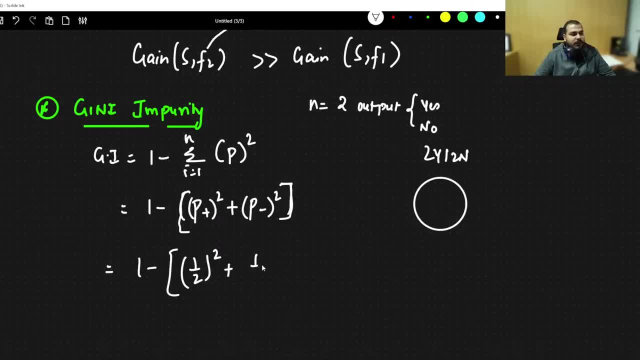 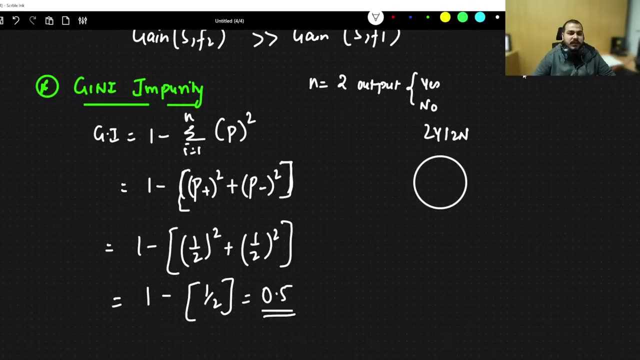 yeah, one by two square plus one by two square. right, then I will say: one by one by four plus one by four is nothing but two by four, which is nothing but one by two. so I will be getting point five now here. you understand, this is a complete impure split, right, if you have? 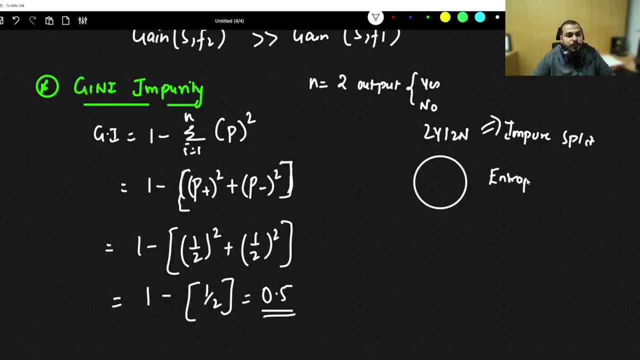 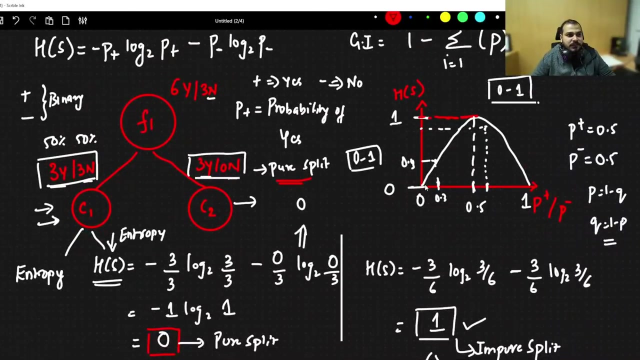 an impure split. in entropy, the output, you are getting it as one right, whereas in the case of guinea impurity, guinea impurity- you are getting how much as zero. sorry point five. so if I go ahead with the graph that I probably had created here, so my guinea impurity line will 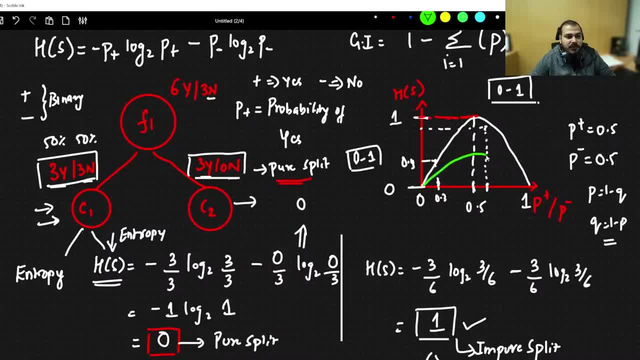 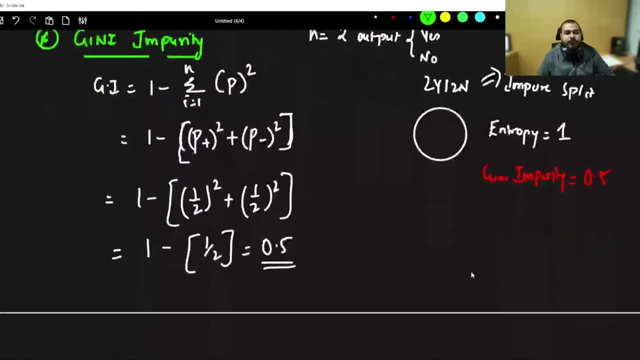 look something like this. so it will be looking something like this for zero. obviously I will be getting zero, but whenever my probability of plus is point five, I am going to get point five over here, and that is the difference between guinea impurity and entropy. but the re, but you may. 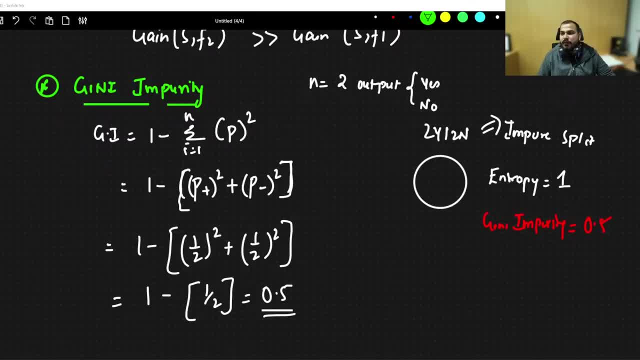 be seeing krish. when to use what? ok. when to use: ok, it's ok, sanjay, you can say guinea impurity. you can say guinea index. you can say guinea coefficient- anything you can, ok, not a issue, now, let's understand that. when to use: 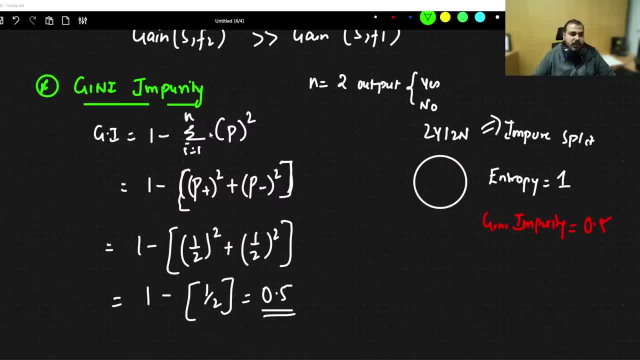 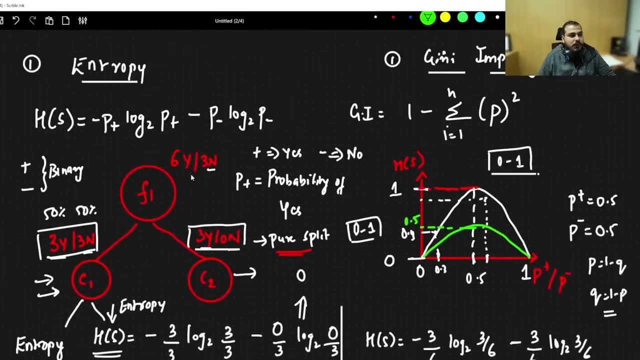 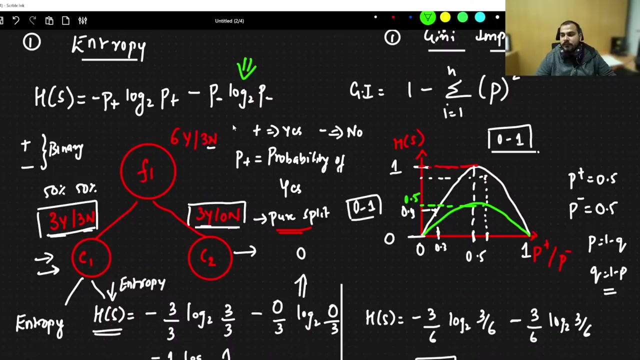 when to use guinea and when to use entropy. tell me, guys, if I consider this formula ok, if I consider this formula of guinea impurity and if I probably consider, if I consider entropy, this formula, where do you think more time will take for execution for this particular? 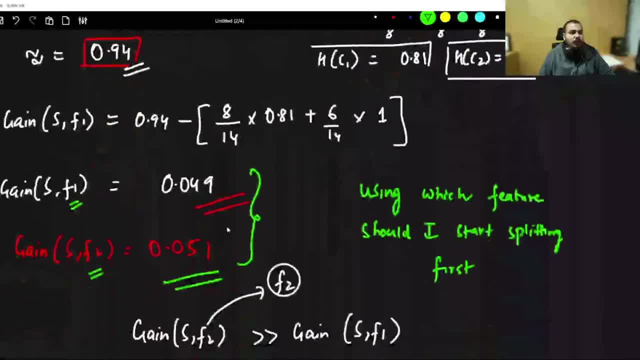 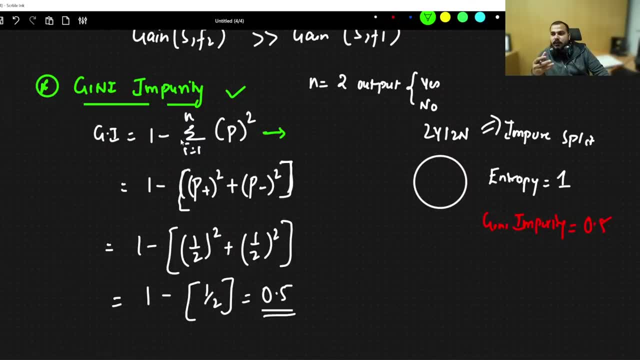 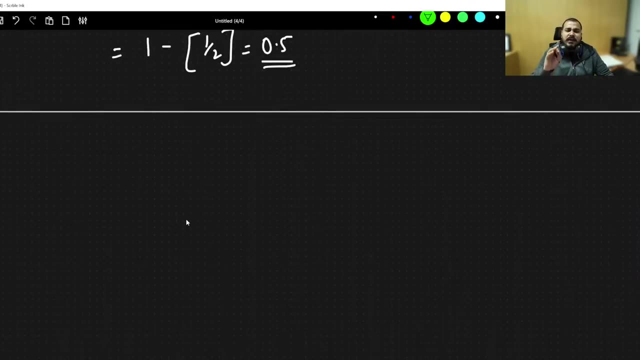 formula, whether for entropy it will take or for guinea impurity it will take more time. where it will probably take for the execution purpose to understand decision tree is having a worst time: complexity, because if you have hundred features probably you'll keep on comparing by dividing many, many features. then probably compute information again like this if you have. 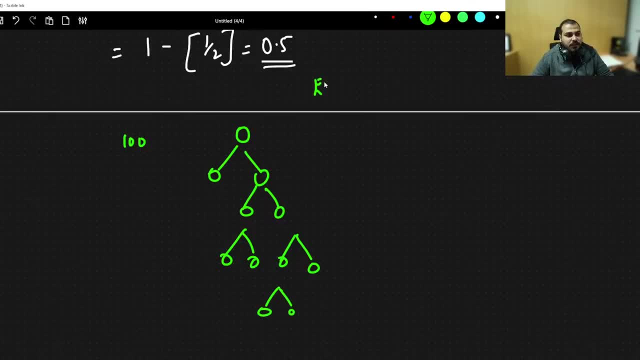 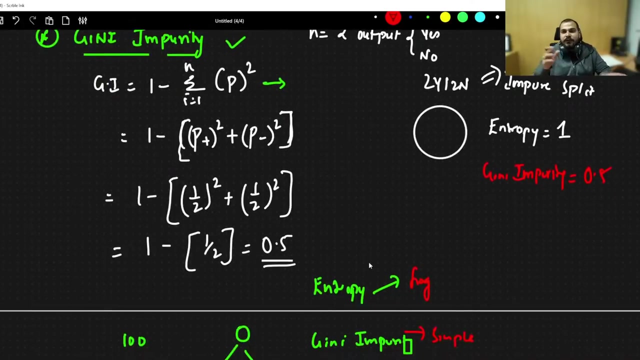 just hundred features, right? so which is faster, entropy or guinea impurity? understand, in entropy you have log function. here you have log function. here you have simple maths. so the more amount of time out of entropy and guinea impurity, the more amount of time basically is taken by entropy. so if you have huge number of features like hundred, 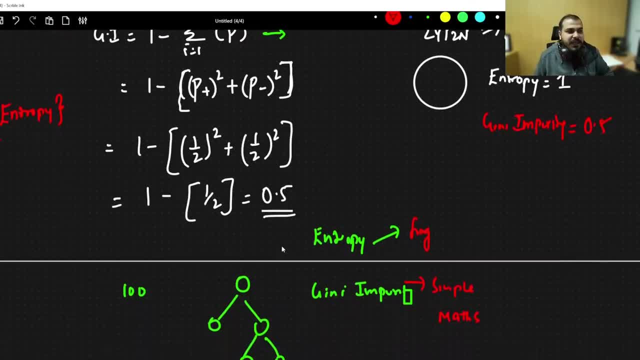 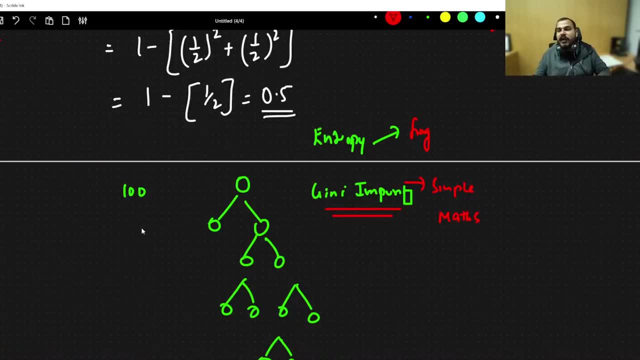 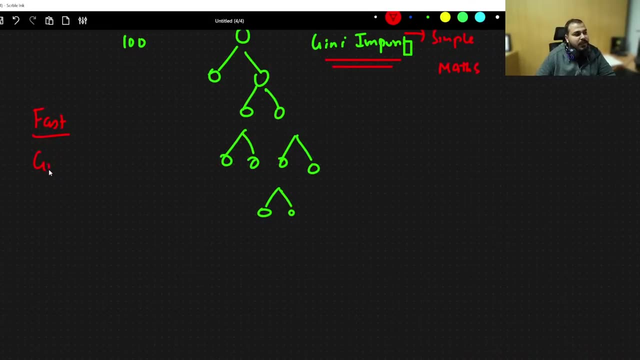 two hundred features and you are planning to apply decision tree, i would suggest try to use guinea impurity, then entropy. if you have small set of features, then you can go ahead with entropy. okay, so over here, definitely with respect to fast, guinea is greater than. 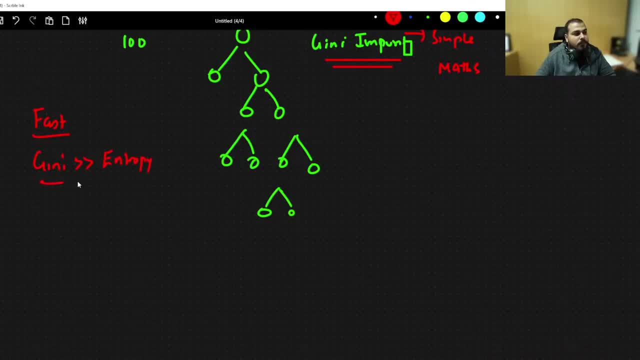 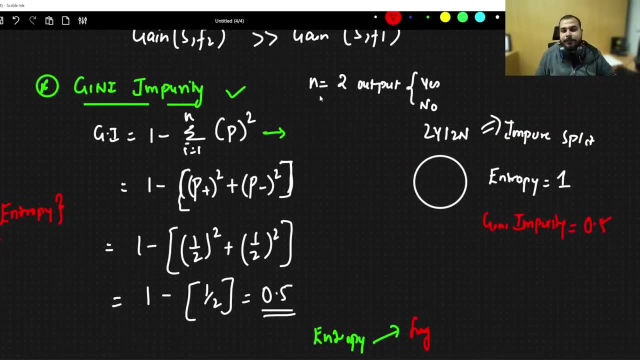 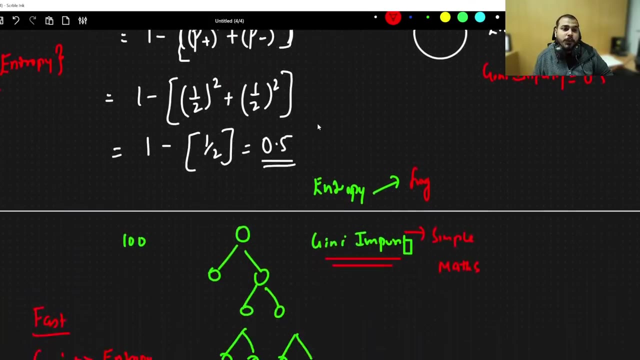 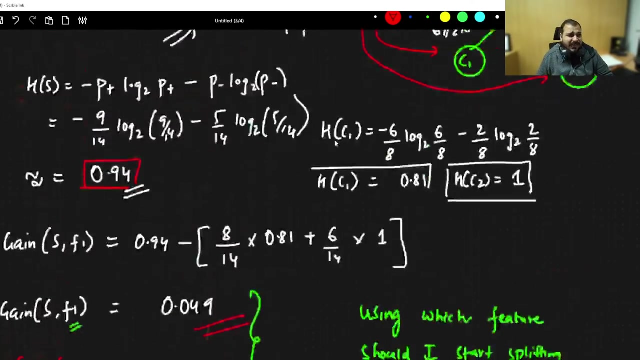 entropy. good, i hope everybody is able to understand. okay, now let's go ahead and understand with respect to, with respect to. you may be thinking krish, okay, fine, you have basically explained us about categorical variables over here. see, over here you have explained about categorical variables. what if i have? 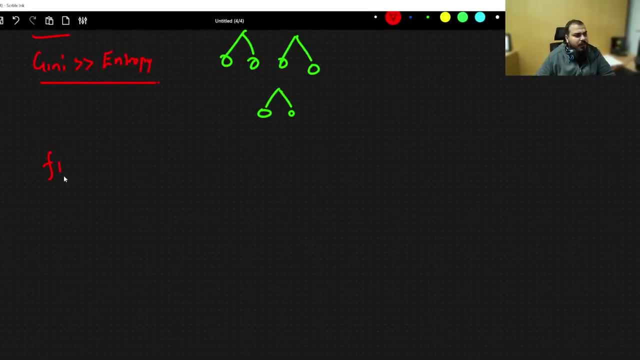 numerical features. let's say i have f1 over here, which is a numerical feature, i have an f1 feature, which is numerical feature, and i may have values. let's say that i have sorted all the values over here. okay, what is the advantage of entropy over guinea? 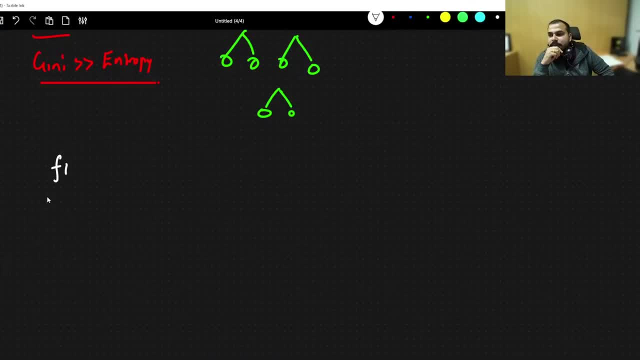 guinea is fast. entropy is slow. entropy should be used when less number of features are there. guinea should be used when huge number of features are there. very simple, okay. okay, let's say that i have f1 and output. okay. so this f1, let's say that i have values like 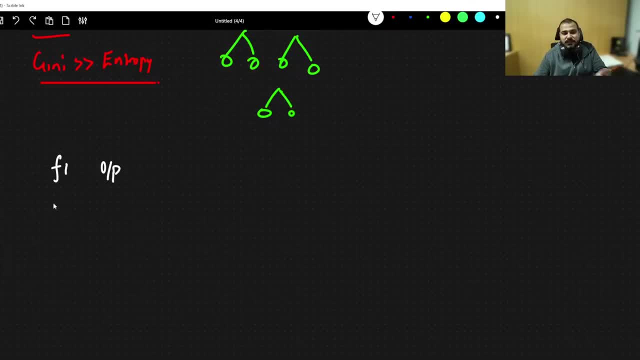 a sorted order values. i'm sorting these features. i'm basically doing this. let's say that initially i have these features like this: okay, and let's say i have values like 2.3, 1.3, 4, 5, 7, 3- okay, let's. 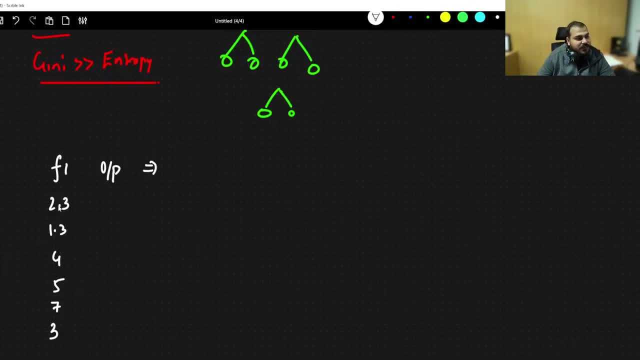 say, i have these features. okay, now, this is a continuous feature. this is a continuous feature. so for a continuous feature, how probably the decision tree entropy will be calculated and the information gain will get calculated. okay, so here you will be able to see that i will first of all sort these values. so in f1 the decision tree will basically first of all. 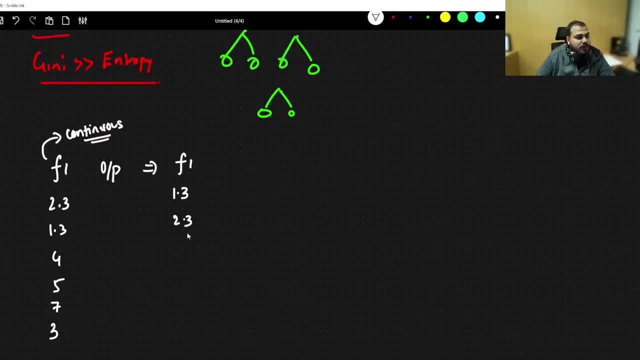 sort this value. so i have 1.3, then you have 2.3, then you have 4, then you have 4, then you have 3, 3, then you have 4, then you have 5 and then you have 6. okay, now, whenever you, 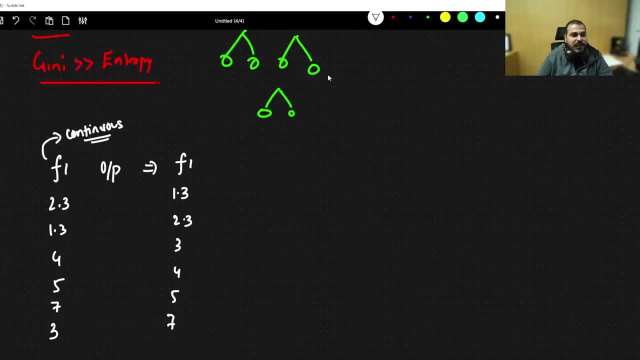 have a continuous feature. so how the continuous feature will basically work in this case. first of all, your decision tree node will say that we'll take this one, only one first record and say that if it is less than or equal to 1.3, okay, if it is less than or equal to 1.3. 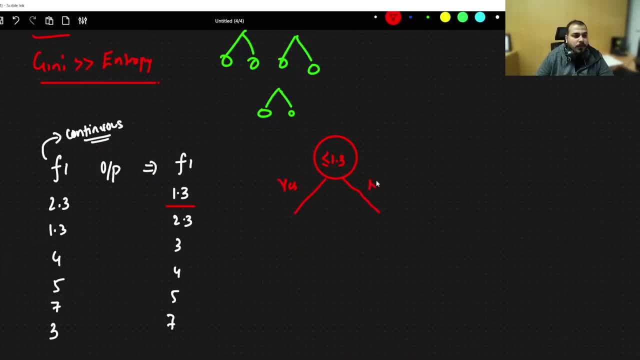 so here you will be getting two branches, yes or no. so yes and no, definitely your output over here will be put over here, right, and then for the no, here you will be having another node over here: how many number of records you'll be having in this particular case you will be having one record in this. 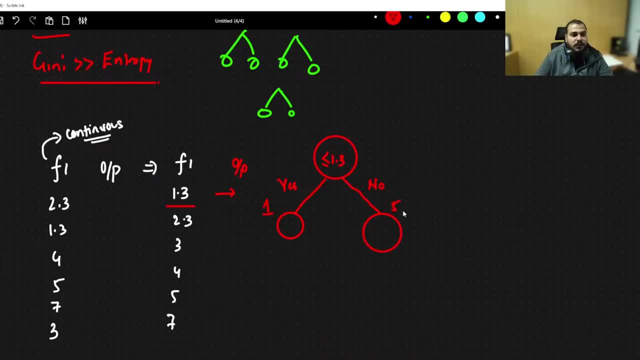 particular case, you will be having around five to six records and here also you'll be able to see right how many yes and no's are there. definitely this will be a leaf node, right? so in the first instance, so in this instance, they will go ahead and calculate the information. 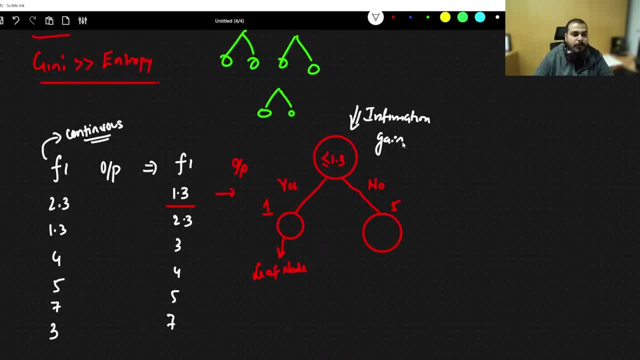 gain of this. okay, then probably, once the information gain is got, then what they'll do? they will take the first two records and again create a new decision tree. let's say that this will be my suggestion- where they'll say it is less than or equal to 2.3, so I will get 1 and 1 over here. so in this now you'll be having. 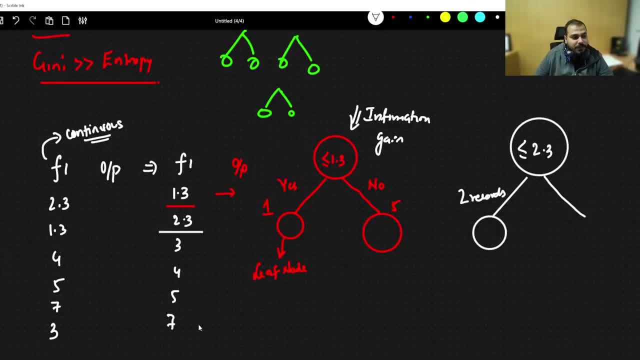 two records, which will be one and one over here. so now I will get two records and I'll basically say how many yes and no are there, and remaining all records will come over here. then again, information gain will be computed here. information gain will be computed then. 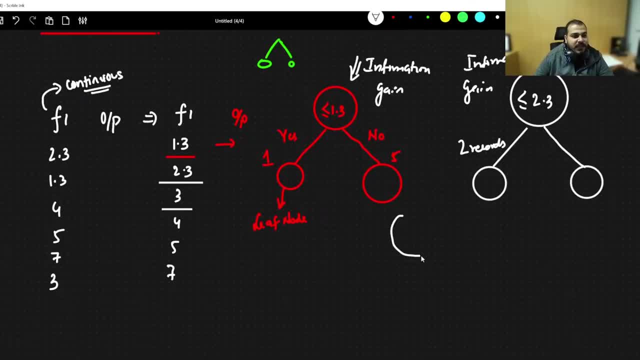 again. what will happen? they will go to the next record. then again they will create another feature where they will say less than or equal to 3, and they will create this many nodes again. they will try to understand how many yes or no are there, and then they will again. 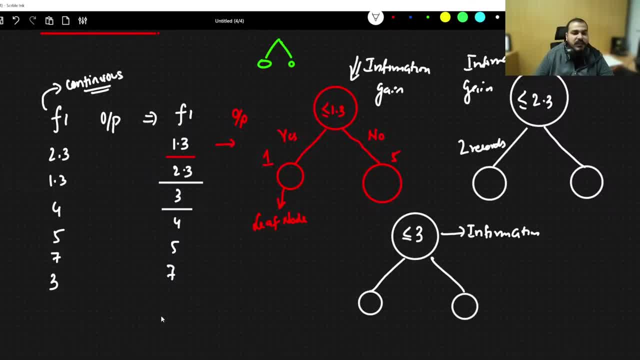 compute the information gain like this: they will do it for each and every record and, finally, whichever information gain is higher, they will select that specific value in that feature and they will split the node. I hope everybody is able to understand now. yes, so in a continuous feature. whenever you have a continuous feature, this is how it will basically have, ok, and 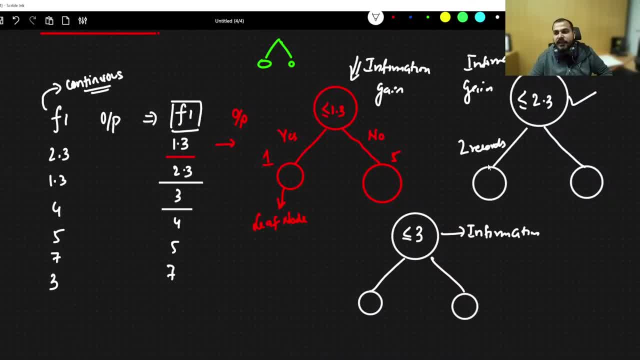 then it will try to compute who is having the highest information gain and who is having information gain right. the best information gain will get selected and from there the splitting will happen. best information gain. now let's go ahead and understand. now let's go ahead and understand about the next topic. is that how this? entirely? 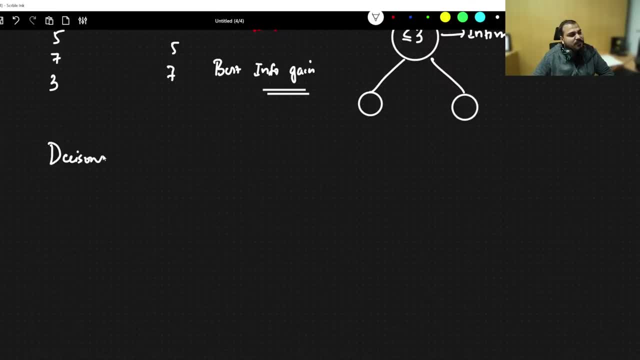 things work in decision tree regressor because in decision tree regressor my output is an continuous variable. so suppose if I have one feature one, feature two and this output is a continuous feature, it will be continuous. any value can be there. so in this particular case, how do I split it right? 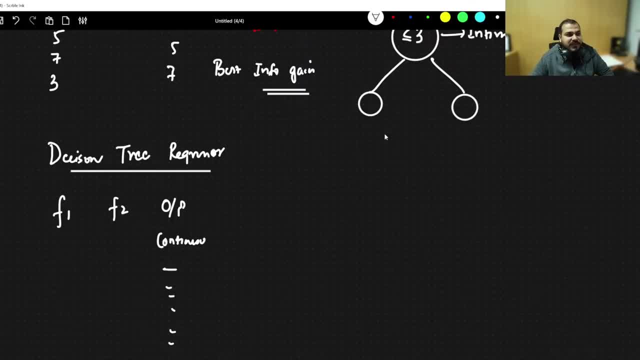 how do I split it right? so let's say that f1c feature is getting selected now in this particular case, how do I split it right? so let's say that f1c feature is getting selected now. in this f1c feature, what value will come when it is getting selected? okay, first of 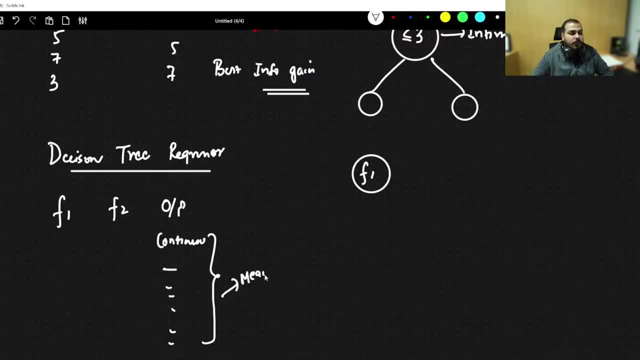 all the entire mean will get calculated of the output. okay, mean will get calculated. so here I will have the mean, and here the cost function that is used is not Gini coefficient or Gini impurity or entropy. here we use mean squared error, or you can also use mean absolute error. now 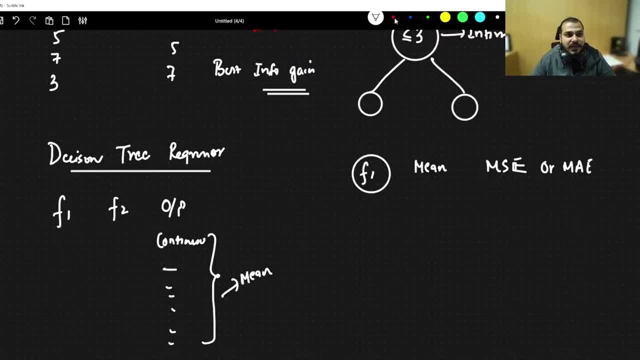 what is mean squared error? what is mean squared error? if you remember from our logistic linear regression, how do we calculate 1 by 2? M summation of i is equal to 1 to n. y hat minus y whole square right. y hat of i. y minus y whole square. this is what is. 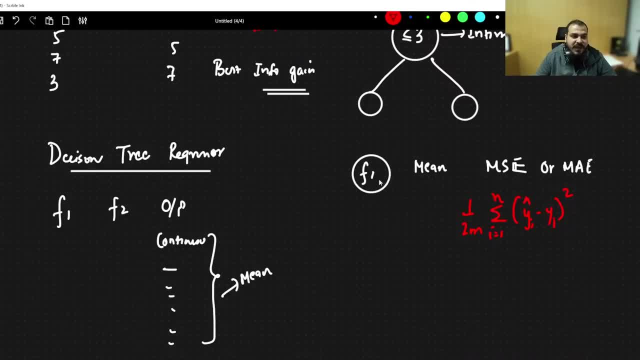 mean squared error. so what it will do: first, based on f1 feature, it will try to assign a mean value and then it will compute the MSC value, okay, and then it will go ahead and do the splitting. now, when it is doing splitting based on categories of continuous variable, i will be having different. 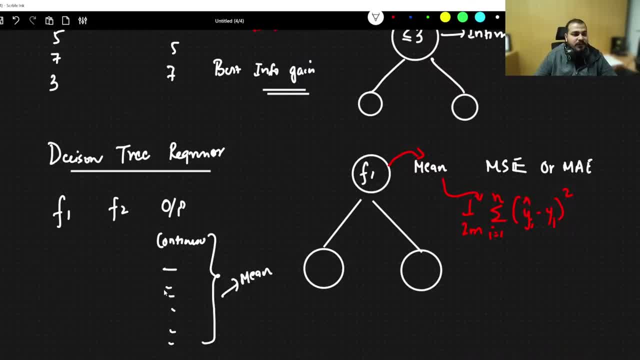 different categories. now in this categories, what will happen after split? some records will go over here. then I will be having a mean value of this over here. that will be my output. okay, that will be my output. and then again the MSC will get calculated, calculated over here As the MSE gets reduced. that basically means we are reaching near. 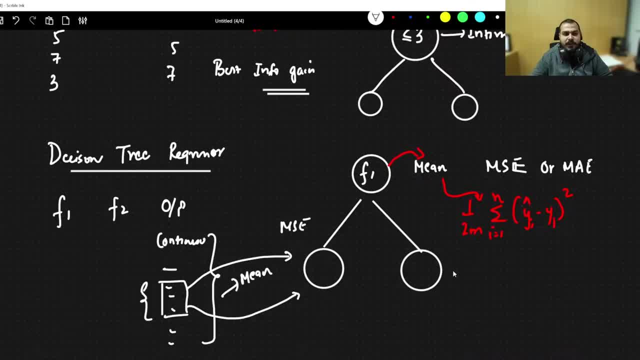 the leaf node And the same thing will happen over here. So, finally, when you follow this path, whatever mean value is present over here, that will be your output. I hope everybody is able to understand this specific thing. Okay, This is the difference between the decision. 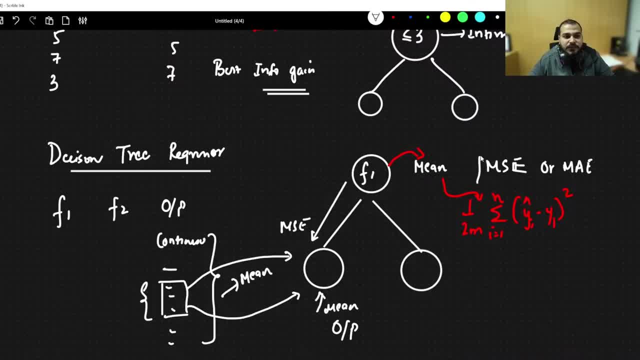 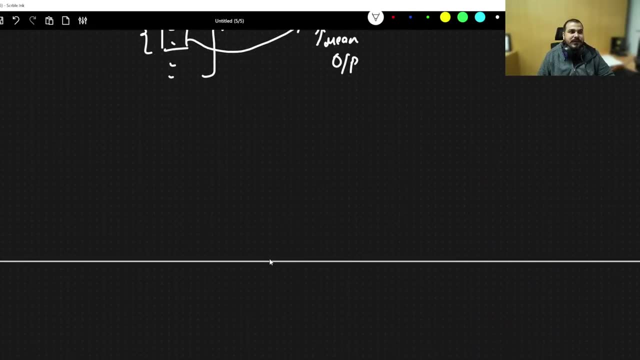 tree regressor and the classifier Here, instead of using entropy and all, you use mean squared error or mean absolute error, And this is the formula of mean squared error. Okay, Now let's go to the one more topic, which is called as the hyperparameters. 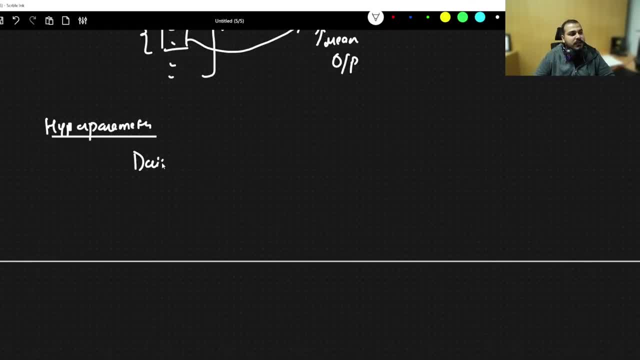 Tell me decision tree: if I keep on growing this to any depth, what kind of problem it will face? Regressor part: you want me to explain? Okay, let's see. Okay, let's do the regression Decision tree. regressor: Let's say: I have feature F1, and this is my output. 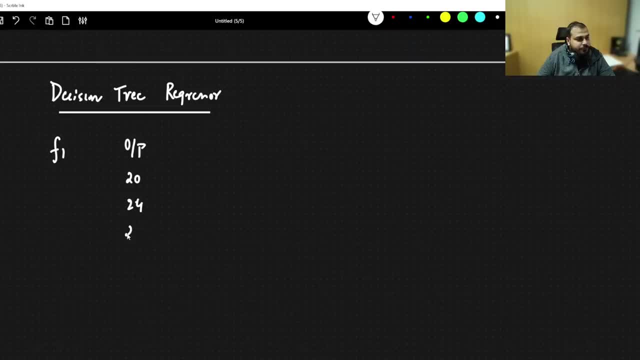 Let's say I have values like 20,, 24,, 26,, 28,, 30. And this is my feature one with category one. category one, let's say Some categories are there. Let's say I have done the division. 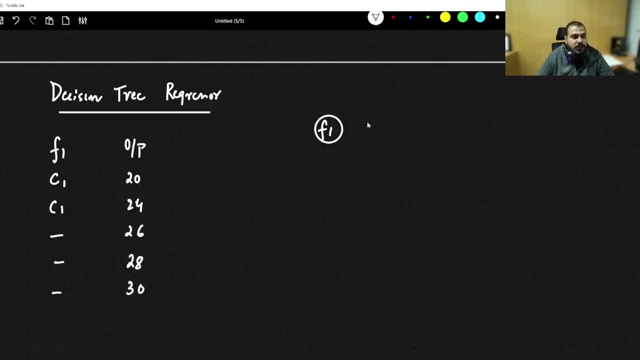 by F1.. That is this feature. Initially, tell me what is the mean of this, What is the mean of this, What is the mean of this? That mean value will get assigned over here. Then, using MSC, that is mean squared error. here you will try to calculate. Suppose I get an MSC of. 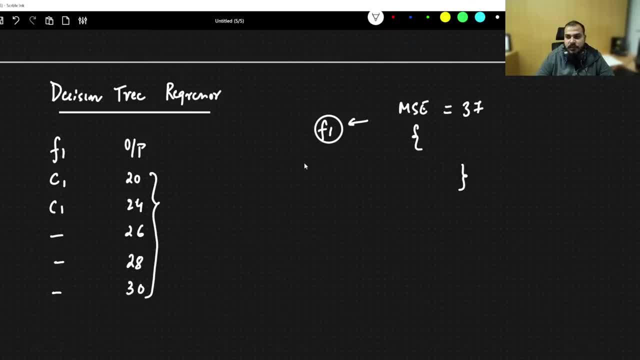 some 37,, 47,, something like this, And then I will try to split this. Then I will be getting two more nodes or three more nodes, It depends. Then that specific nodes will be the part of this. Again, the mean will change. Okay. 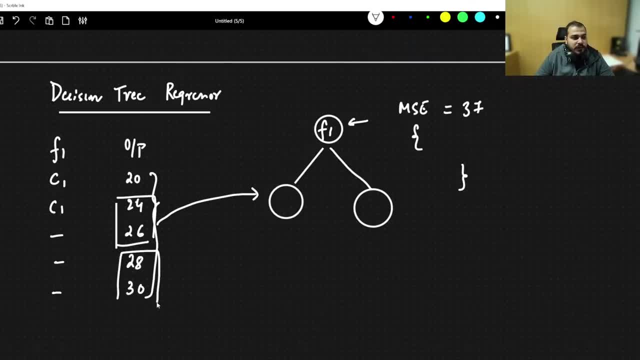 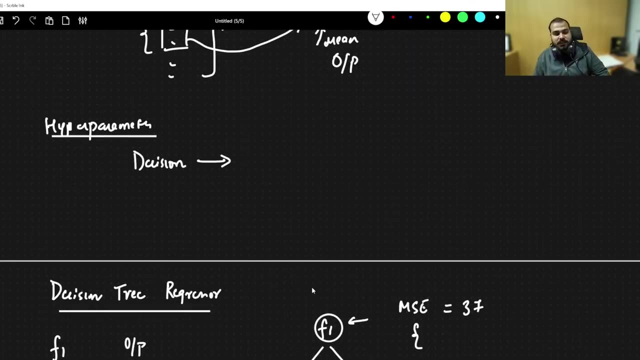 Again, the mean will change over here. Suppose this two is there, This two records go here Right, Then again MSC will get calculated. Okay, I'm just taking as an example over here. Okay, Just try to assume this thing. Okay, Now, if I talk about hyperparameter, See, 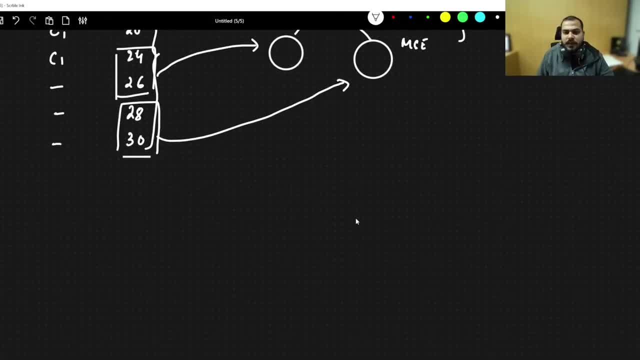 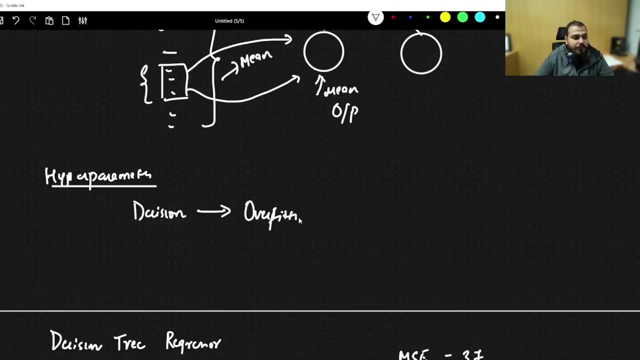 this is what is the formula that gets applied over here: MSC. Okay, Now let's see in this: always understand: decision tree leads to overfitting because we are just going to divide the nodes to whatever level we want, okay, so this obviously will lead to overfitting. 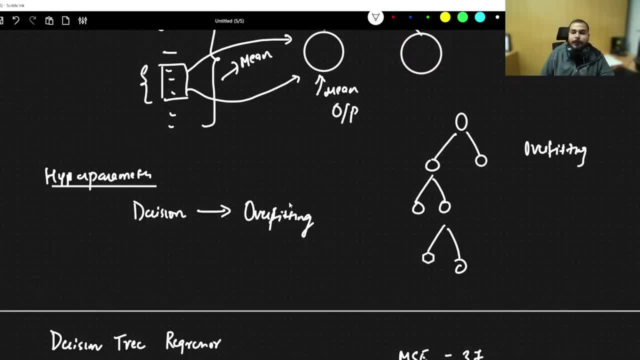 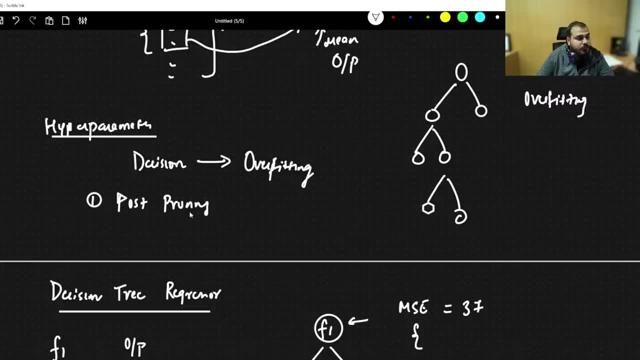 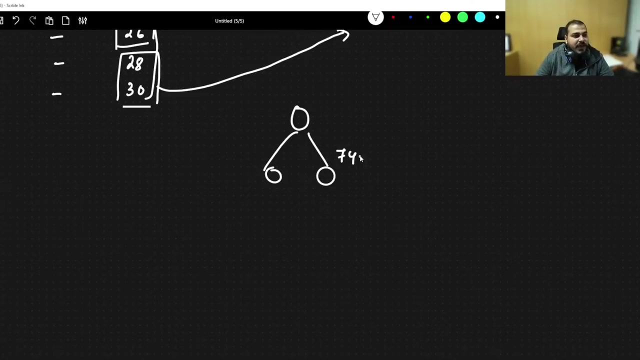 now, in order to prevent overfitting, we perform two important steps: one is post pruning and one is pre-pruning. so this two post pruning and pre-pruning is a condition. let's say that i have done some splits. i have done some splits. let's say, over here i have seven yes and two no. 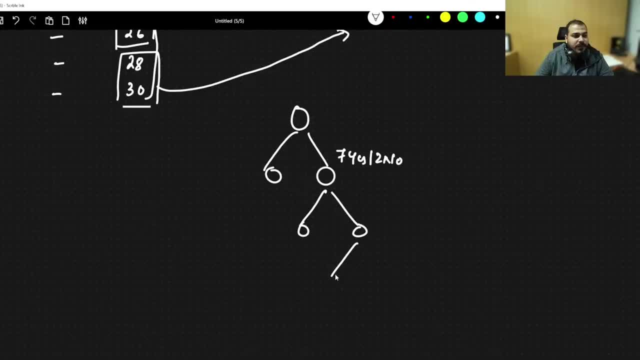 and again probably, i do the further split like this now, in this particular scenario, you know that if seven yes and two no's are there, there is a maximum. there is more than 80 percent chances that this node is saying that the output is yes. so should we further do this? 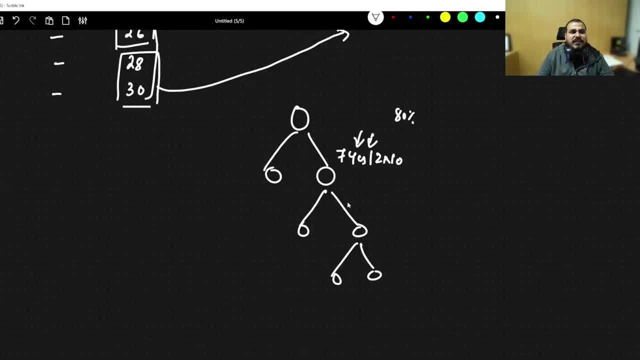 further, do more pruning? the answer is no. we can close it and we can cut the branch from here. okay, this technique is basically called as post pruning. that basically means, first of all, you create your decision tree, then probably see the decision tree and see that, whether there is an extra branch or not, and just try to cut it. there is one more thing. 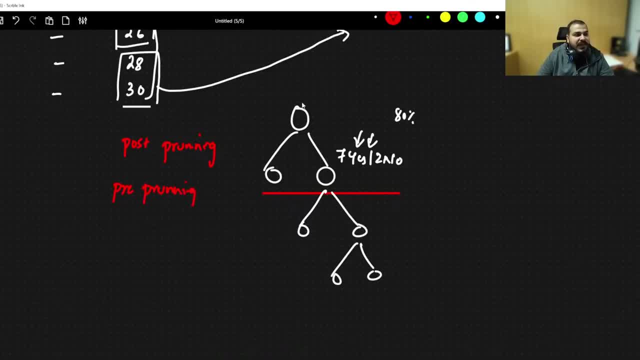 which is called as pre-pruning. now, pre-pruning is decided by hyper parameters. what kind of hyper parameters? you can basically say that how many number of decision tree needs to be used, not number of decision tree, sorry over here. you may say that what is the max depth? 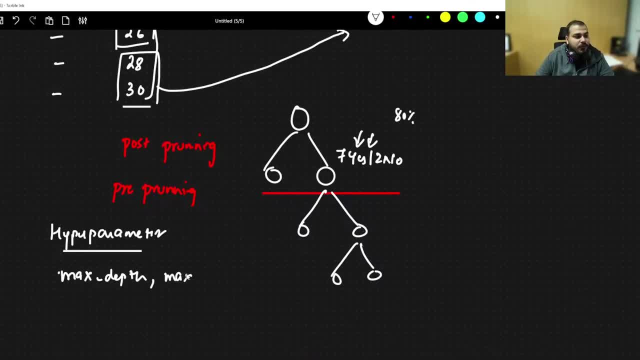 what is the max depth, how many max leaf you can have. so this all parameters. you can set it with grid search, cv and you can try it, and you can basically come up with a pre-pruning technique, arУqVths, unfolding time for your trend, and all these parameters which I will be. 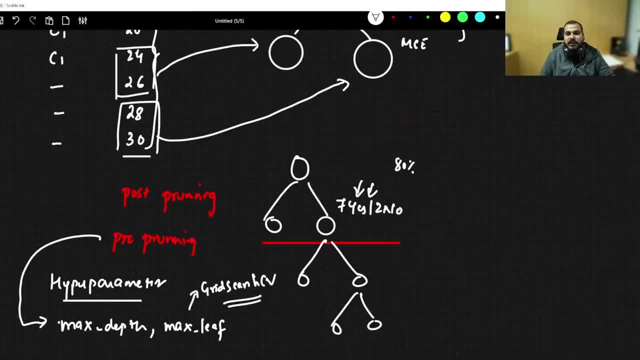 showing for you is data montage and I hope everybody's able to understand right? so this is the idea about decision tree regressor, and what I will also do is that I will show you one practical example. do you want to see one practical example? everyone, just tell me. 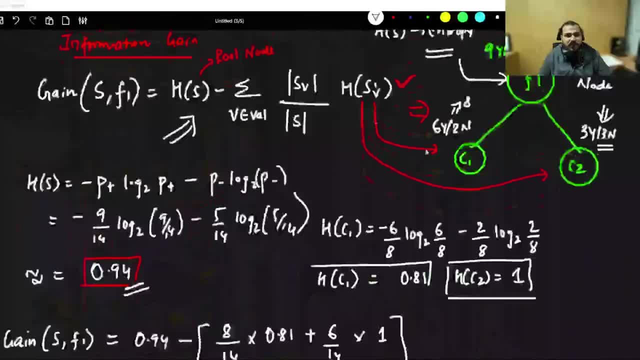 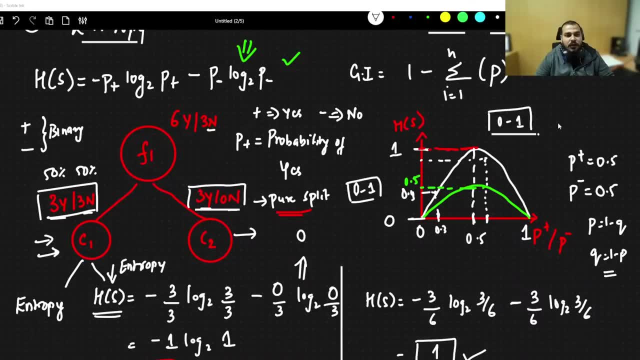 we're probably will also show you post pruning technique. just let me know. but till here, have you understood or not? yes, it is possible. your Gini value will be one. this graph is there. entropy: it will not be 1,. it will always be between 0 to 0.5,. Muhammad Aki Patel. ok. 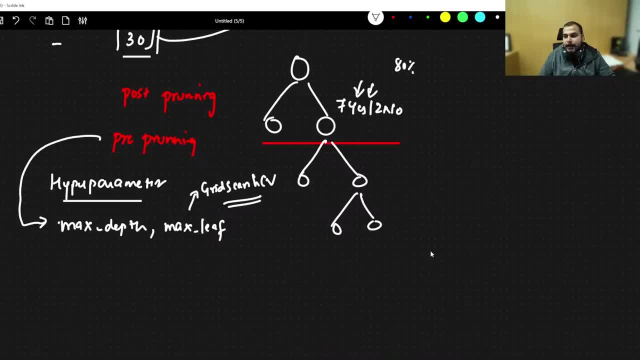 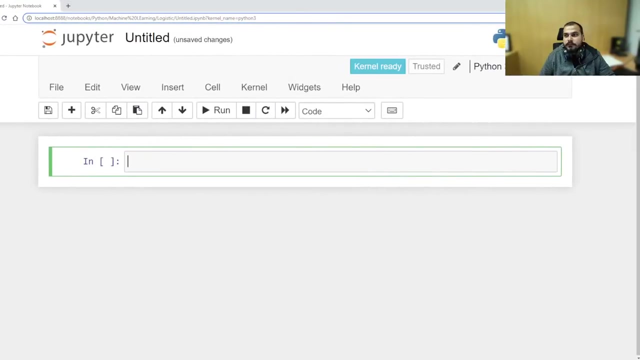 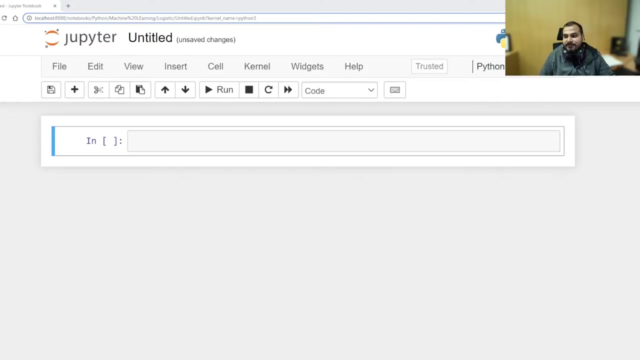 but I hope everybody understood. ok, now let's go ahead and let's try to solve a problem. so the first thing. first, As usual, what we should do. tell me we should import the libraries. so here I will go ahead and import the libraries. so I will say: import pandas as np. this is fun, right, if I do it. 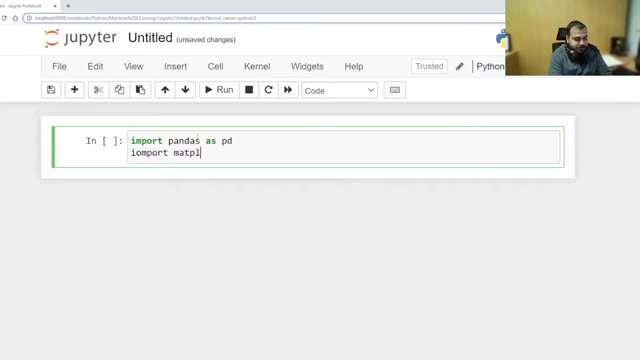 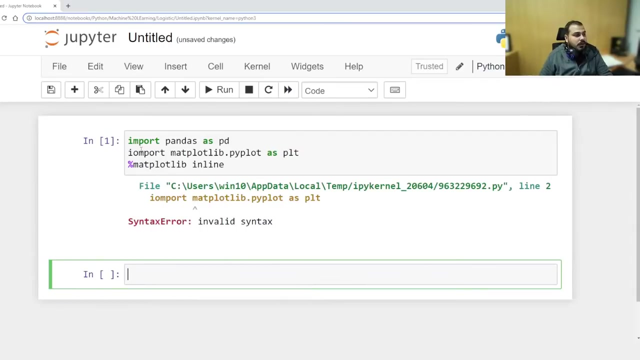 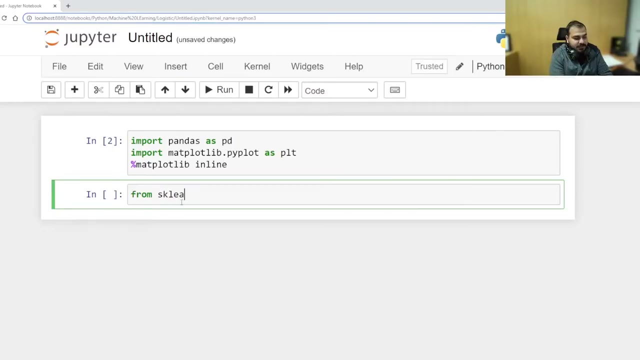 pd import matplotlibpyplot as plt. ok, import. so this basic things I have with me, so I will go ahead and take any dataset that I want from sklearndatasets import. let's say that I am going to take load iris dataset. 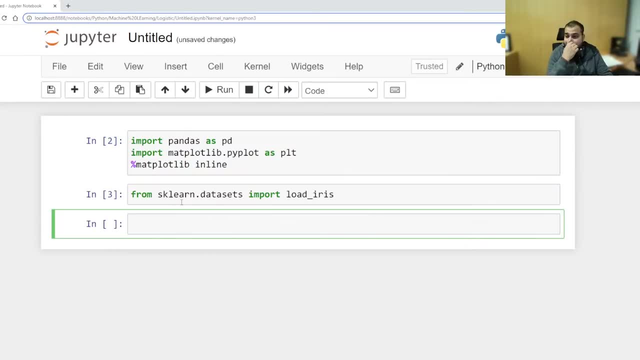 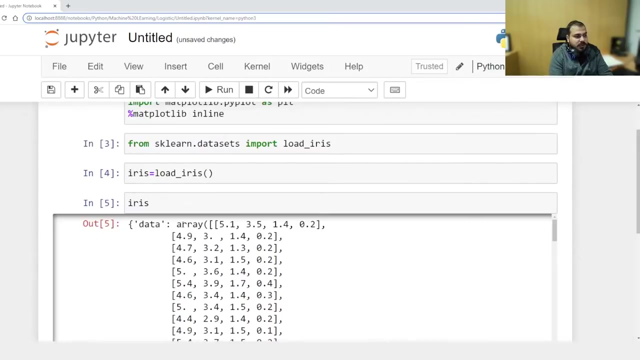 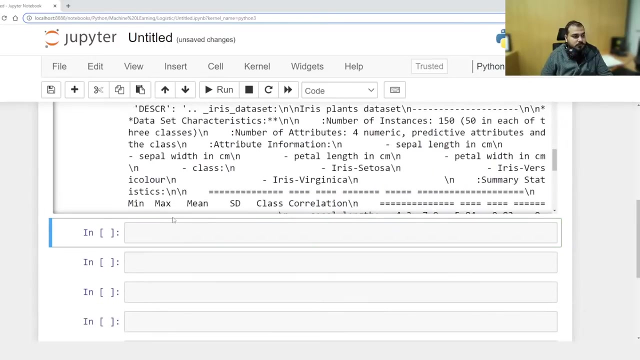 iris dataset. so everybody go ahead and write it down, Ok, and then I am going to upload the iris dataset. so I am going to write: load: iris. this is my iris dataset. then the next step: once you get your iris dataset, you will need: 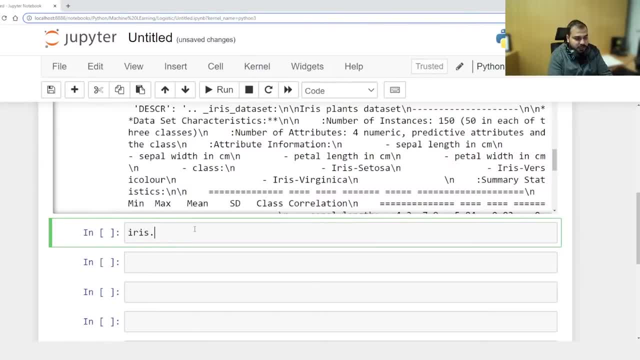 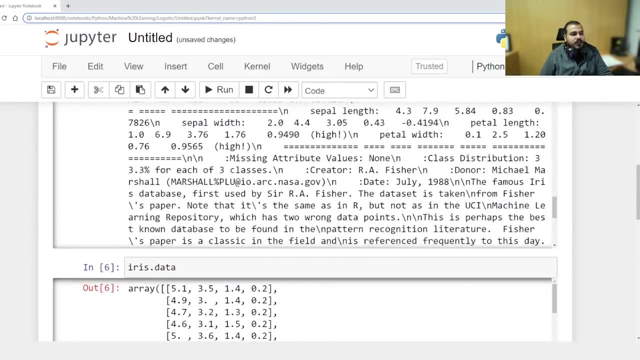 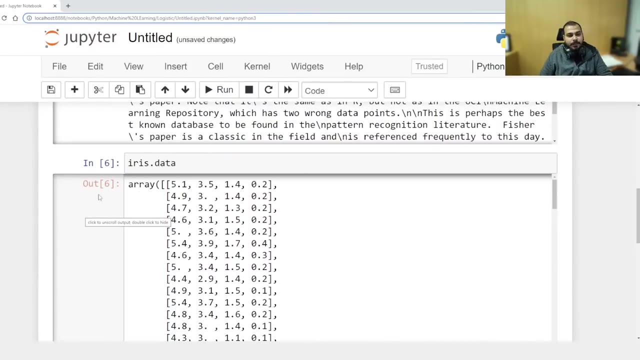 to import. ok, so this is my irisdata. ok, these are all my features. the four features will be there over here. these four features are: petal length, Petal Width, Sepal Length and Sepal Width. ok, this is my independent features. ok, then, if I really want to apply. 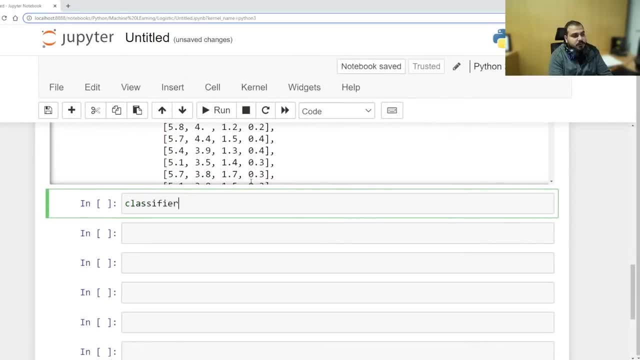 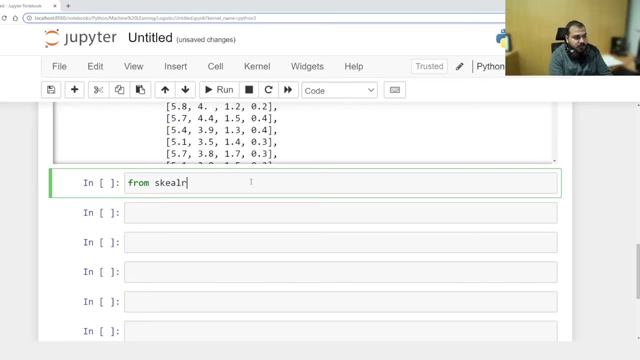 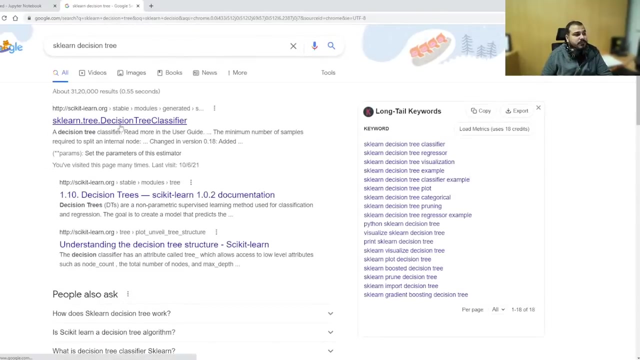 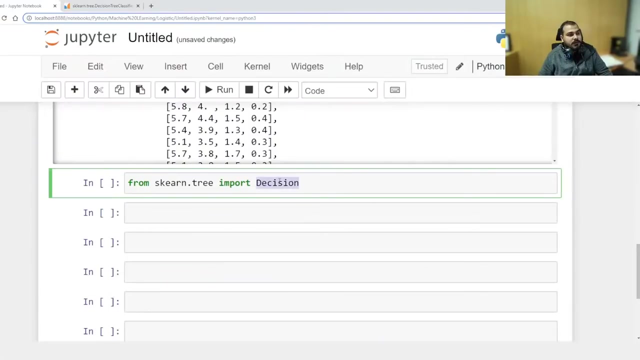 for classifier, for decision tree classifier, so I can first of all import it from sqn methods. ok, sklearntree import decision. let's see where is decision tree present in sklearn. hmm, decision tree classifier. the name is absolutely fine, but i was not getting over here, so 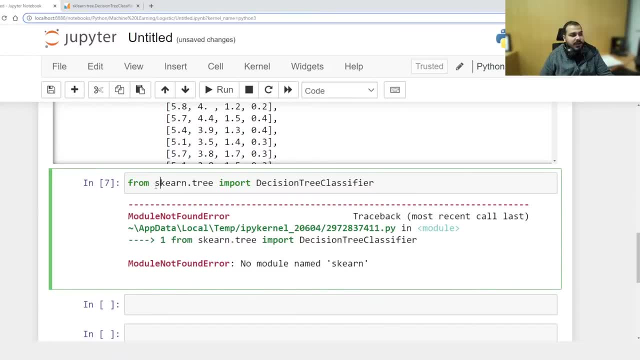 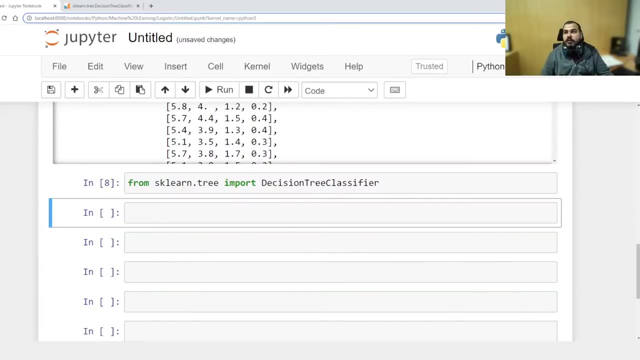 this is got no module. sklearn, okay, sklearn, sklearn, okay. so here you have classifier. right now I'm just going to over fit the data, then I'll probably show you how you can go ahead with pruning. so by default, what are the parameters over here? if you probably go and see in in the 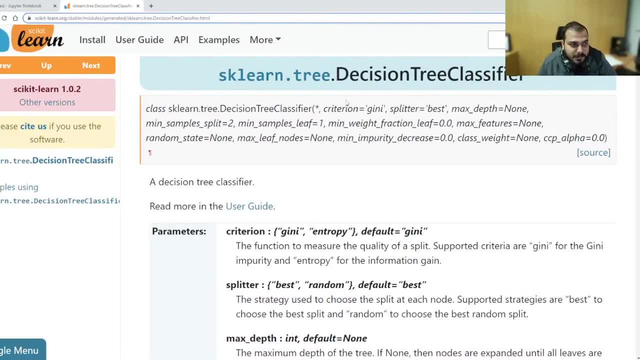 classifier over here you have criterion, see this. the first parameter parameter is criterion. by default it is guinea. okay, then you have splitter. splitter basically means how you are going to split, and there also you have two types: best and random. you can then randomly select the features and do it. okay, you should. 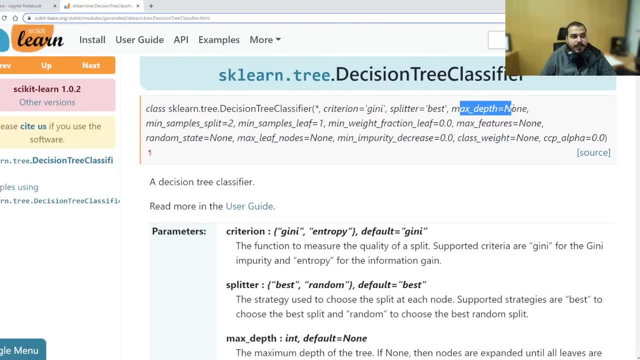 always go with best. max depth is a hyper parameter- minimum sample. if is a hyper parameter, max features- how many number of features we are going to take in order to fix that? how many number of features we are going to take in order to fix that? that is also an hyperparameter. so all these things are hyperparameter, okay, so i will just. 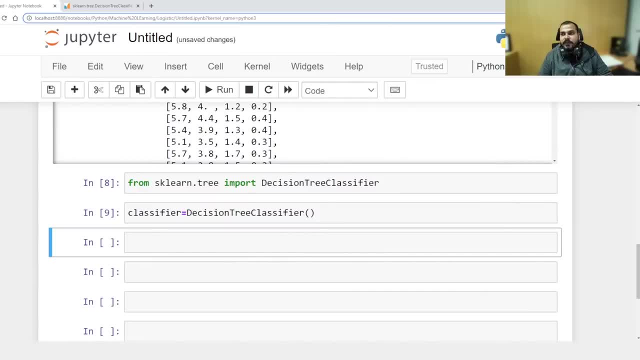 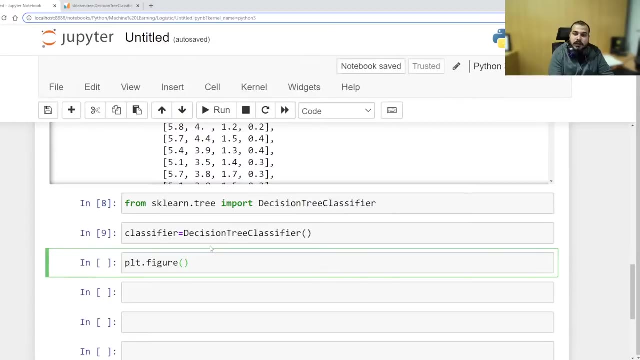 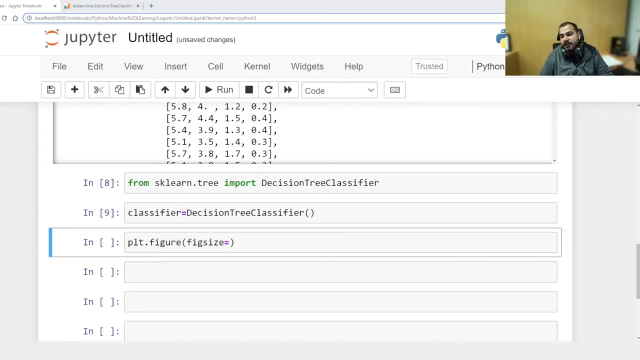 by default executed whatever is giving me in decision tree, and the next thing that i'm actually going to do is create a decision tree. okay, so for this i will be using plot dot fig size, plot dot figure inside figure. i have this fix size, okay, and i will probably show in some better figure size so that everybody will be able to. 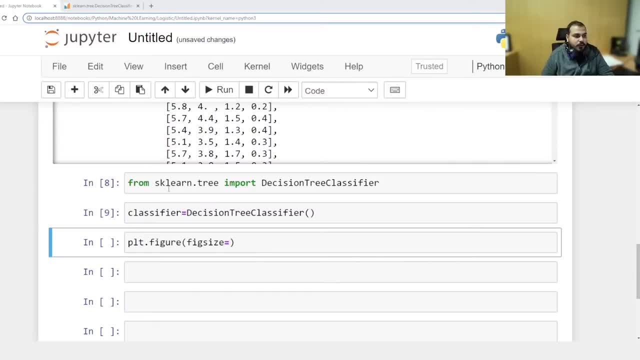 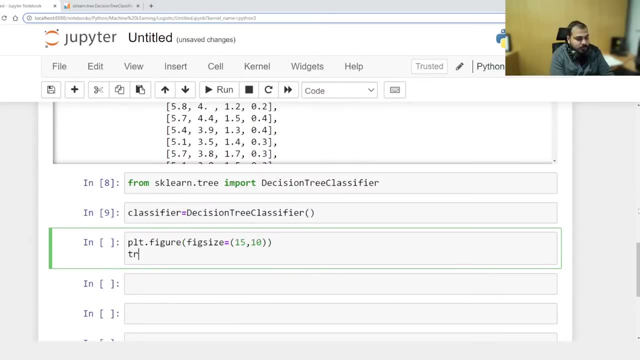 see it okay. so here let me say that i'm going to take an area of 15, 10, 15 comma 10, and then probably i'm going to say tree dot, plot, and here i'm going to say it's place, a classifier, and it should be filled, the coloring should be filled with this. 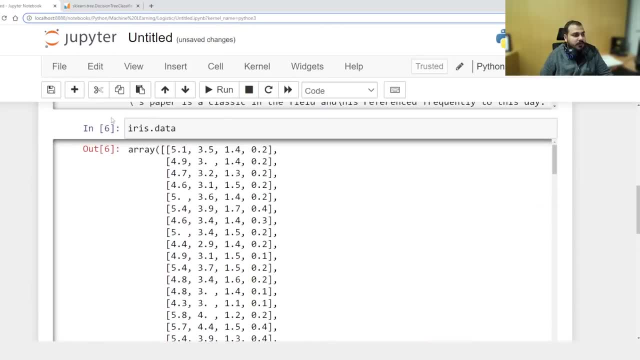 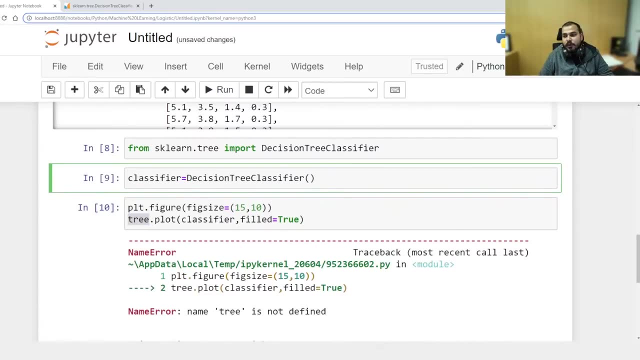 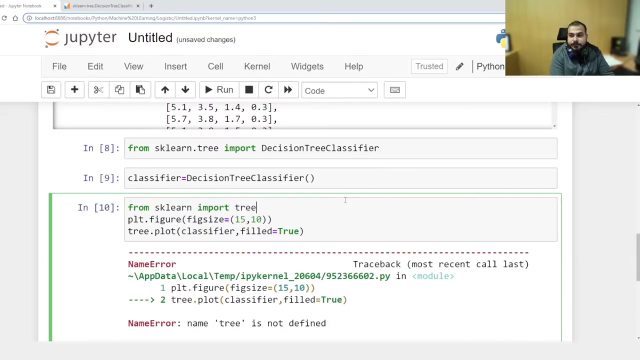 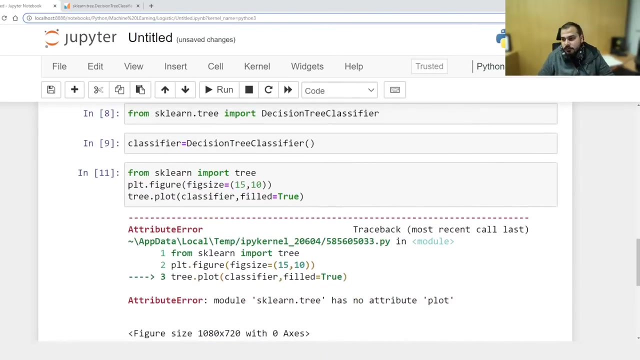 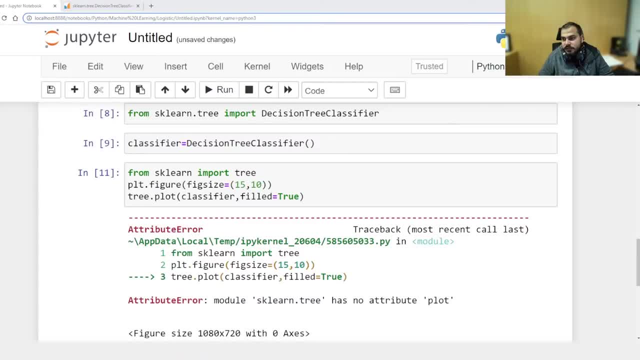 let me just see the documentation guys. let me just see the documentation guys. we are seeing the sk learn documentation. just a second: we are seeing the sk learn documentation. So this plot function is like plot underscore tree, just a second dot tab plot underscore. 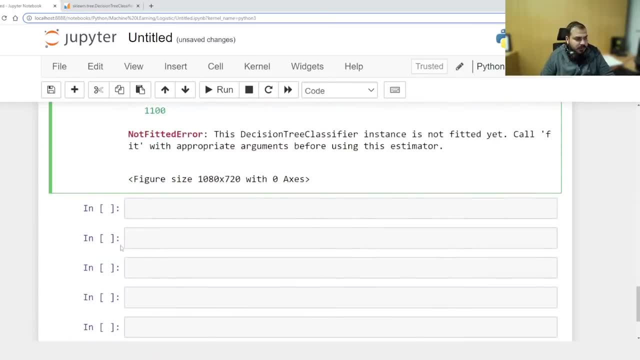 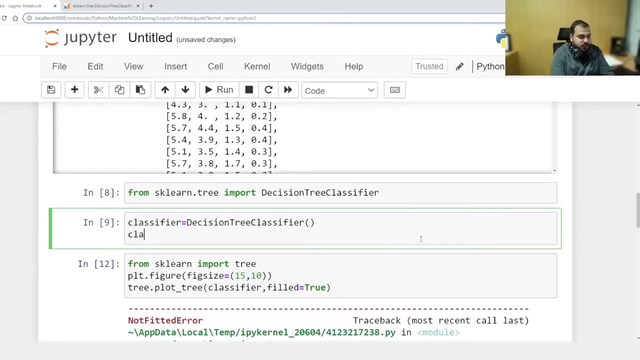 tree. now what is the error we are getting? ok, not fitted yet, sorry. so I am going to say: classifier dot, fit on data. what data? iris dot data. and then I am going to fit with iris dot target. so once this is done, I think now it will get executed. so this: 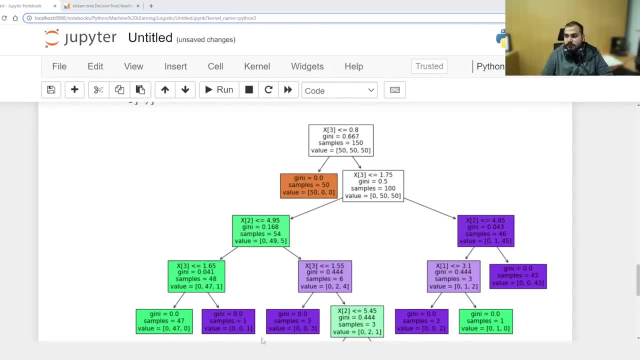 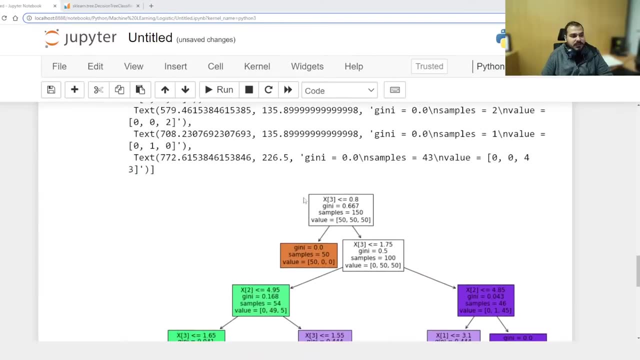 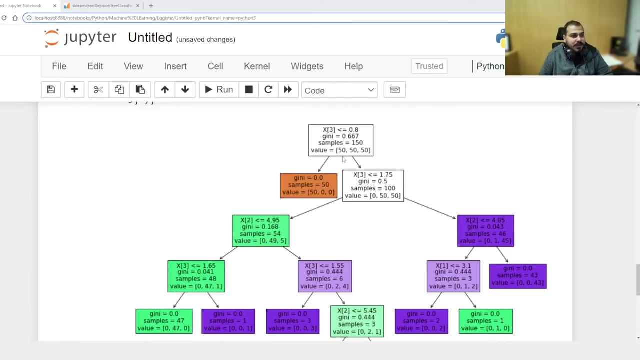 is how your graph will look like guys. ok, So here you can see, this is how your graph looks like. now, if I show you the graph over here, see, you can see some amazing things over here. three outputs are actually there. 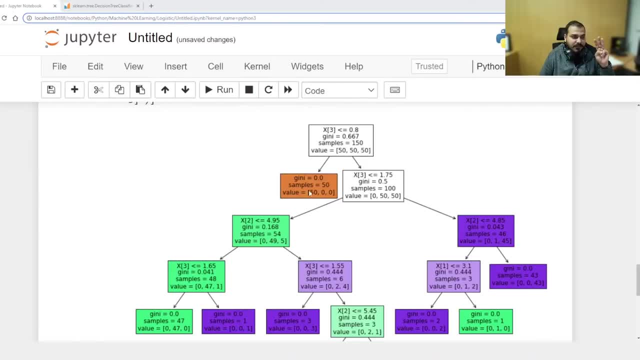 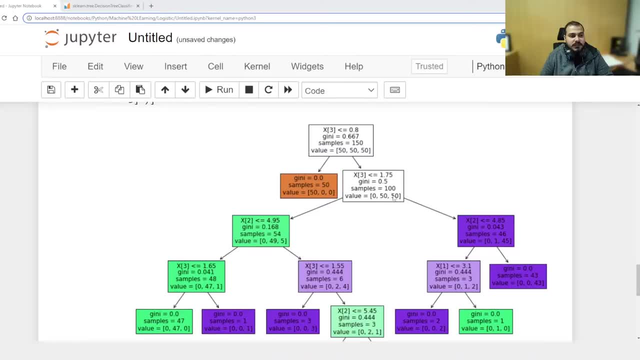 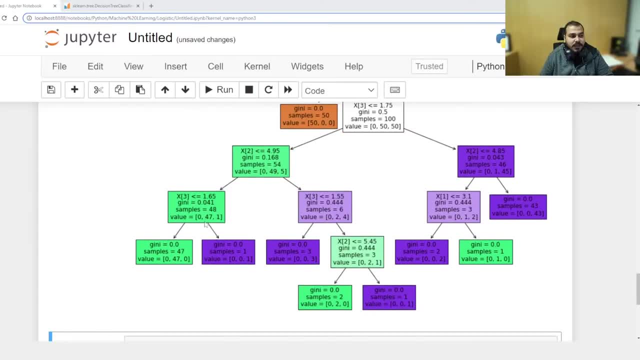 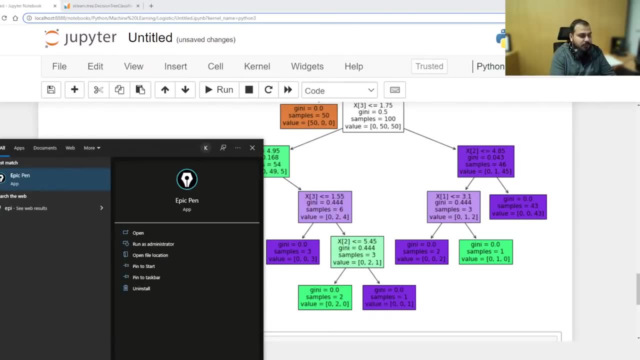 over here. ok, so here you have 49-5,. here you have 47-1,. do we require this split? anybody tell me from here: do we require any more split? just try to think. this is after post. 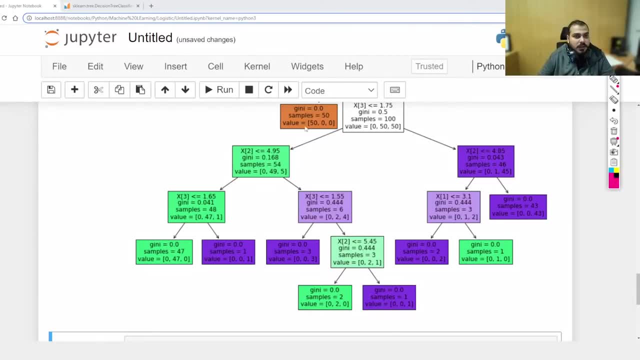 pruning. I want to find out whether more splits are required or not now in this particular case. you see this: after this, do you require any split? you did not require right. here you are basically getting forty seven and one right. i guess after this also, you require no split. 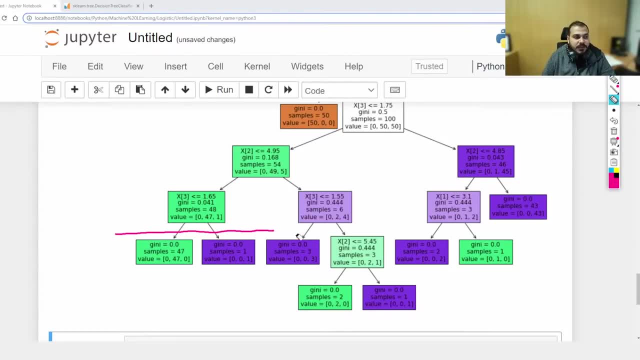 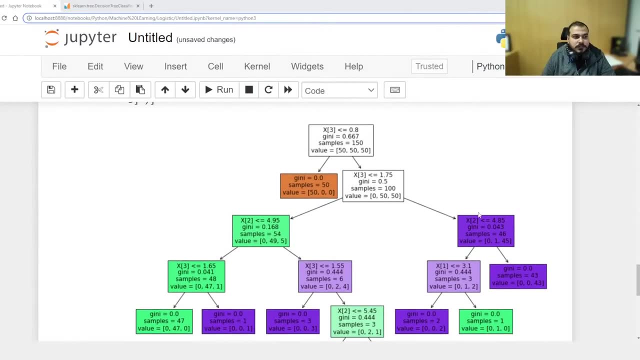 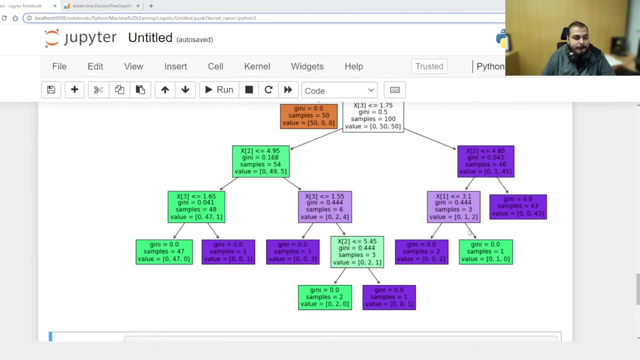 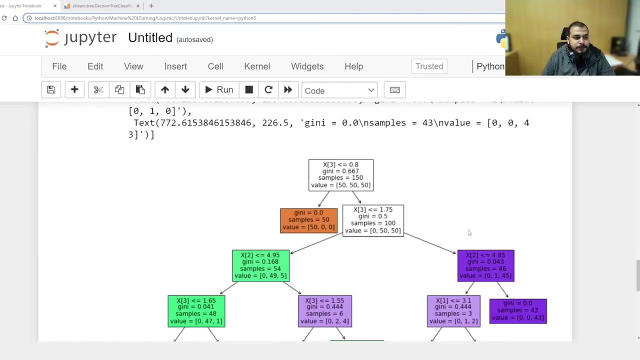 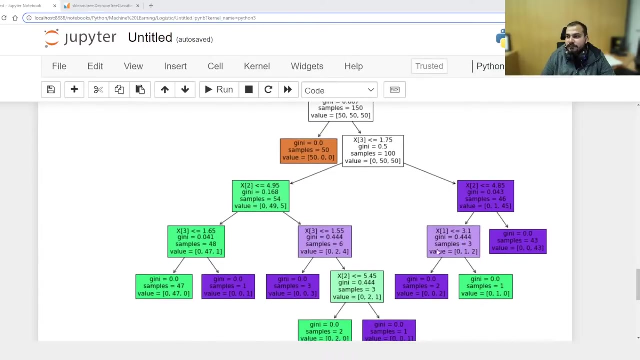 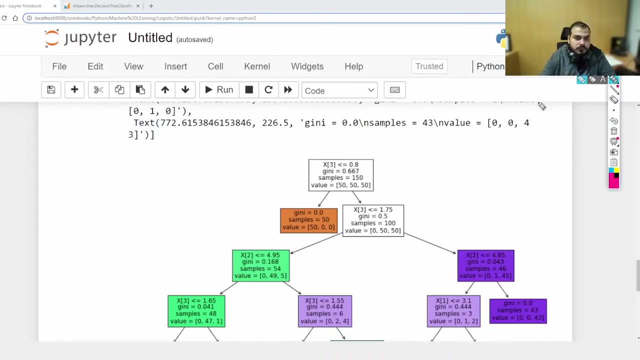 right, so understand this. so this is basically post pruning, so you can then decide your level and probably do it. any value is more than point five. okay, this side, this is coming as point five greater than point five. it should not had. here it is point five. no, maximum point five can come. 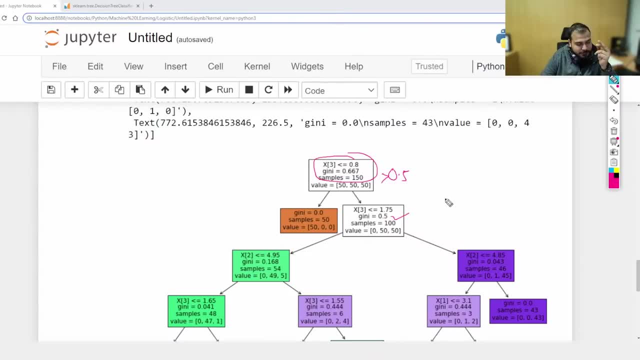 zero to point five. only you should come. i don't know why this is coming as point six, six, seven. i'll have a look on to this guys, but anywhere you see- other than that you're everywhere- you're getting less than point five. let's see that. 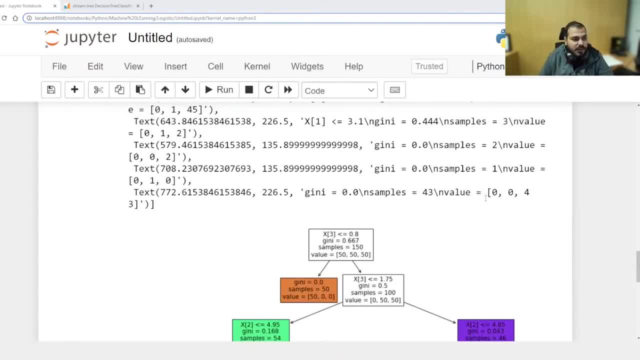 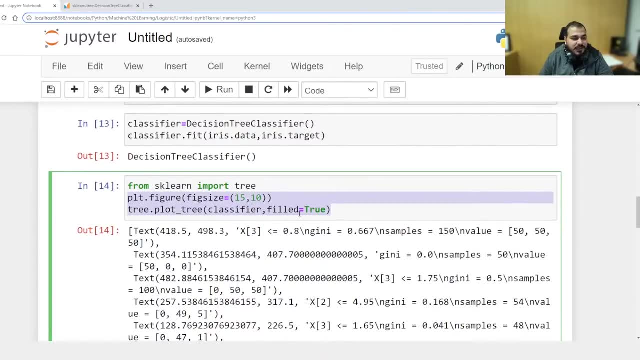 okay, the plotting graph is very much easy. you use sklearn import tree. then you basically do this: get classified and filled is equal to true, and you can just do this. i'll give the code. anyhow, i'll upload it in the next video and i'll see you in the next video. bye, bye. 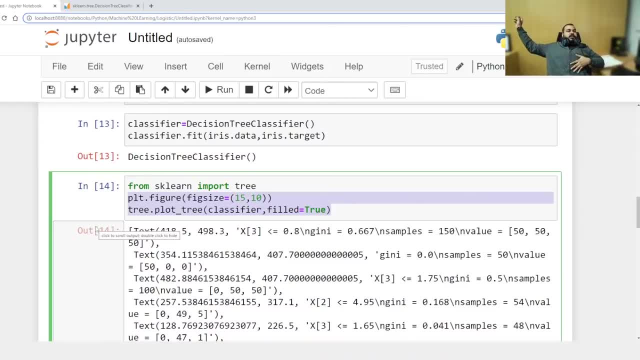 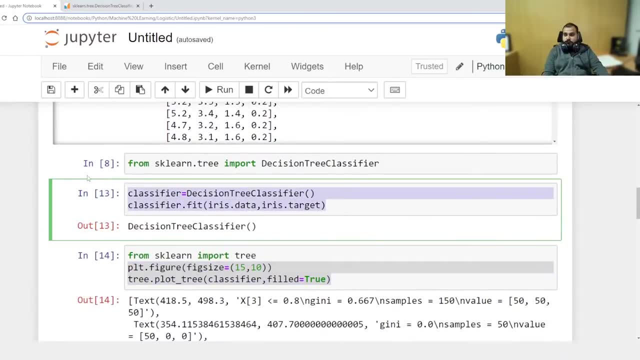 in the community session. please make sure that you join the community session over there. okay, fit queries here. so i hope you enjoyed the session. ensemble learning is there. i feel lot of tiredness right now, so i'll take assemble learning tomorrow guys. okay, assemble ML techniques i'll do tomorrow. 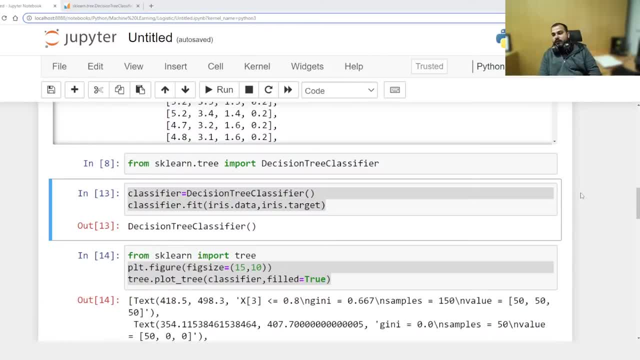